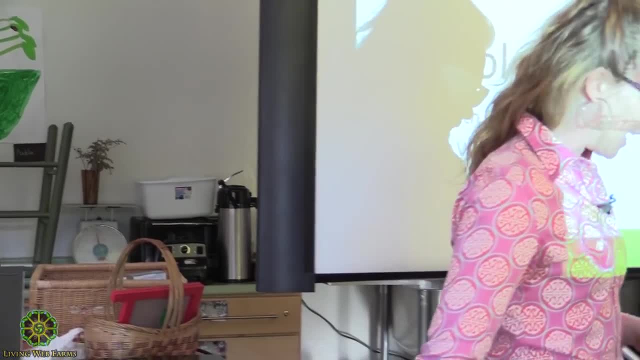 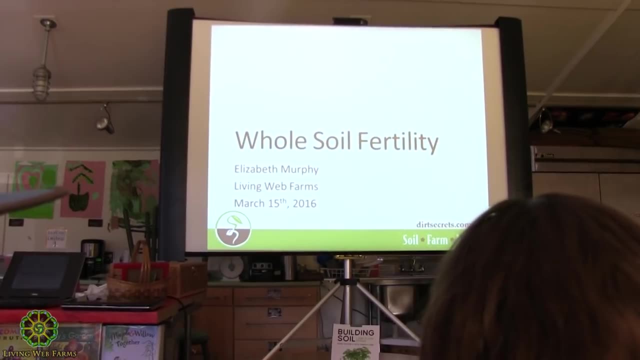 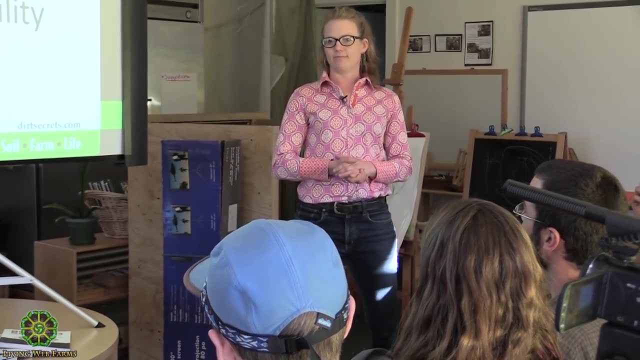 some of the things we're going to cover today, But first I kind of like getting an idea of who you are. So how many people here, Farmers? How many of you are growing things to sell? Okay, How many of you are growing vegetable? 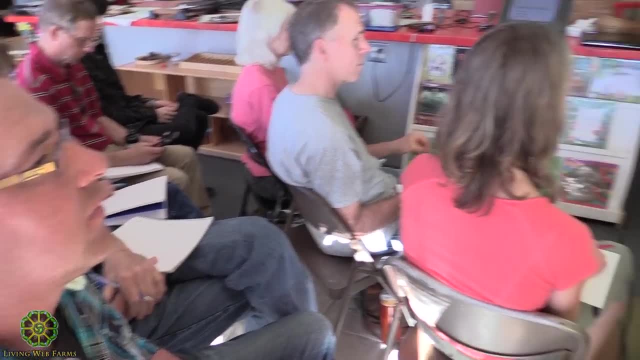 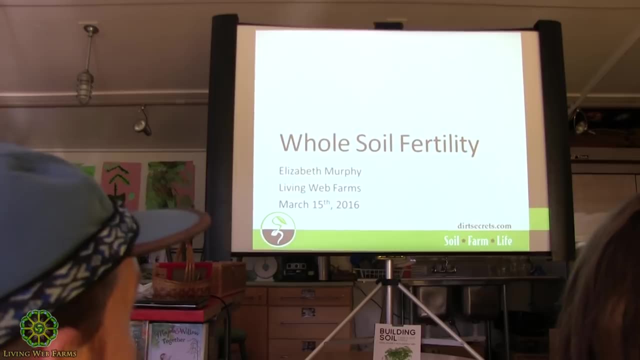 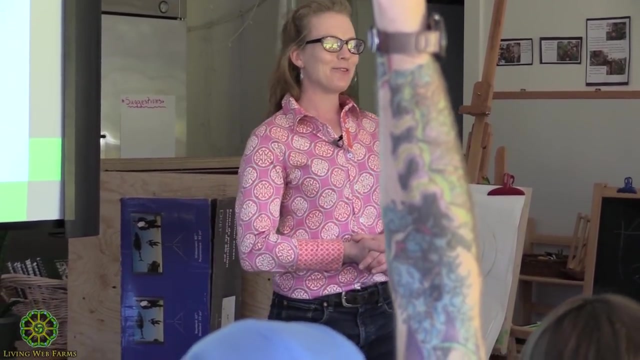 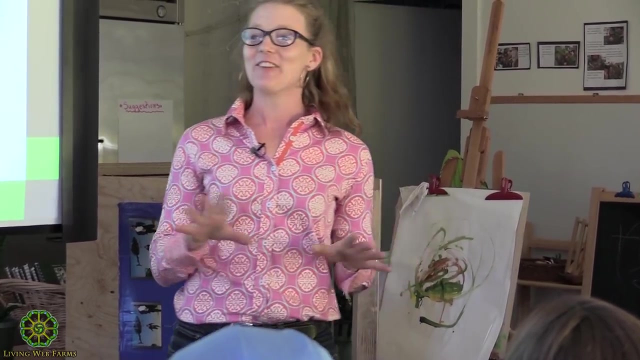 crops, Tree crops, Livestock. How many of you periodically submit soil tests? How many of you think you should submit soil tests? How many of you know what your soil test says and you get it All right? Okay, So I'm just kidding. Okay, So how many of you are soil scientists? 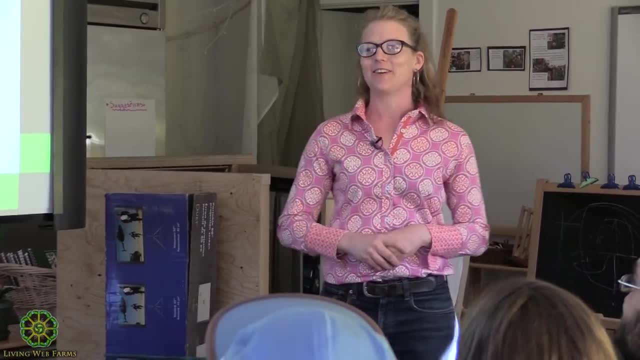 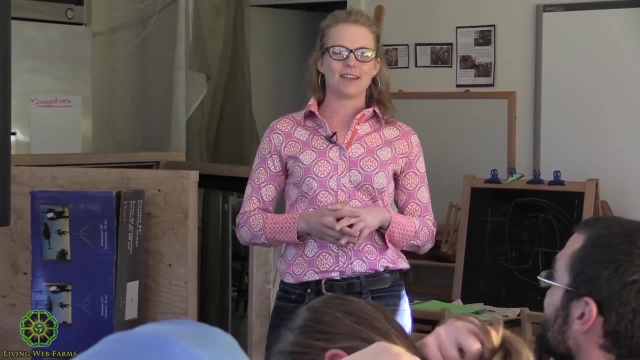 Raise your hand. So how many of your plants, Anyway? So I also want to know what you're interested, what you came to this class thinking you'd like to get out of it, So anyone. I'm going to write this up on the board so we can kind. 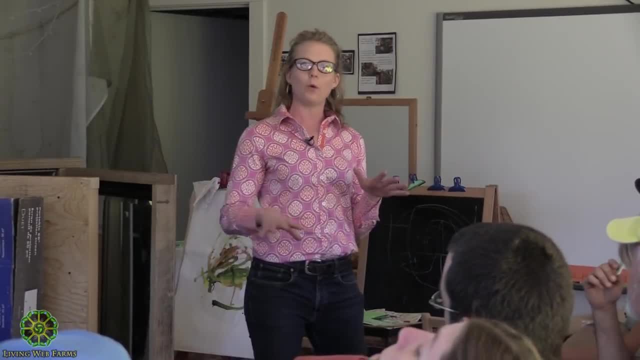 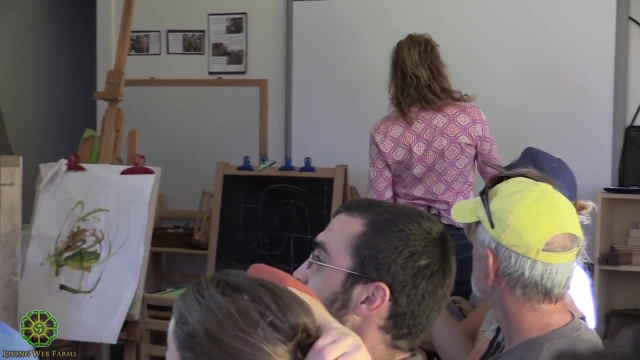 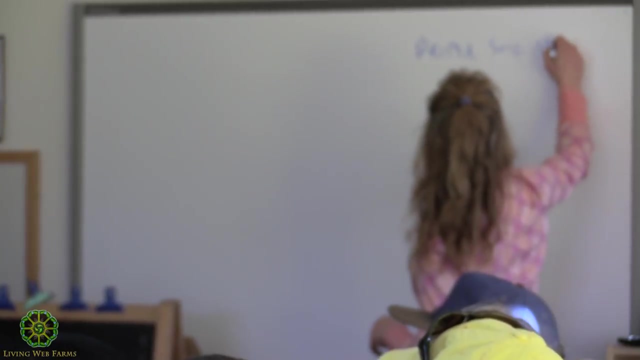 of think about it as we go through, But just go ahead and shout things out. What sort of things. when you heard you're coming to a whole soil fertility class, did you want to get out of it? No, proper soil management. anyone else intervals animals. oh, you thought this. 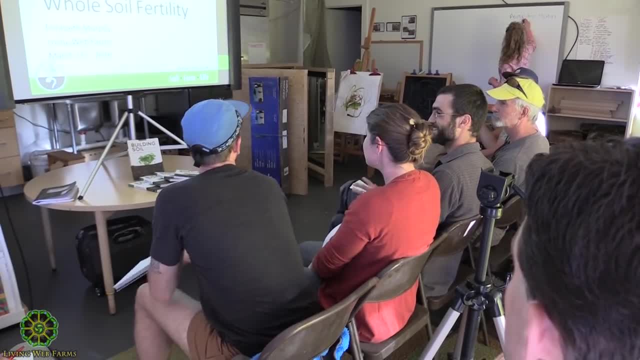 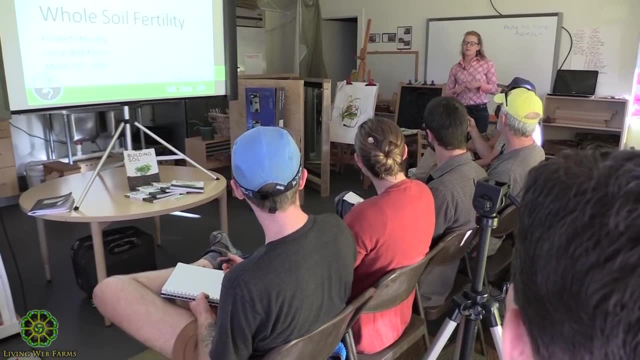 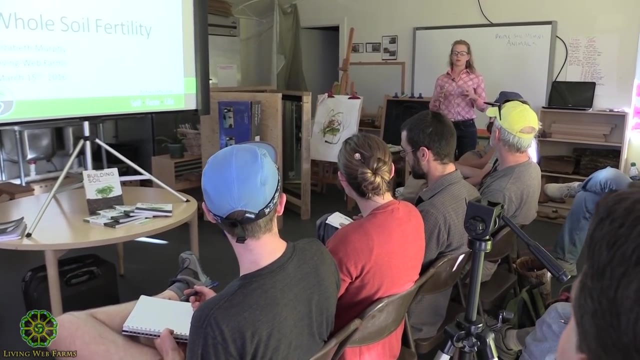 was the plant animal integration class. okay, animals- we're not going to talk too much about animals, but the fundamentals. actually, there's a lot of overlap between this class and the class I taught over the weekend, because the basics are all the same. we're talking about these whole ecosystems and an 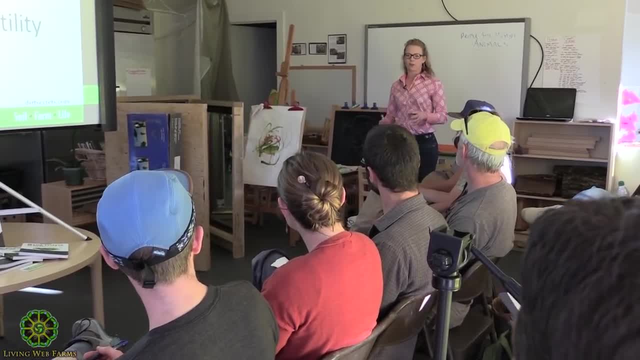 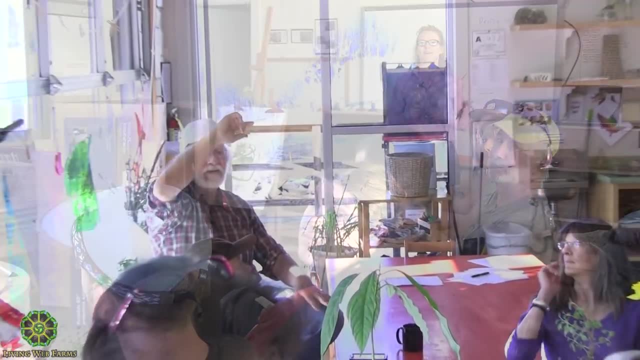 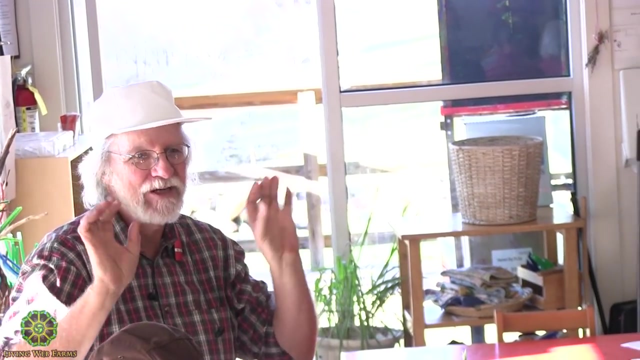 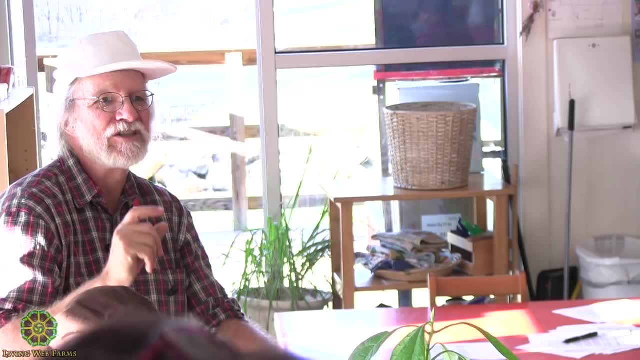 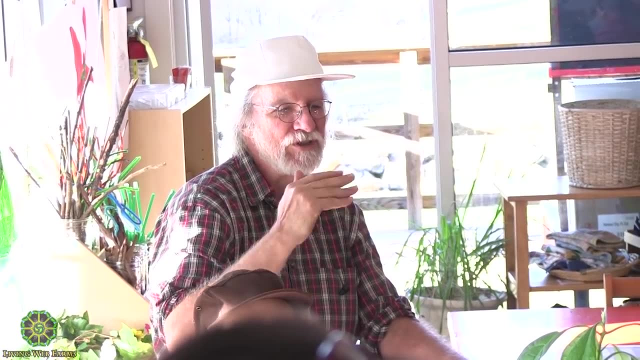 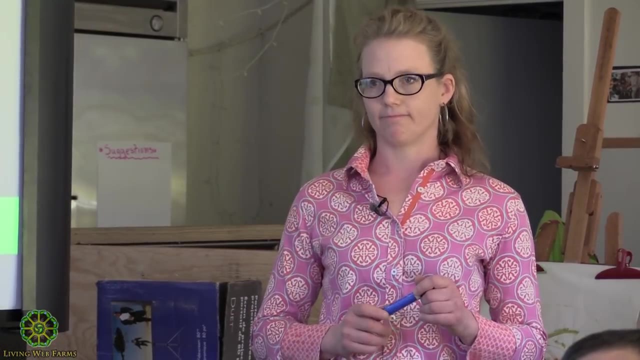 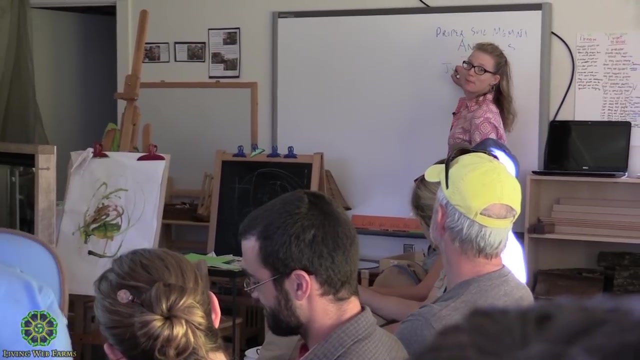 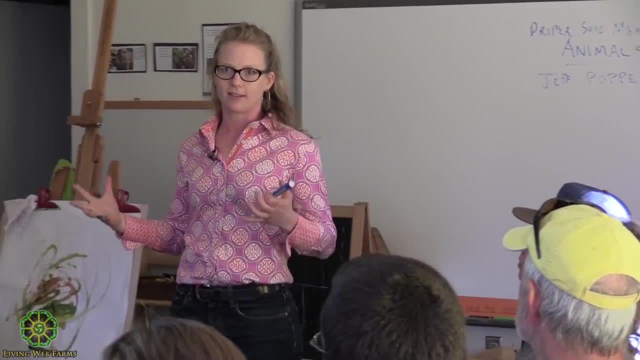 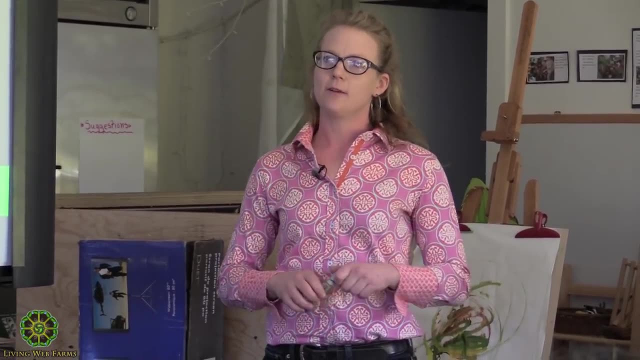 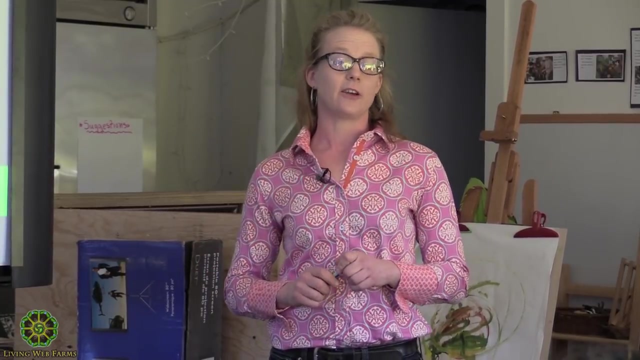 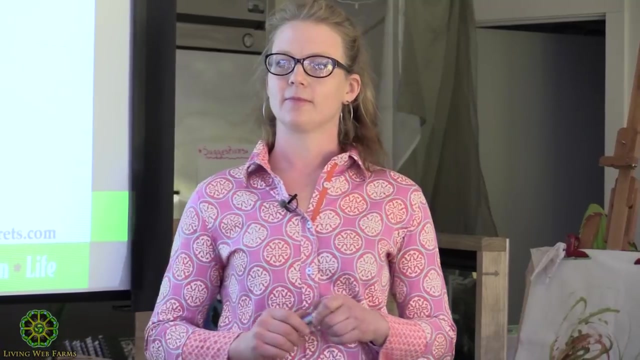 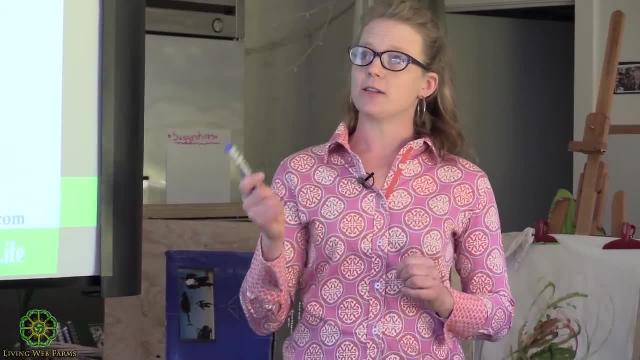 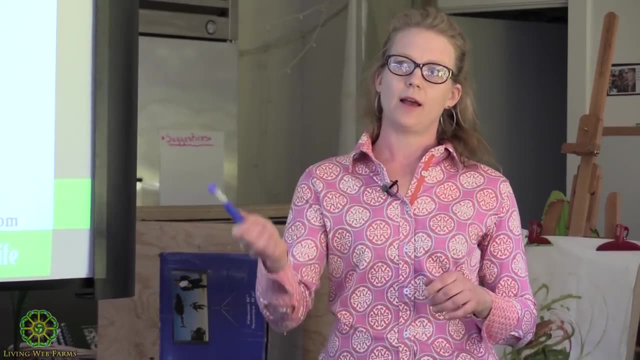 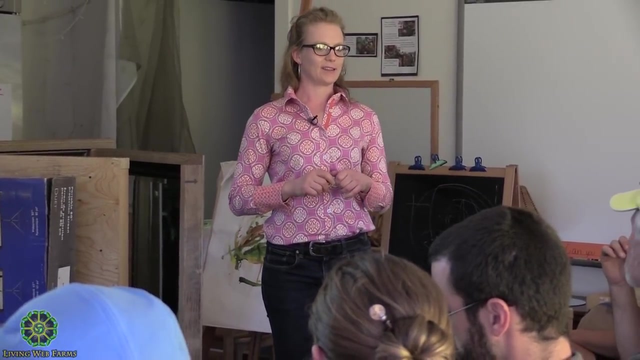 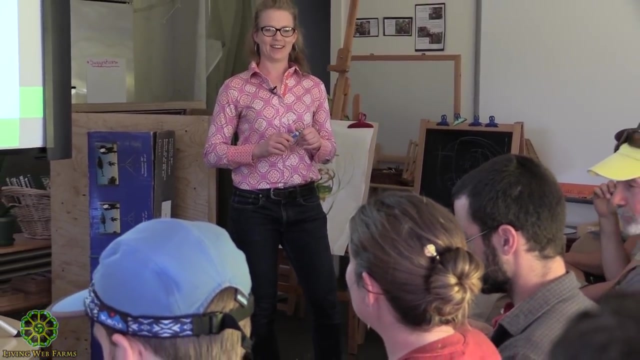 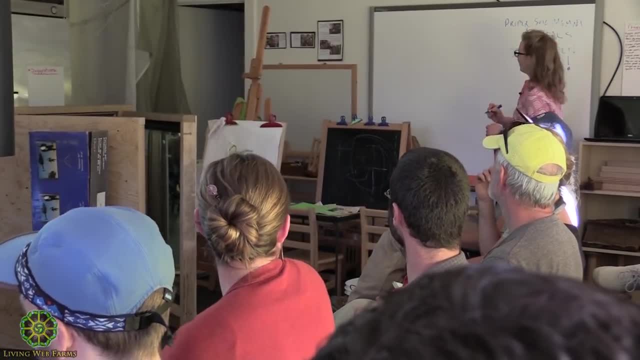 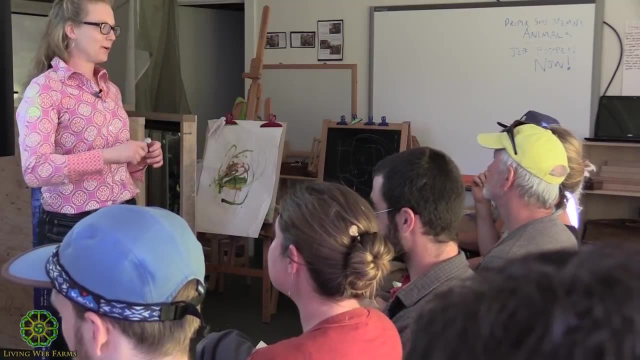 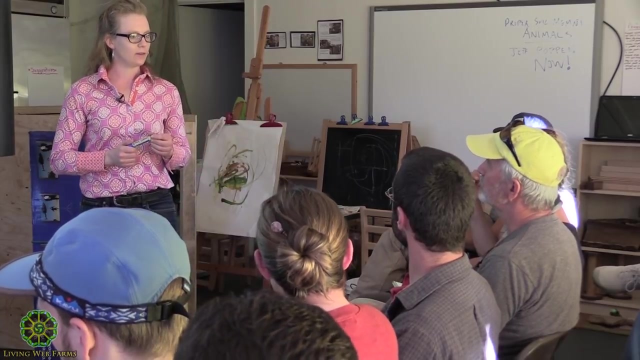 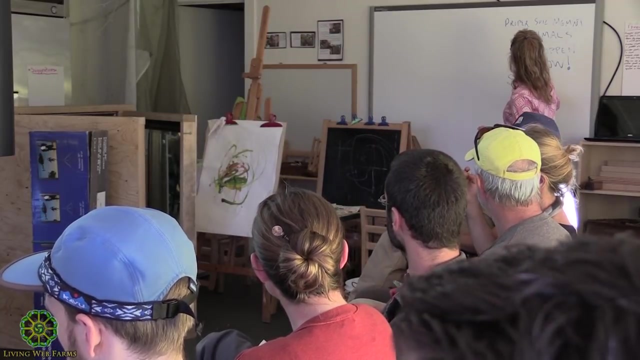 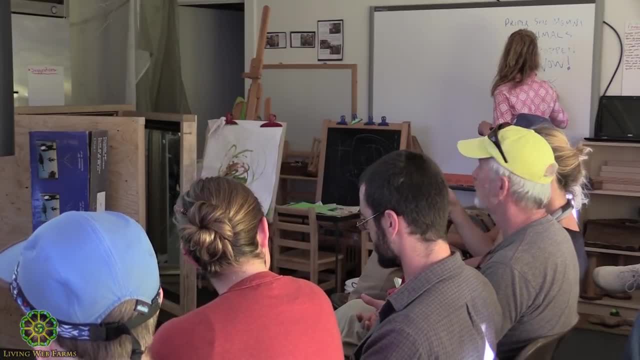 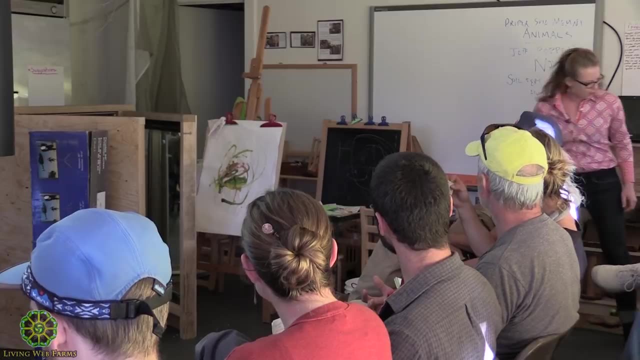 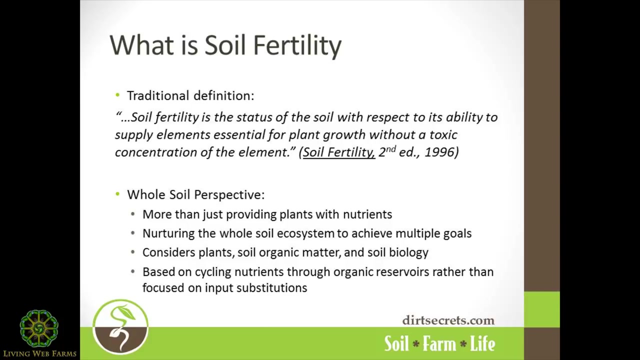 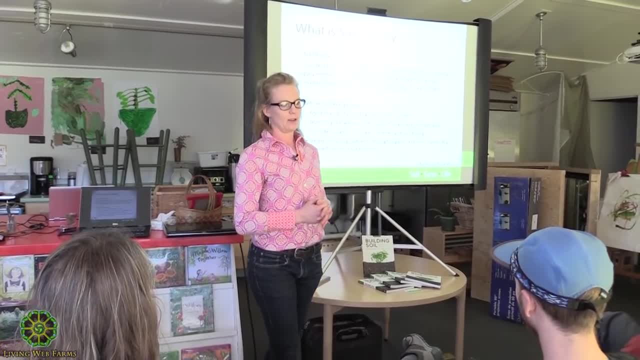 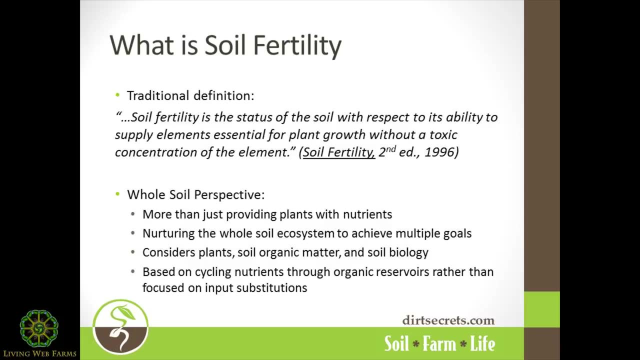 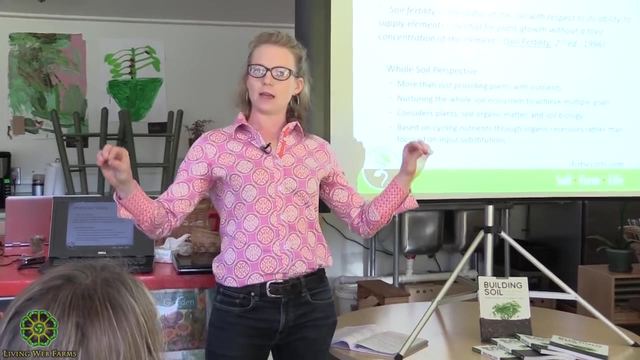 secondary nutrients for the purpose of plant growth. In my opinion, this is maybe not such a relevant definition for us, especially in these whole systems. When we look at soil fertility, we're looking at the whole soil perspective is looking at managing soils to provide a range of functions. 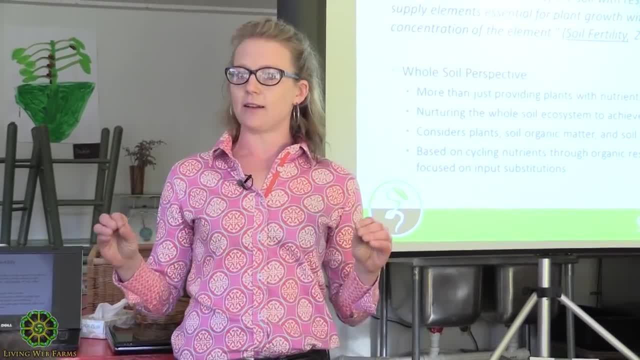 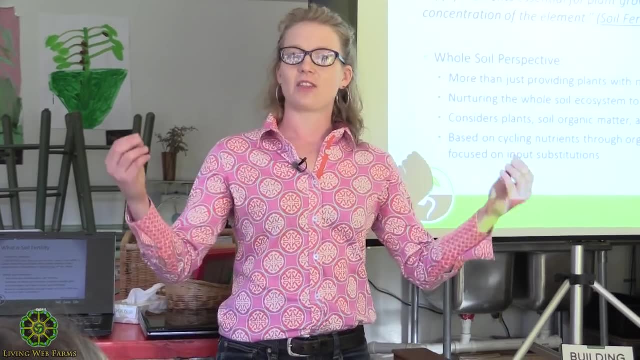 and managing soil fertility to provide a range of functions. It's not just about growing the plants, And I'm sure most of you are aware that we're dealing- and we're not going to talk about this too much- with the living, breathing, dying, throbbing, growing. 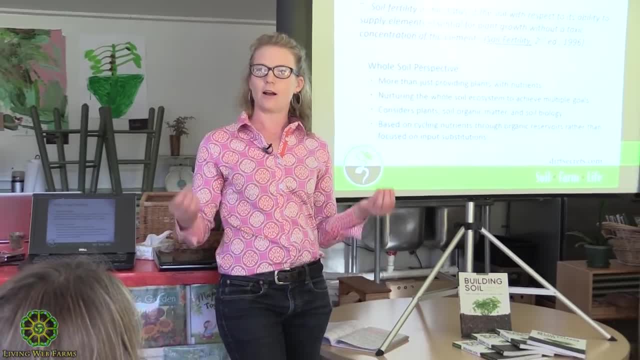 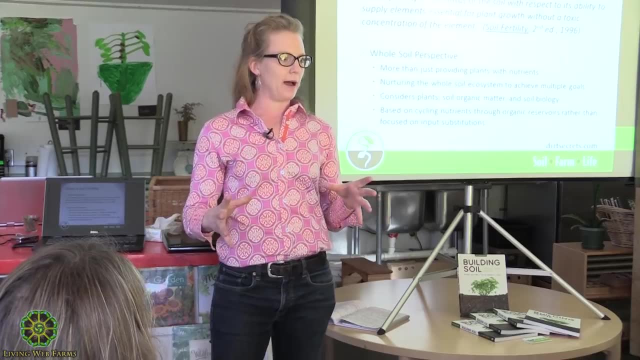 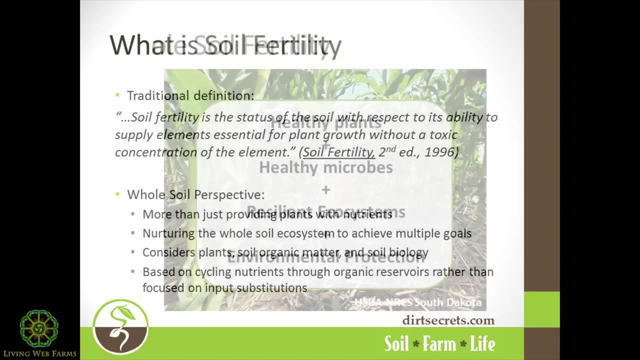 excreting system That's our soil. Our soil is alive, So we're looking at soils from a whole perspective of feeding the soil biology, nurturing the soil biology and having these complex interactions to achieve multiple goals. OK, so we want healthy plants and we want healthy microbes. 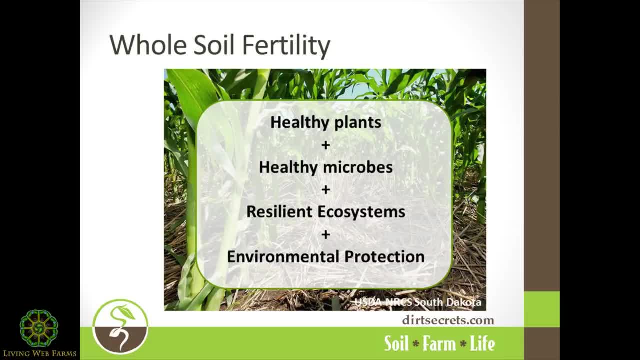 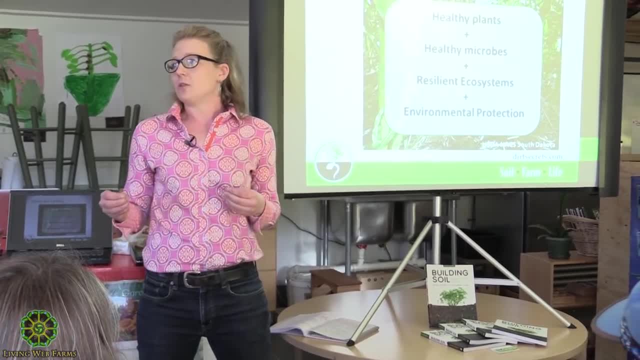 And through this we get a sweet, deep ecosystem functions. We get resilient ecosystems that are more resilient to pests and disease, that are more resilient to disturbance that if we do till them like crazy, if we do think that you have to have this deep till, 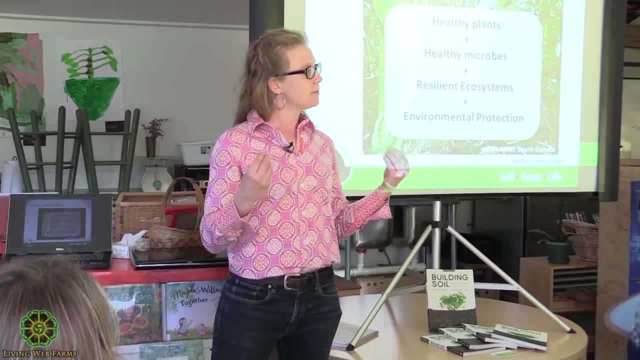 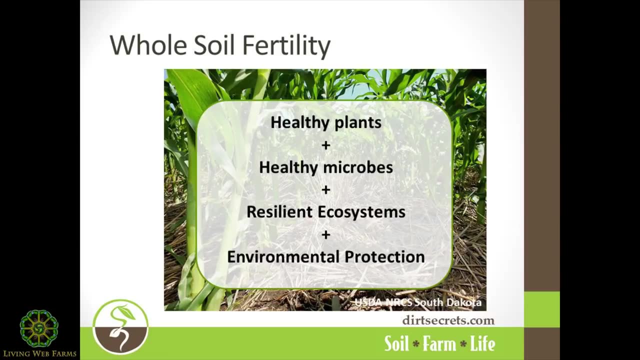 that Jeff Poppins is talking about. they're these amazingly healthy systems. They recover from that And they also provide an enormous amount of environmental protection, so preventing the degradation of water quality through loss of nutrients. degrading toxic compounds- Microbes can degrade. Some pretty nasty organochemical compounds. So these are the functions that our soils perform for us, And they're very important in agronomic systems, agronomic ecosystems, because they are what lead to higher yields, better tasting, more nutritious food. So these are the soil nutrient pools. OK, so soil nutrients exist in a range of pools, So we have the soil, Soil solution right in the center. Oh, the soil solution. That's where all the good nutrients are. That's where all the nutrients are that the plant can take up. 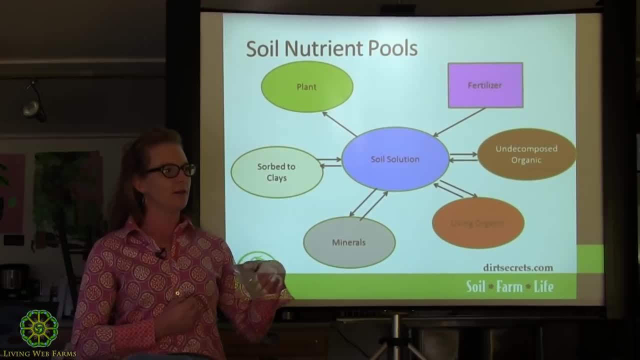 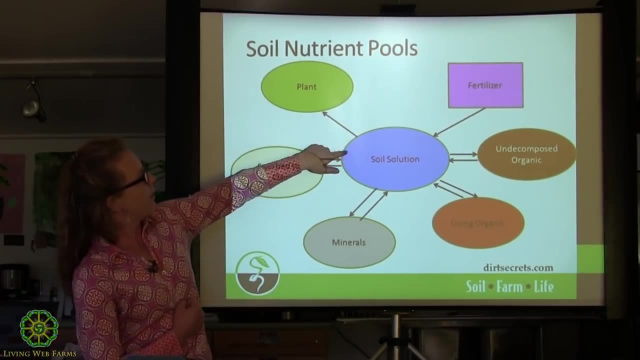 We have the plant. There's a lot of nutrients in the plant that, when it goes back to the soil, are recycled and decomposed. We have nutrients sorbed to clays that are exchanged with the soil solution. That's right. plants can only take up things. 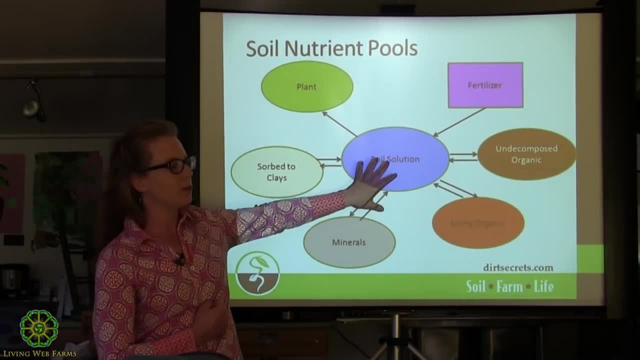 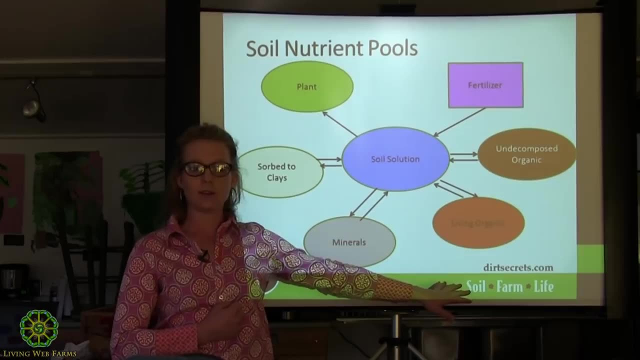 from the soil solution. We have minerals that are weathered into soil solution. We have living organic. We have organic materials that decompose into the soil solution. We have the organic material that decomposes into the soil solution. We have the live, living part of the soil that also needs nutrients. 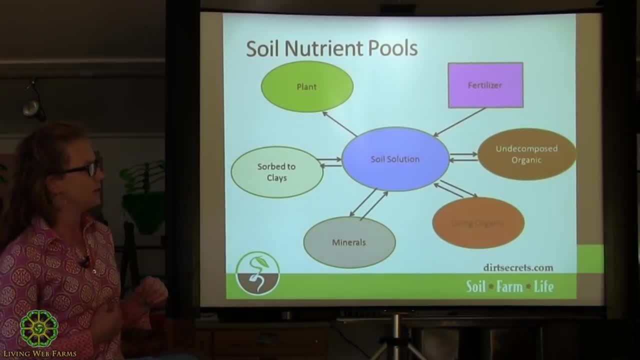 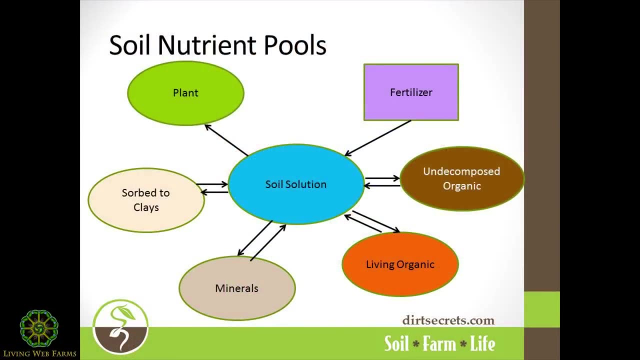 essential nutrients. We have the undecomposed organic part of the soil that decomposes via the biology to go into the soil solution. And we have the fertilizer that goes straight into the soil solution so that the plants can take it up. OK, so the traditional view of soil fertility. 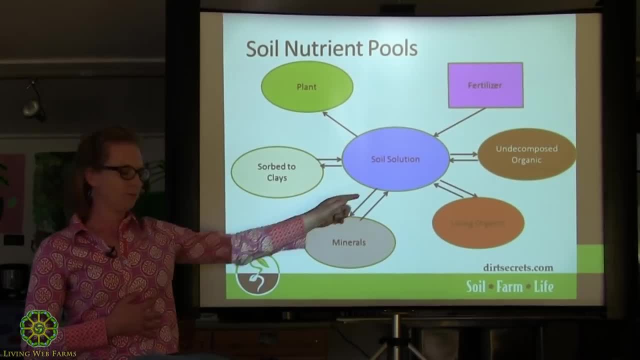 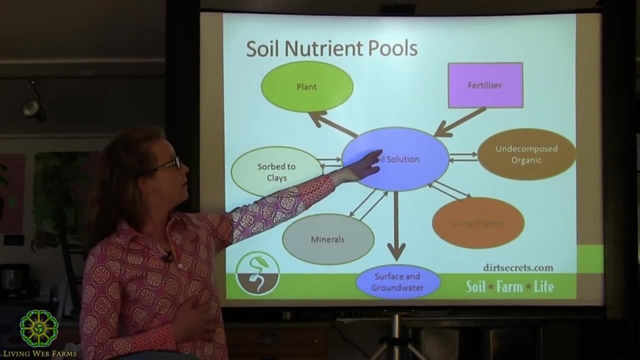 that we've been dealing with are these three pools, OK, so this: we're really concerned about the fertilizer. It's immediately soluble, taken up by the plants, And then anything left over. a lot of it is going to be leached out of the system. 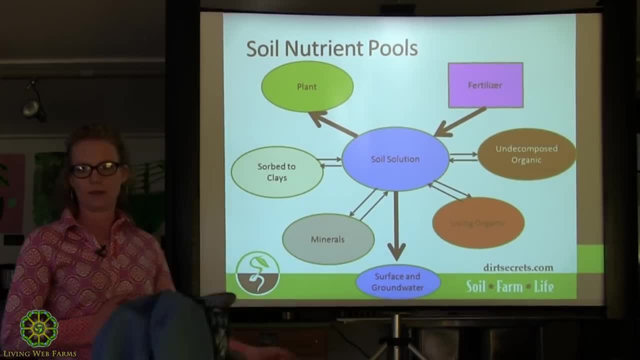 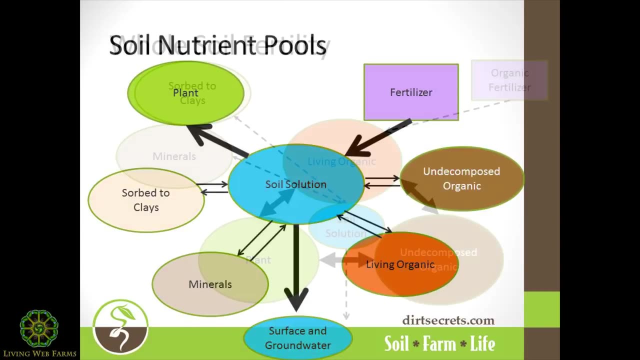 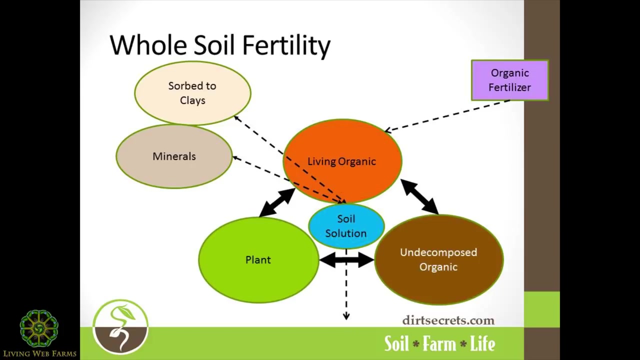 So these are the nutrient flows in our traditional system And, as I said, this is what we're measuring. But in a whole soil fertility perspective, we're really concerned about the nutrient flows and the nutrients that go into the soil solution. OK, so the nutrient flows and the nutrient cycling. 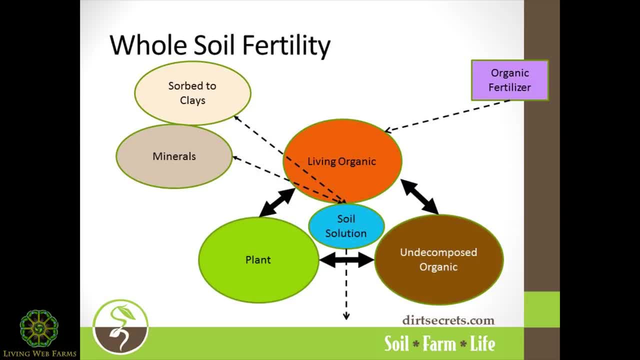 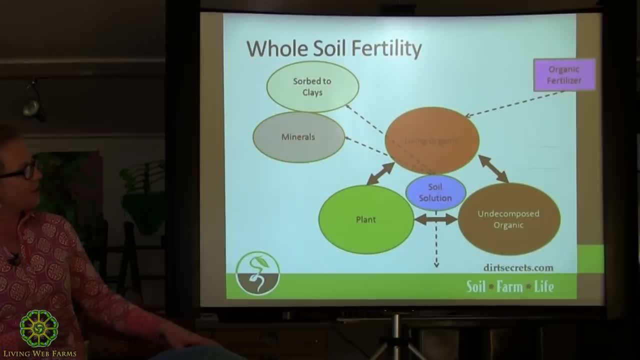 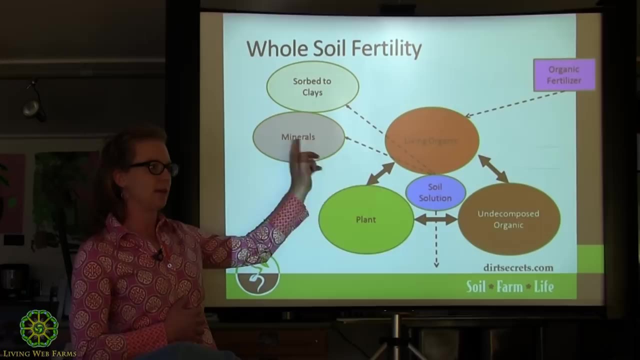 in these organic pools. OK, so the organic pools include the plant, include the living organic, the soil biology, include the undecomposed organic. There's a small amount lost to leaching. There's some exchange with minerals, And I say exchange because it is a chemical process that. 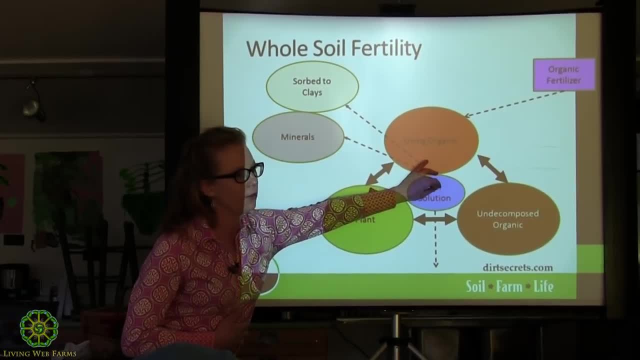 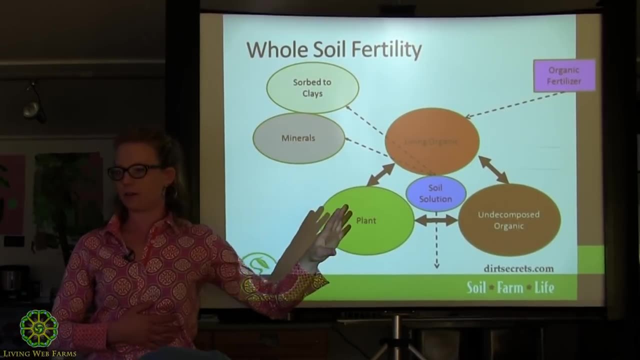 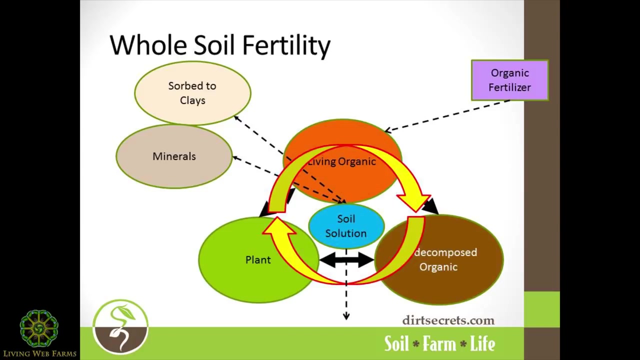 goes both ways, But these are actually largely biologically mediated through the living organic portion, And the soil solution is really just a medium for these transfers. So we're really focused on this nutrient cycling between the live, the plant and the organic material. 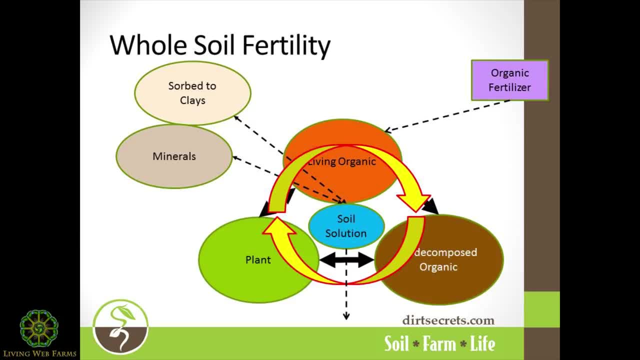 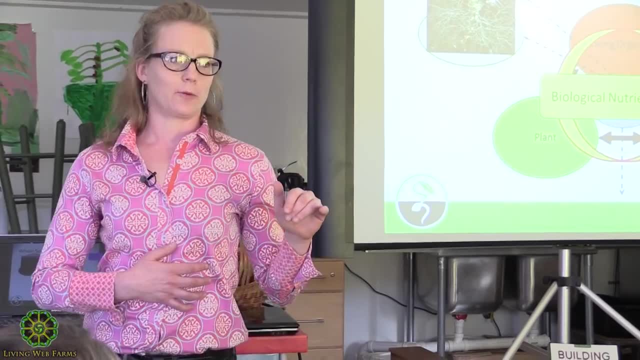 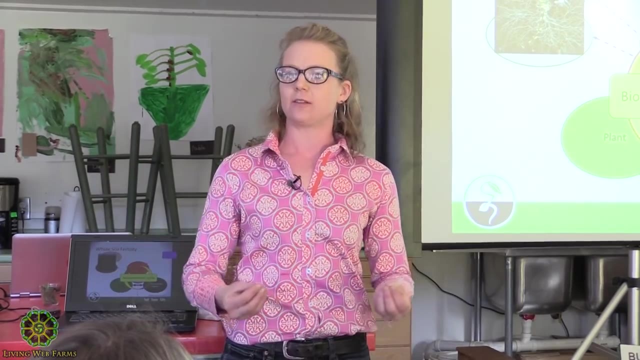 to retain the nutrients in our system, to make the most efficient use of the nutrients in our system, and to exploit- which is a weird word, but I used it to exploit- a whole range of ecosystem services that having this living ecosystem affords us. 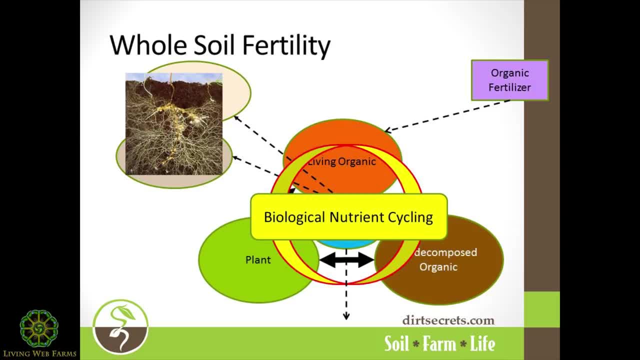 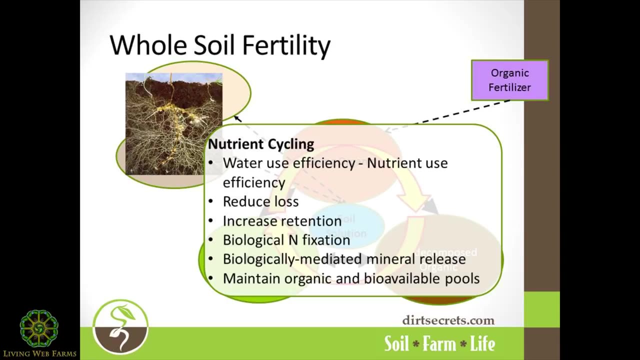 And, as I said, there's a lot of this, even what we think of as inorganic processes that are mediated by the biological system. So this leads to increased water use efficiency, nutrient use efficiency, So not just the amount of nutrients in water. 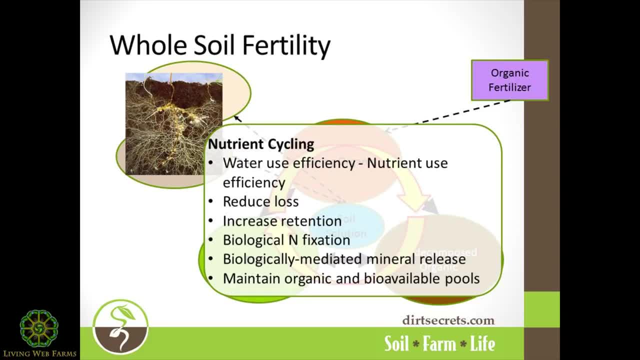 but the efficiency with which they're used. Very important concepts for us to realize when we talk about making sure our plants have the right nutrition: Reducing loss, increasing retention, focusing on biological nitrogen fixation and biologically mediated mineral release of nutrients in order to maintain diverse pools. 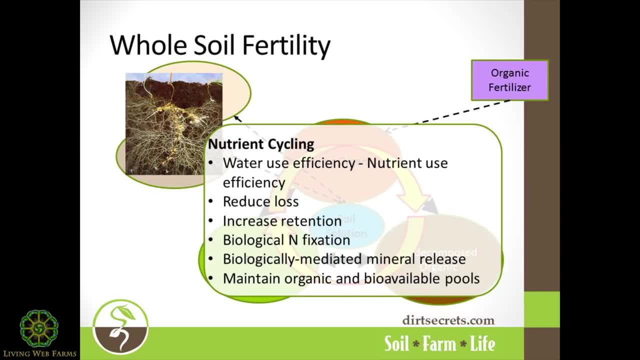 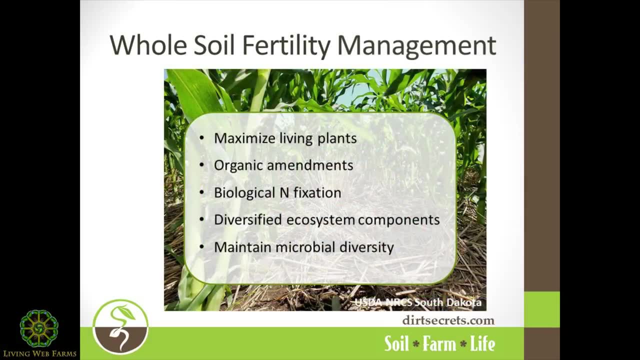 of bioavailable nutrients, but not nutrients that are just stuck in the soil solution to be lost. So how do we do that? We maximize the living plants. Our biological system needs living plants. We want to minimize our bare fallows, The more roots we have. 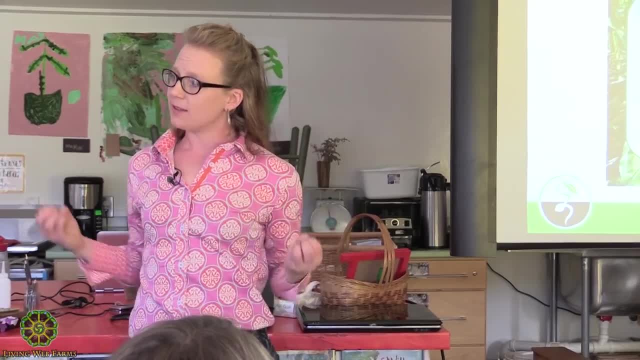 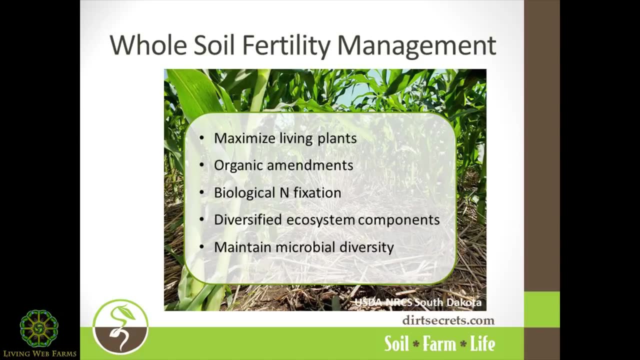 the more rhizosphere interactions we have, the more that photosynthetic carbon is getting pumped into our system, the better off we are by maximizing these living plants. We want to focus on organic amendments instead of water soluble chemical fertilizers. But even if we are going to use fertilizers, 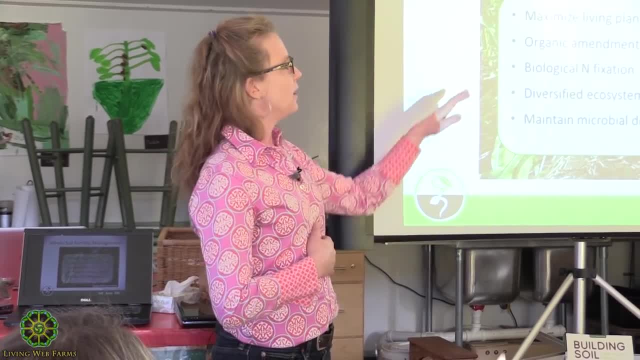 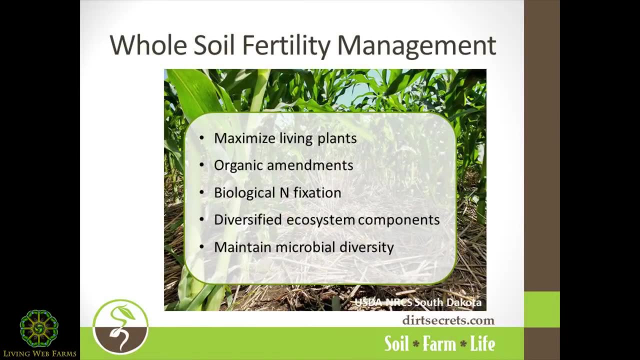 organic fertilizers do offer some benefits of most of them Having some organic matter to feed the living soil. We want to focus on biological infixation instead of importing it from outside the system, And biologically mediated phosphorus, potassium, calcium release from our nutrient rich soils. 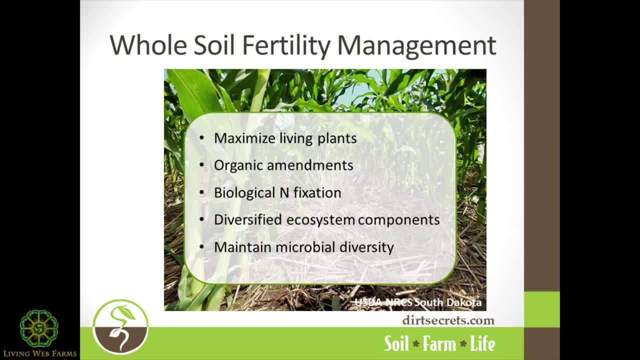 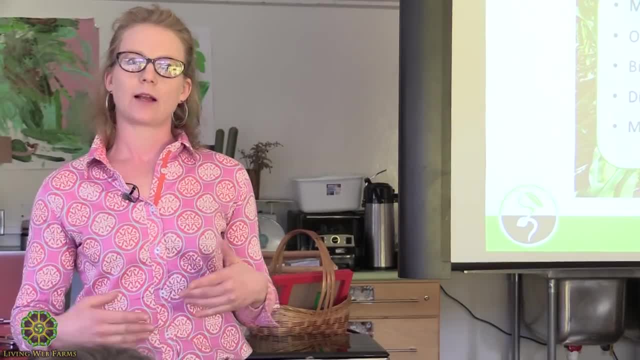 We want to focus on diversified ecosystem components and all the benefits that you get from diverse systems, And we want to maintain microbial diversity, And this is where a lot of our compost, compost teas- come in. This is where the reason we don't really ever. want to use herbicides or pesticides or salt, heavy fertilizers or manures. if we can help it because we want to maximize our microbial diversity, And if we do a practice that knocks it back, like tillage, we have a healthy enough system that it can recover. 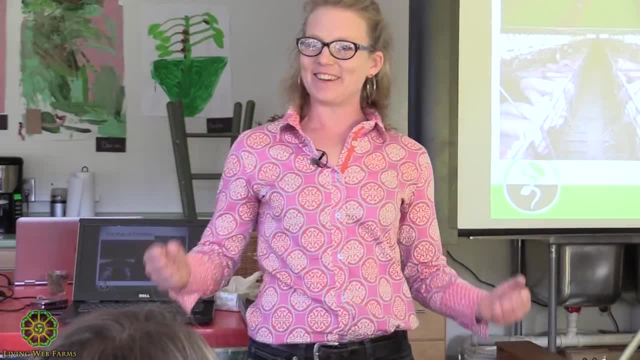 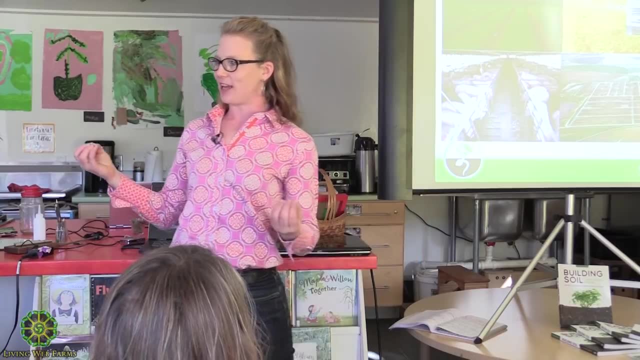 The rise of fertilizers. So what's the story with fertilizers? So there's an incredible amount of nitrogen all around us. 80% of the air is nitrogen, But it's really really really, really tightly bound to each other. And it takes an enormous amount of energy to break it down. One way it gets broken down to be deposited in the earth is through a lightning strike. That's the amount of energy it takes And when we did manage to fix nitrogen through the Haber-Bosch process in 1909,. we also created a lot of munitions, because it takes that much energy that we create these explosive materials. So after World War II in 1945, we had a lot of extra munitions And we also had an agricultural industry that was becoming more industrialized. 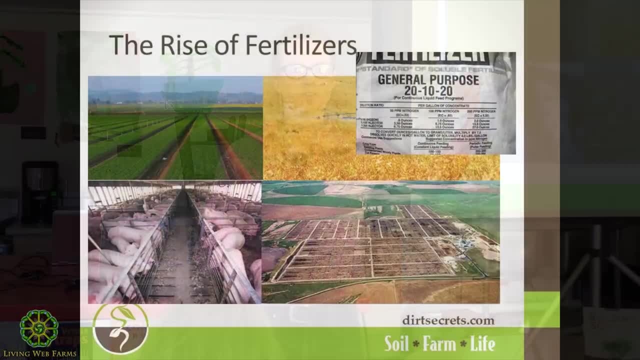 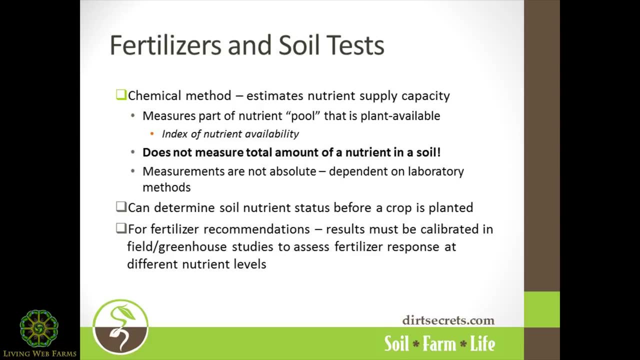 So this led to the rise of fertilizers, specialization in agriculture, the Green Revolution, And soil tests were developed as a marketing tool for these chemical fertilizers. It does not measure the total amount of nutrient in the soil. It measures the nutrients in the soil solution. 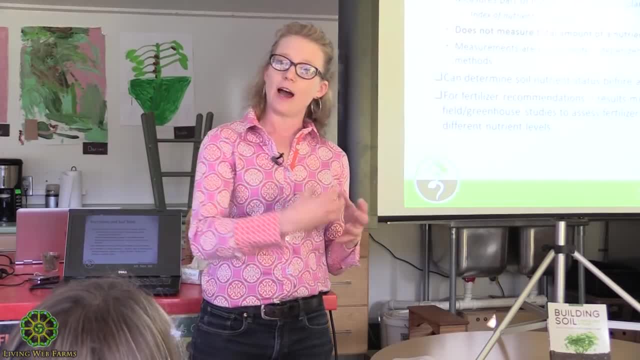 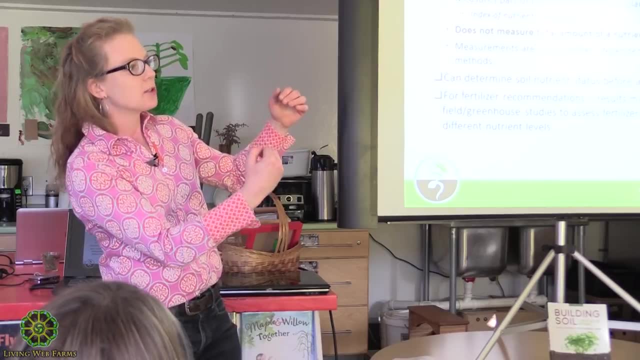 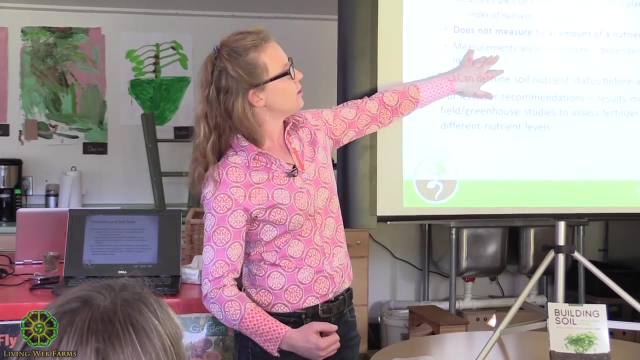 Because fertilizers and there was a lot of market forces for uniformity and industrial processes, so fertilizers weren't focused on feeding the living soil, They were focused on feeding that soil solution and getting it out into the plant. So our soil tests measure the soil solution. 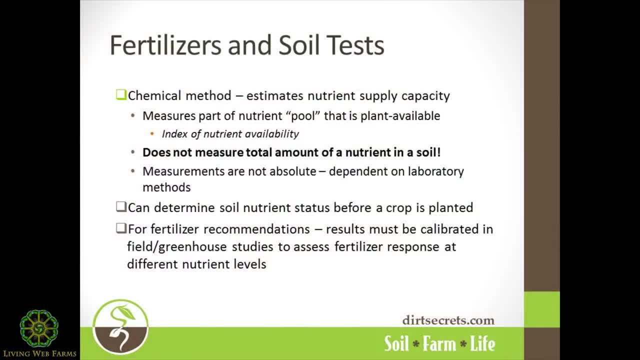 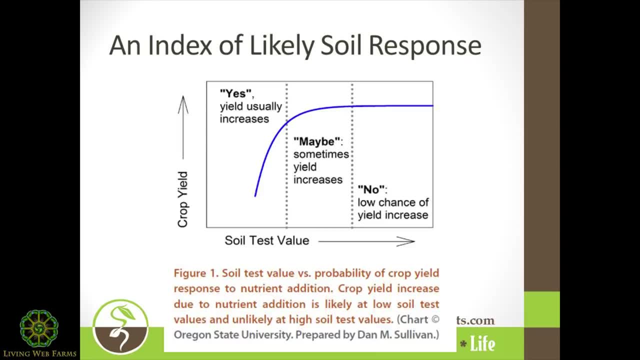 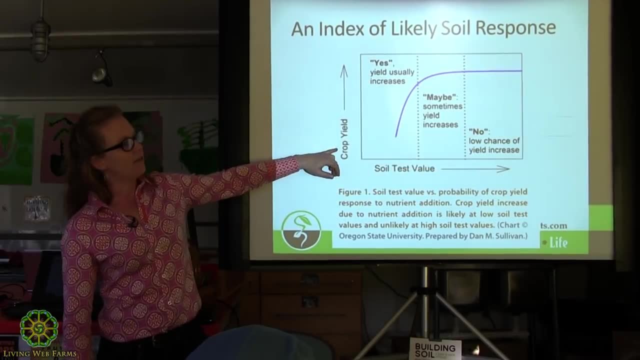 And the fertilizer recommendations are based on correlations and calibrations in greenhouse tests and field tests with the likelihood of a response to fertilizers. So these soil test values were correlated with how much of a response in crop yield you would get from applying fertilizers. 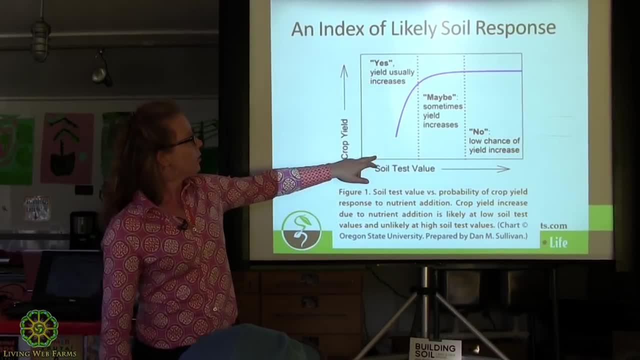 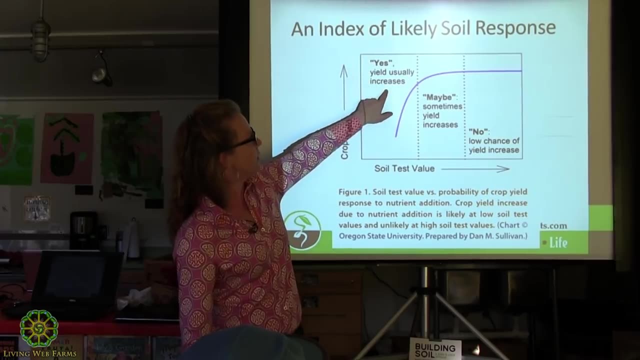 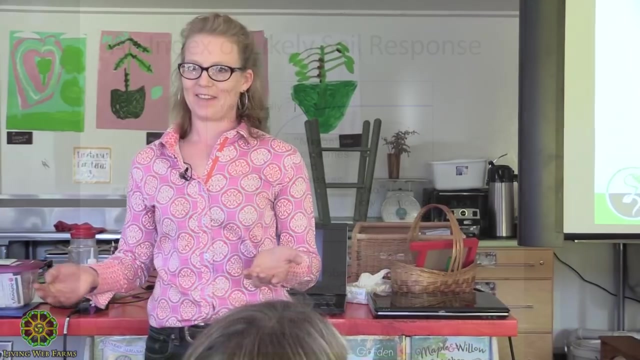 Okay, so at a very low test value, you saw a big. you would see a big response, a yes. Yield usually increases with the addition of fertilizers. okay, So imagine this in a biological system, right? Do you think you're going to see? 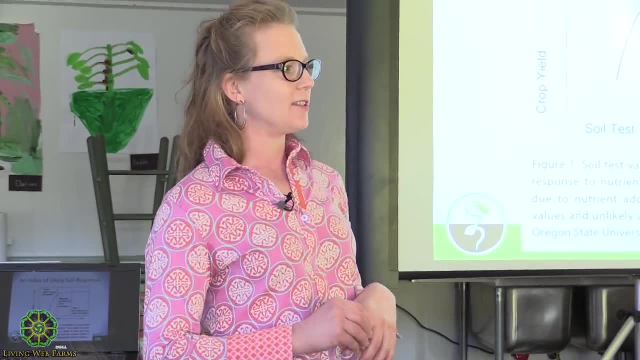 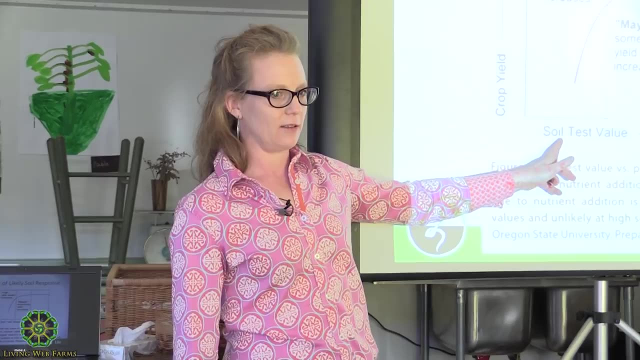 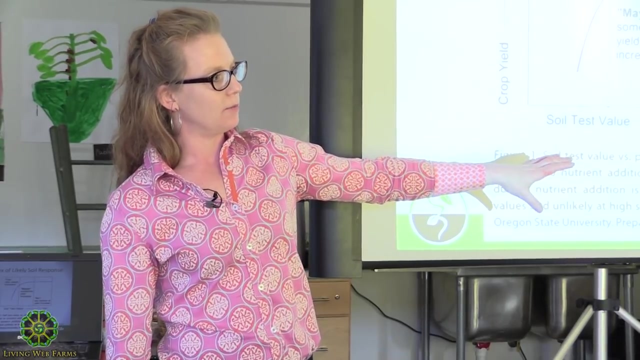 as much of a response in a biological system that is accessing these organic pools, even if you have a very low test value? It's kind of a tricky question, but that's not calibrated. Our biological organic systems are not the systems that they're calibrating. 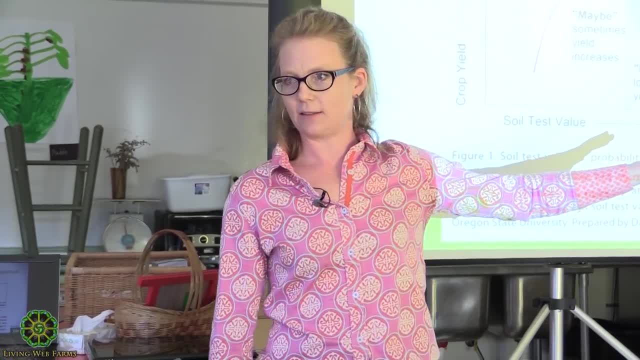 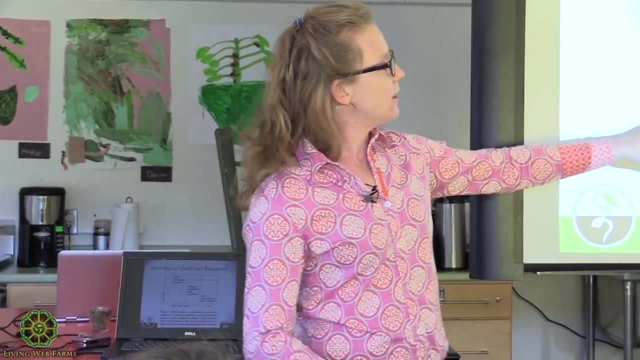 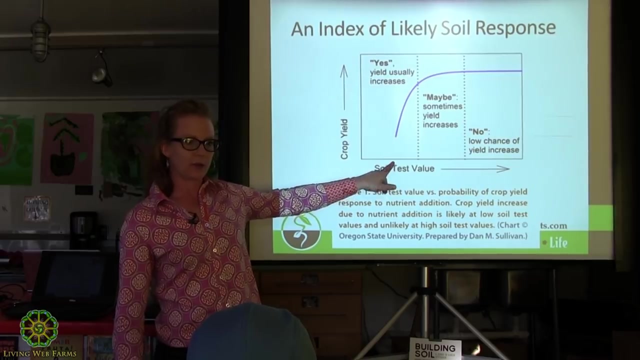 these soil test responses for? Does that make sense? So there's a lot of synergies, a lot of things that play in these natural ecosystems accessing nutrients that our soil test is not accessing. So our soil test value for our biologic organic system. 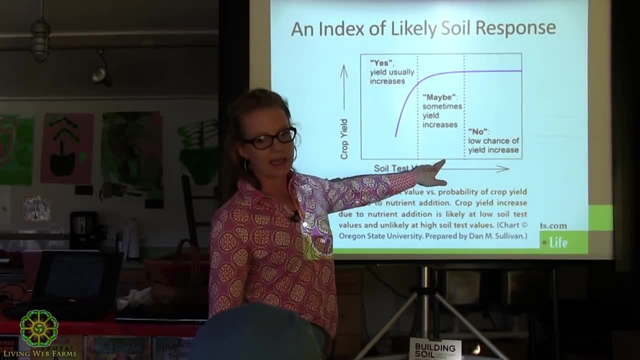 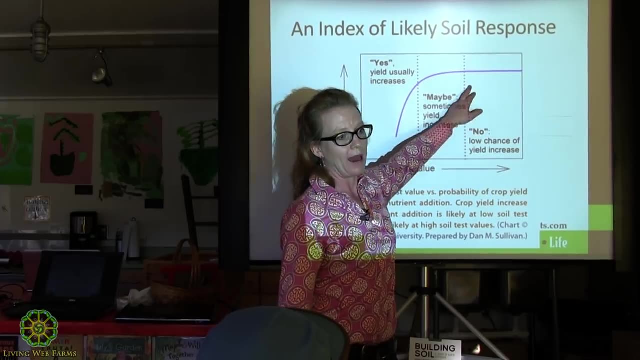 might be down here, but when we actually apply a fertilizer, we might only get a response, a very low response. no, a low chance of yield increase. We might even get a negative increase maybe. So this is why it's pretty tricky for us. 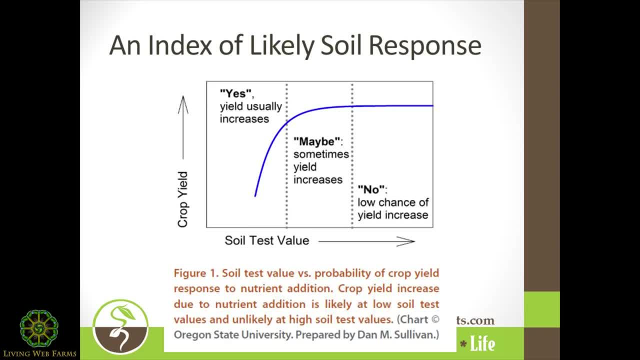 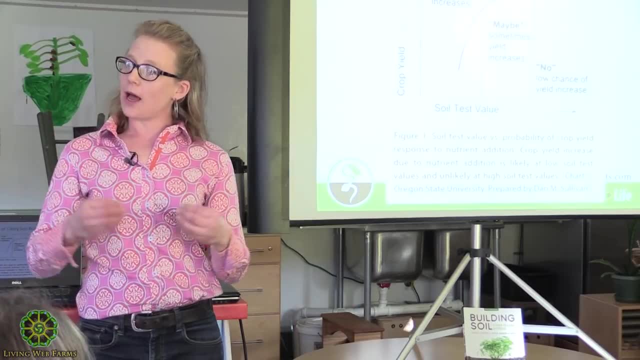 in organic, sustainable systems, and this is why I get a lot of people coming to my soils class, because people are confused, because it's confusing, right, But I think understanding where it comes from it is a tool we can use. Soil tests are a tool we can use. 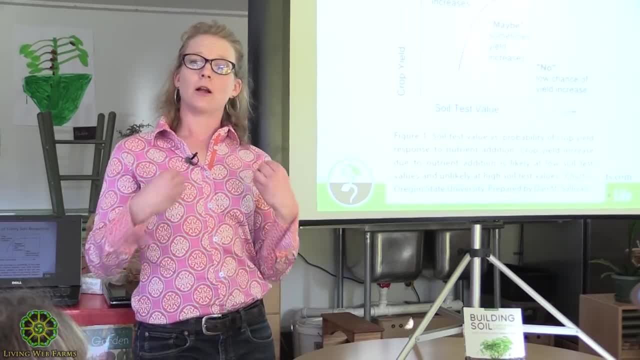 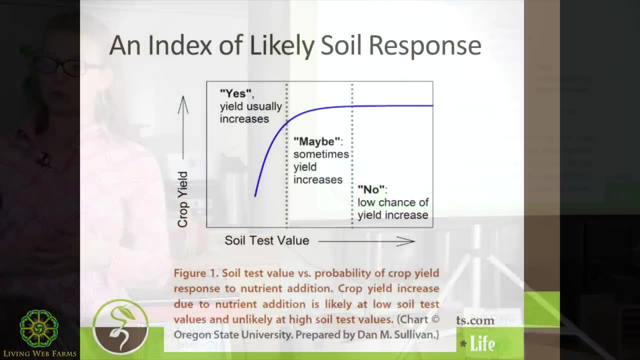 and I definitely think it's worth the investment, especially if your money or your, especially if your love and your labor are really invested in your project. It's a good tool, especially here in North Carolina, where it's so important that it's free okay. 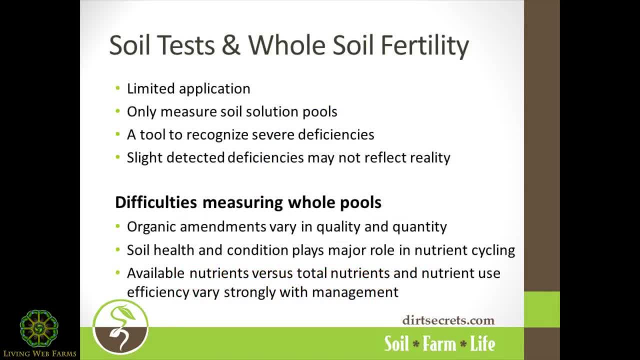 It's an important tool So, like I said, it has limited application to organic systems. It only measures soil solution pools. It is a tool to recognize severe deficiencies and that's why I do suggest that people get it, and we'll talk about which nutrients. 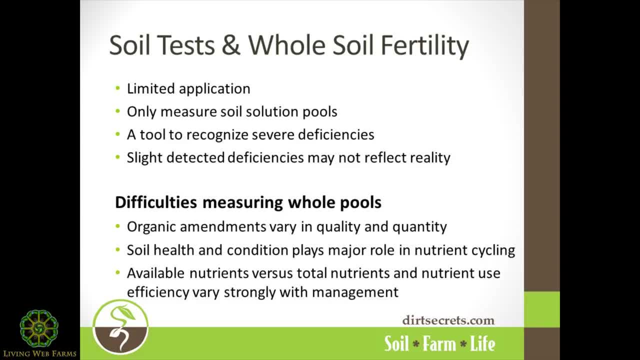 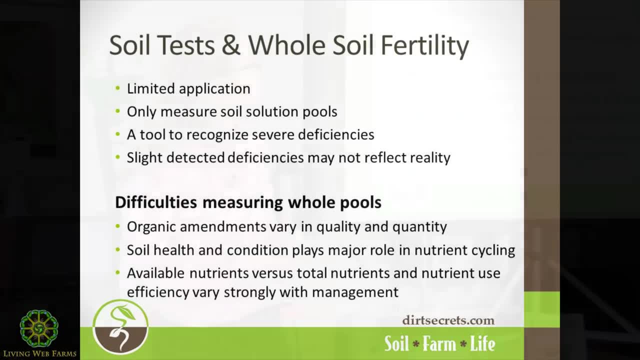 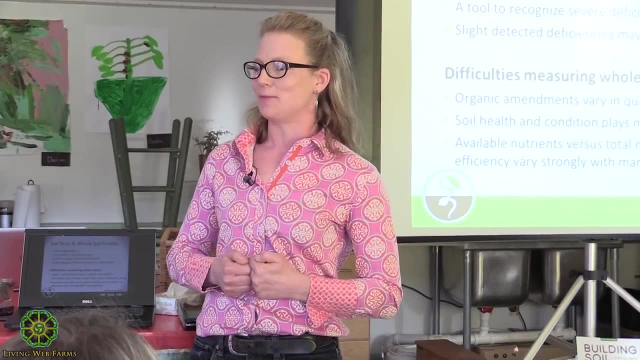 it can be most useful for, But slight detected deficiencies really may not reflect reality, because of what I'm talking about, about this biological system At the same time. well, it would be nice if we just developed some tools for organic systems. It's really really, really hard. 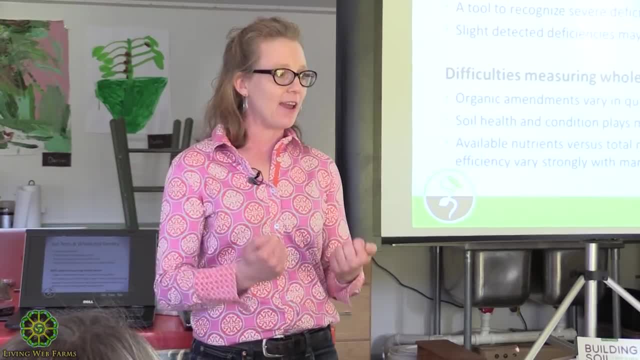 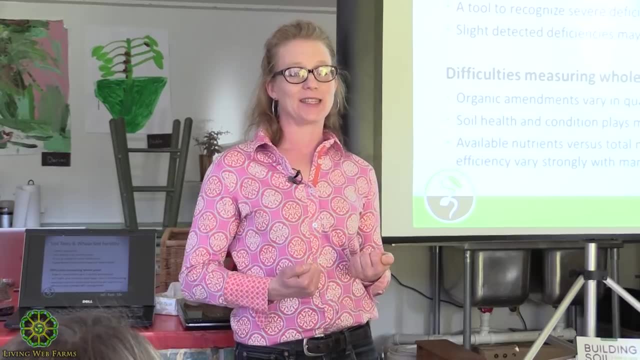 Organic systems are incredibly variable. Life is incredibly variable. If you're a biologist, if you're an ecologist, you know that doing research in these systems is very hard. We were just talking about some different results we were both exposed to just in cover crops. 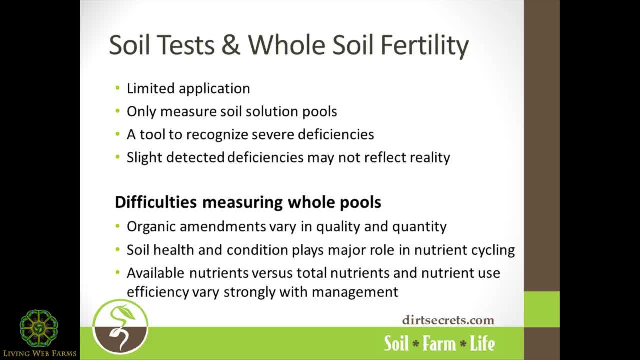 So it's really hard. It's hard to quantify organic emissions. It's hard to quantify organic amendments qualitatively in terms of their nutrient contents. Soil health and condition play such a major role in nutrient cycling. We'll talk a little more about that. but it's very hard to know how your specific system's going to react to the same nutrient inputs. If you're already doing fine and you add additional nutrients, you're going to keep doing fine, Right. So it's not really worth the cost of adding those nutrients. 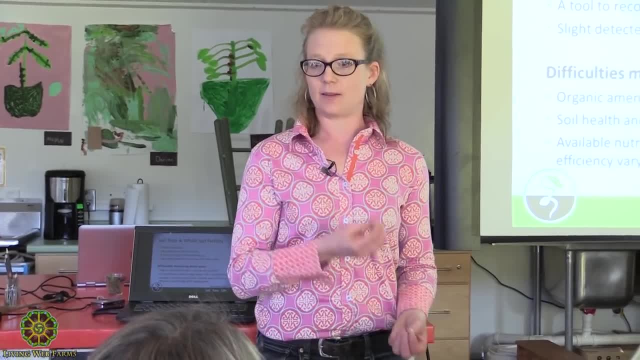 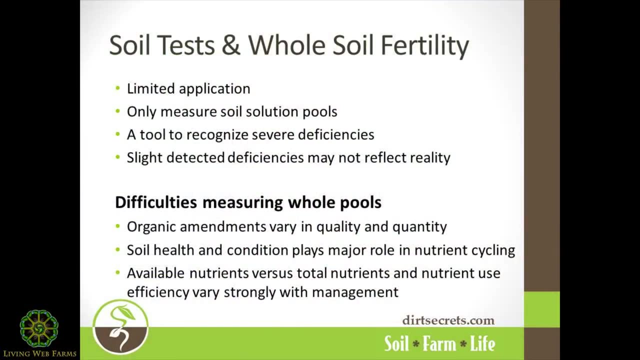 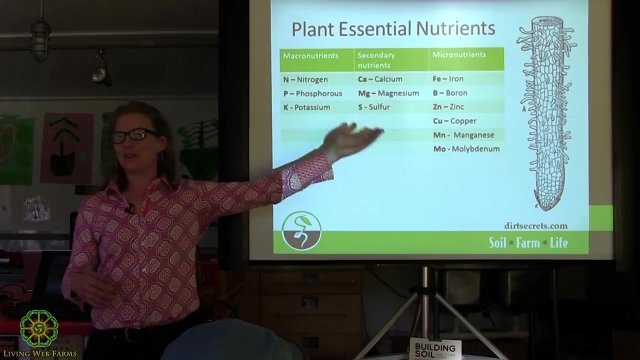 If you're really not doing well and you add nutrients, you're going to see more of a response, But it's hard to know where you are on that spectrum. Okay, so let's go through some fundamental concepts. So if you've looked in any 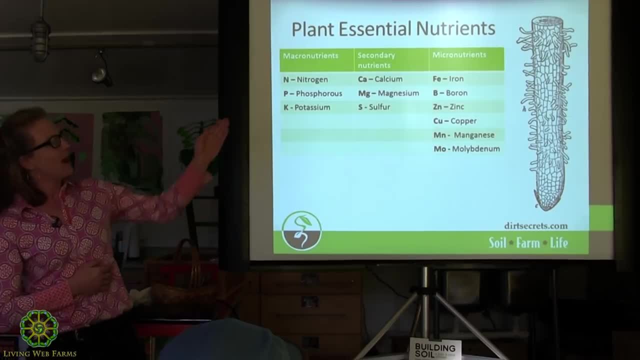 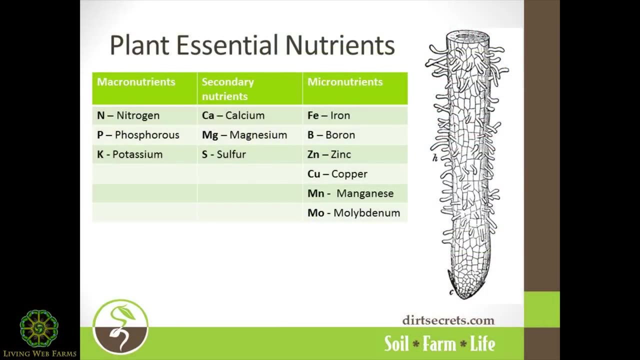 soil nutrient textbook, you'll have seen something like this. So we have our macronutrients. This is what we manage for the most. It's what the plant uses in the most quantity And it's very important For plant growth, for root growth. 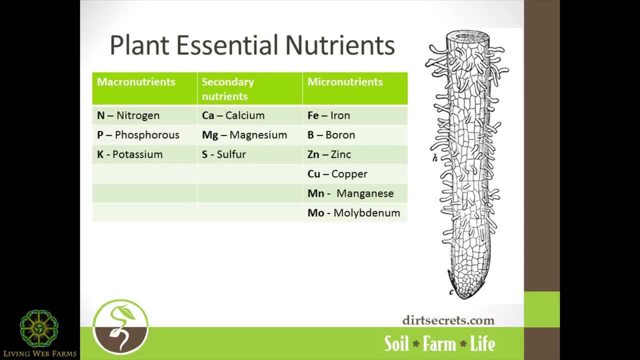 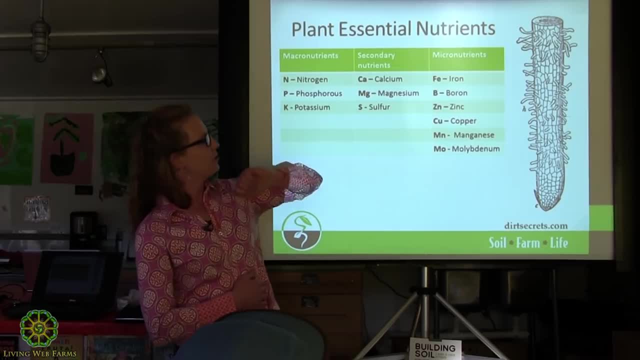 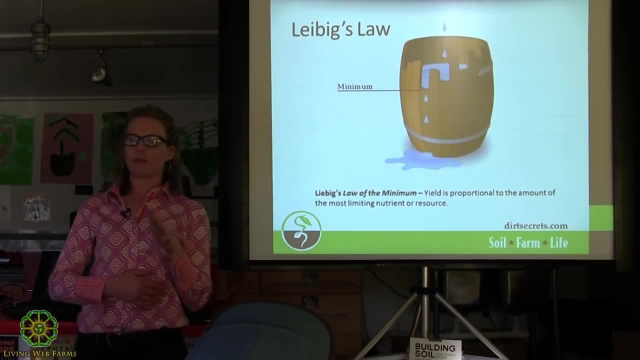 for fruit set for fruit production In excess. it can be equally negative for plants and for our crops. Secondary nutrients: calcium, magnesium, sulfur, micronutrients. Okay, the thing is, if any of these nutrients, if any resource a plant needs, is limited, 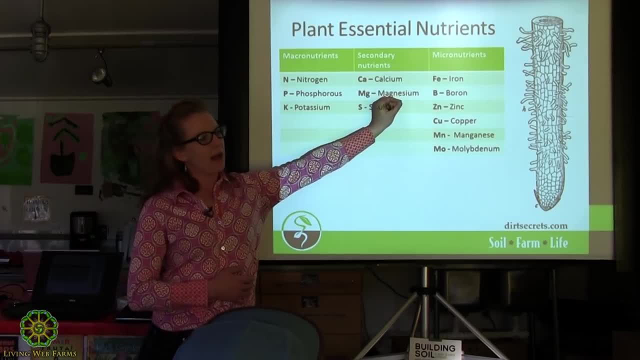 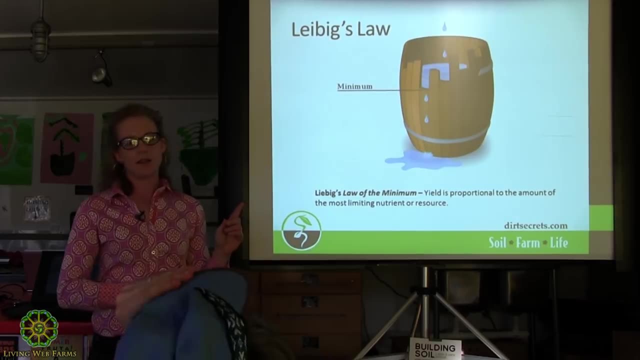 even if we only need that resource on a very micro scale. if any one of the essential resources or nutrients our plants need is limited, then it's going to limit overall yield. Okay, so this is called Liebig's Law of the Minimum. 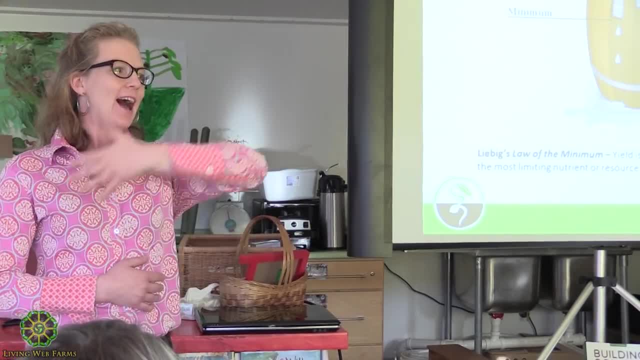 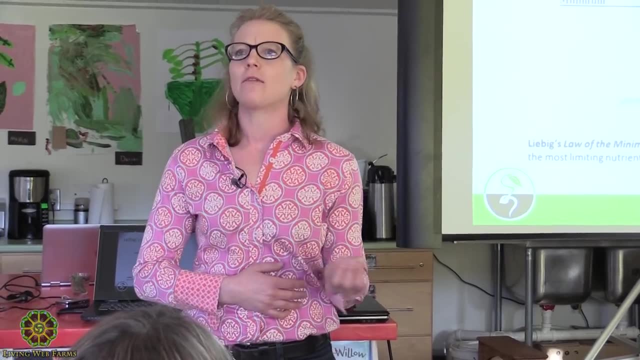 Fundamental concept, But good to keep in mind. So you might have all the nitrogen, potassium, phosphorus in the world. You might have this great biological system If your soils because of the parent rock or past management or some other reason. 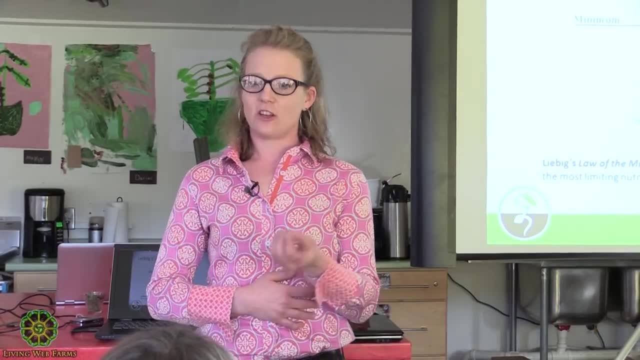 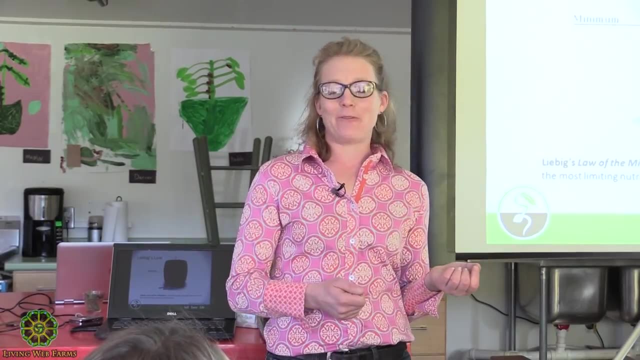 are slightly, slightly deficient in boron, then you're going to have some problems And it might require a little bit of fertilization. And I say a little bit because if you give a teaspoon of boron, you're about right on. 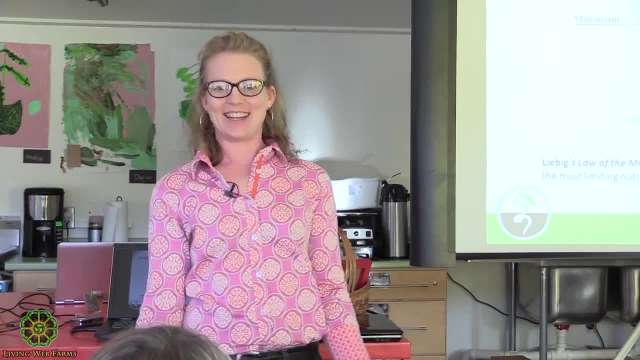 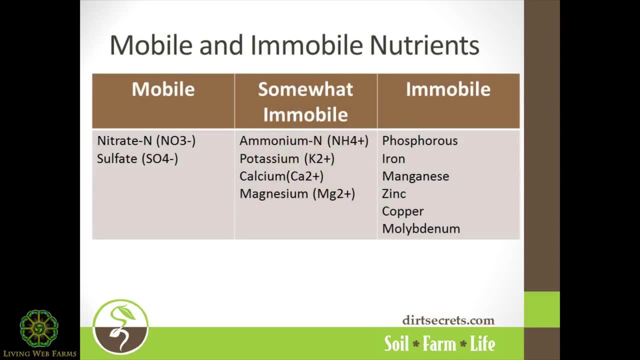 If you give a tablespoon you could kill your plants, right? So it is a very small, sometimes tolerance. Okay, and then it's important to understand which nutrients are largely mobile and which nutrients are largely in mobile in the system. Okay, so any of our positive cations? 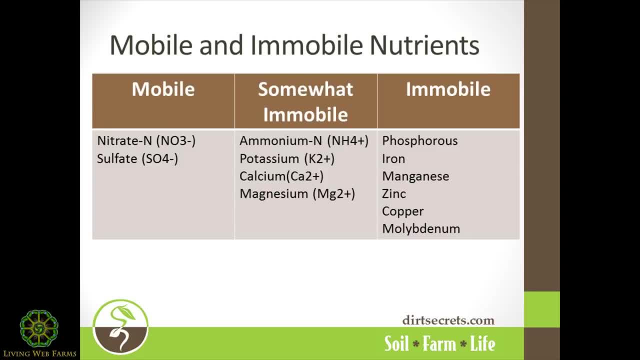 that's nitrate in the form of ammonium, that's potassium, that's calcium, that's magnesium, phosphorus, iron, manganese, zinc. these are largely immobile. okay, These are active in chemical exchanges, so they're sometimes somewhat mobile. 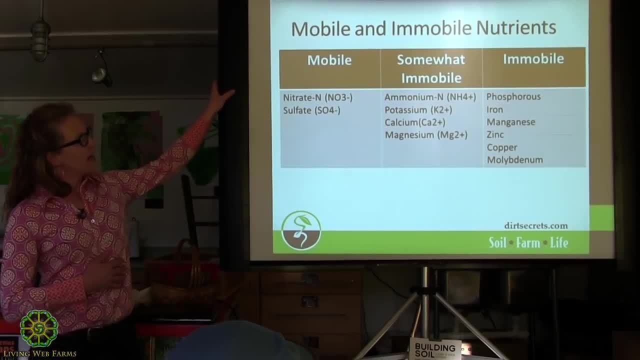 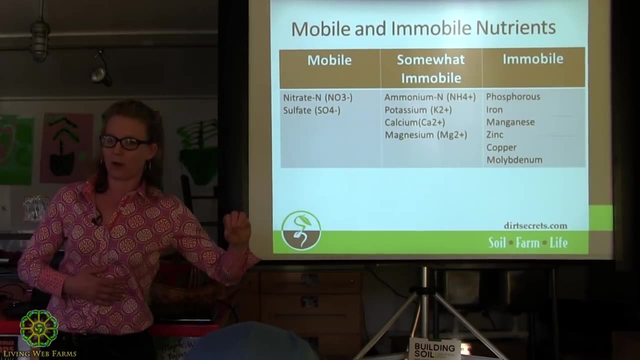 but largely immobile. But the takeaway message here is that nitrate and sulfate and nitrate is one of the dominant nitrogen forms, especially when we're focused on our soil solution, And this is one reason why our organic pools are very important. because they capture and keep this nitrogen In our soil solutions. nitrogen is incredibly mobile and it's easily lost from our systems through leaching, and so is sulfur. We didn't have a problem with sulfur deficiencies as long as we had acid rain. 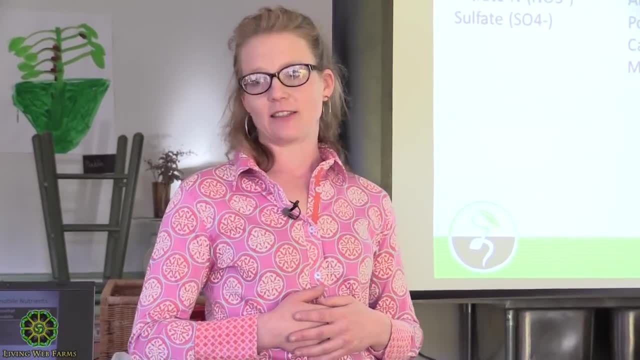 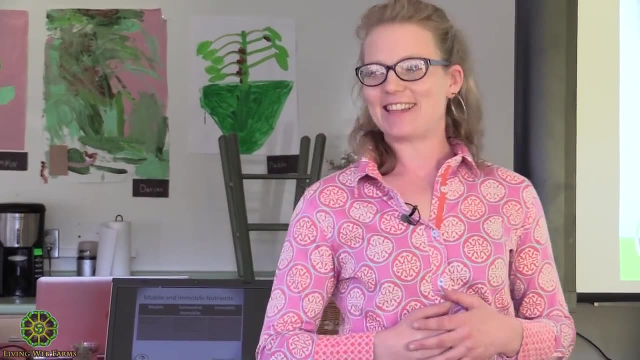 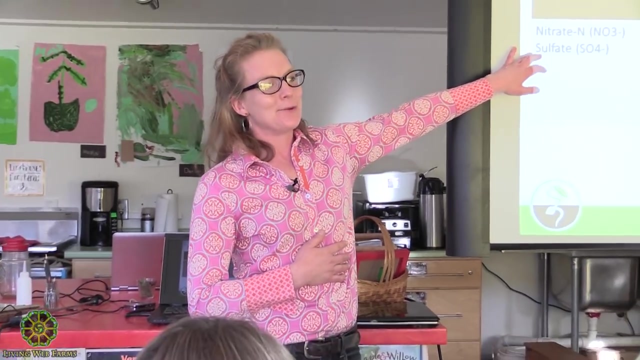 but unfortunately we fixed the problem of acid rain, so now sometimes we have some sulfur deficiencies. I'm just kidding. It's good that we fixed the problem of acid rain. Thank you for laughing, Okay. Okay, but it is a mobile nutrient. 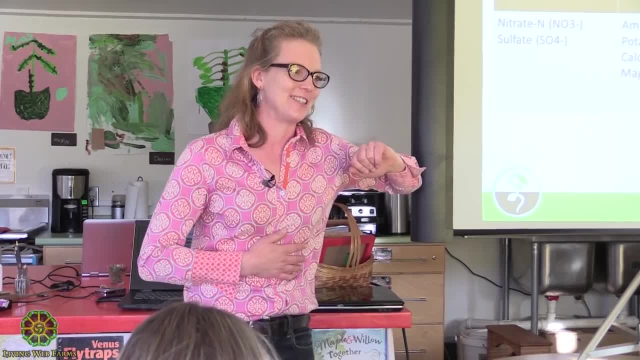 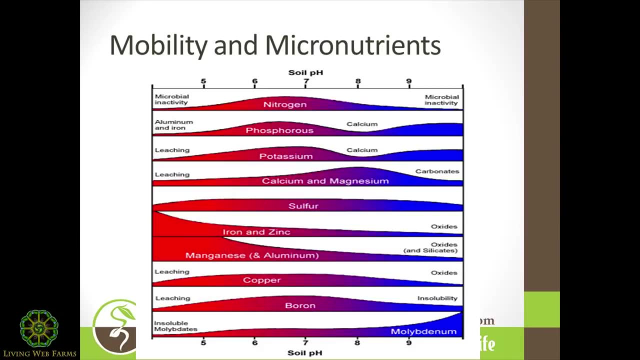 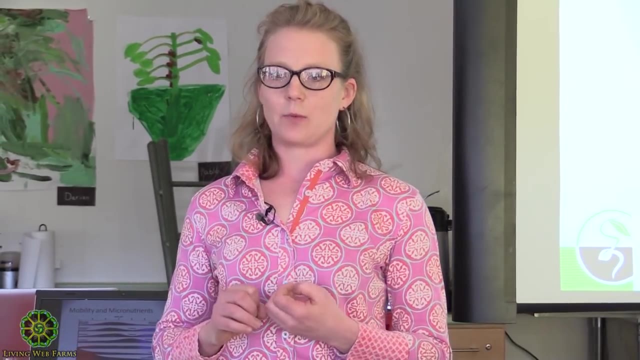 We just were polluting our forests and soils for a while, but also depositing sulfur, Okay, and this mobility is different at different pHs and this is why it's important to manage for pH Okay, and this is why sometimes we have iron deficiencies. 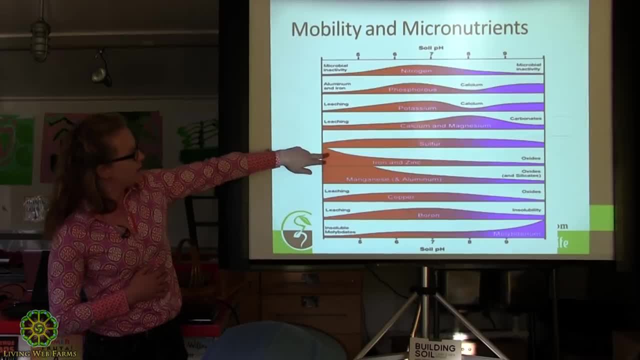 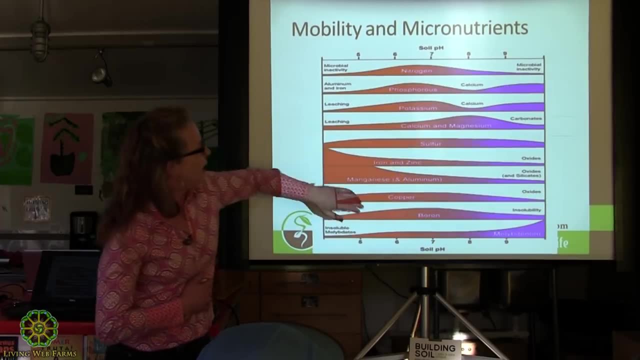 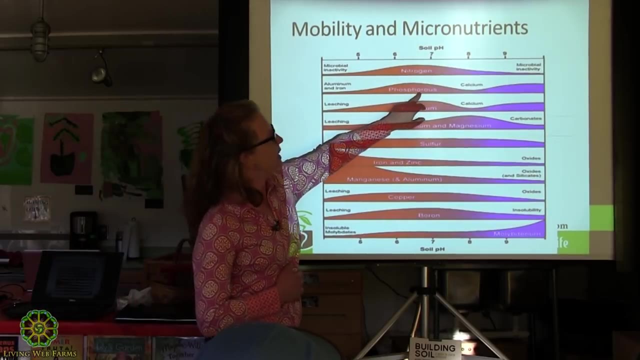 in pretty iron-rich soils because, sorry, yeah, in pretty iron-rich soils. because there's not enough. the pH is too high to have that iron available. Okay, and the same happens to phosphorus. In alkaline soils, phosphorus becomes. 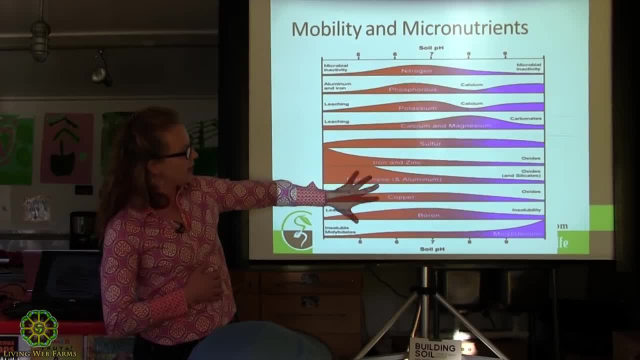 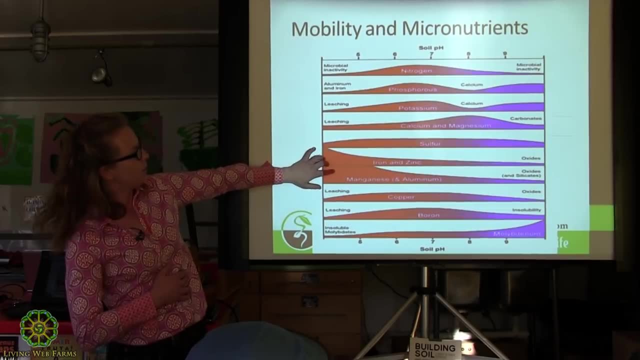 very unavailable. Okay, so it's actually more of a factor in some of these. Actually, we don't want this really acidic, acidic conditions, because we actually have aluminum toxicity here. Okay, so it's important to understand both in availability and toxicity. 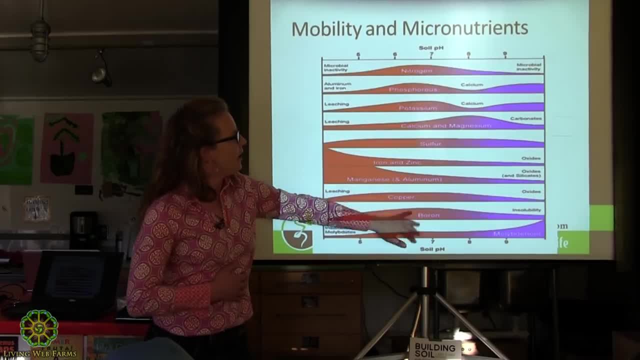 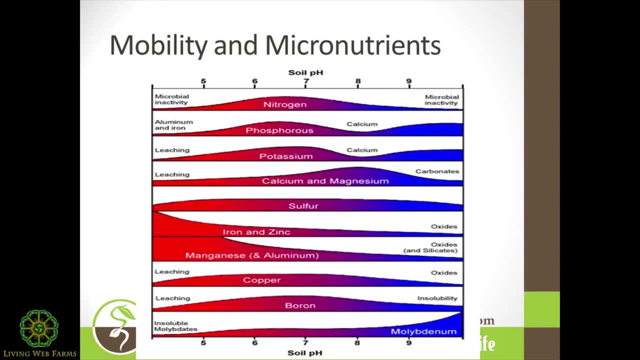 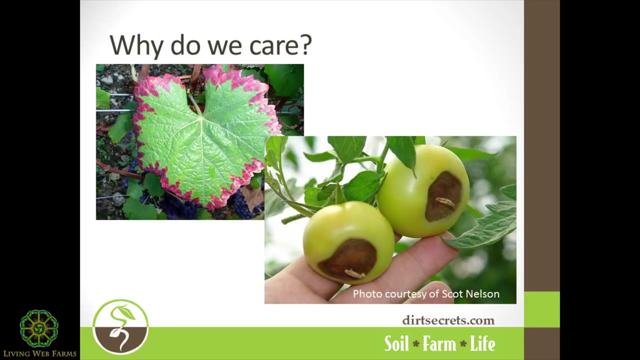 from nutrients. But this is why we manage pH more or less for this neutral to slightly acidic range, because we get the most availability of nutrients. So why do we care? Okay, these are some pictures of nutrient deficiencies So you can diagnose some nutrient deficiencies. 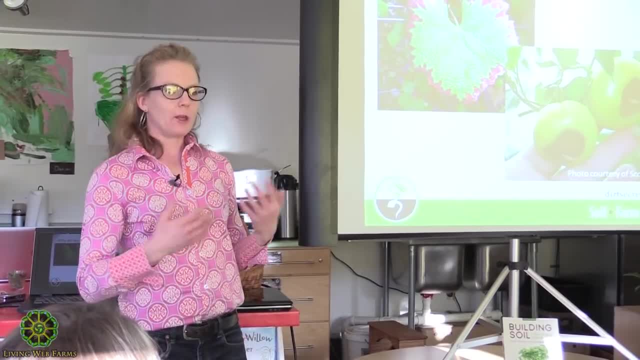 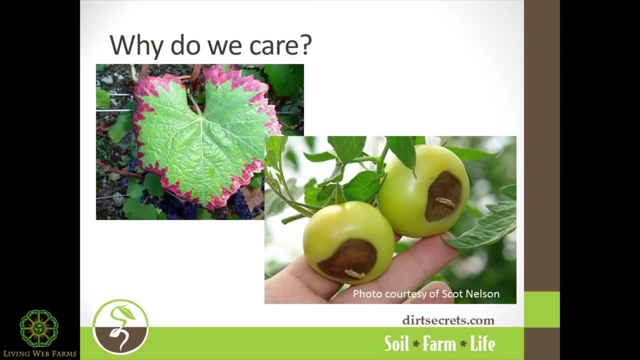 from the way your plants look. Hopefully you won't have to, because you're going to have these great biological systems where you're not going to have these major deficiencies. But you know, blossom end rot can be an indication of calcium, or it can be an indication 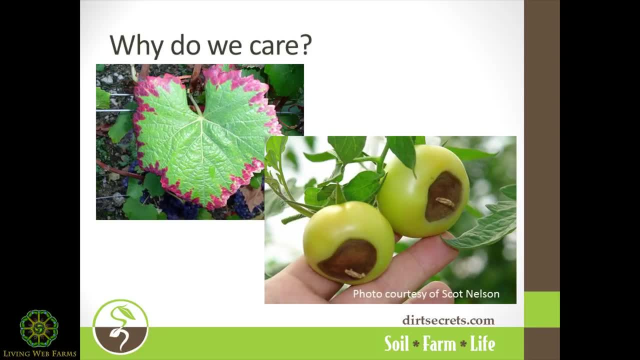 of some other things that make calcium unavailable, or in competition with magnesium, Or you could have these burnt edges, which is often a potassium deficiency. I'm not sure. in this case, Some deficiency symptoms look similar, But most importantly, they limit yield. 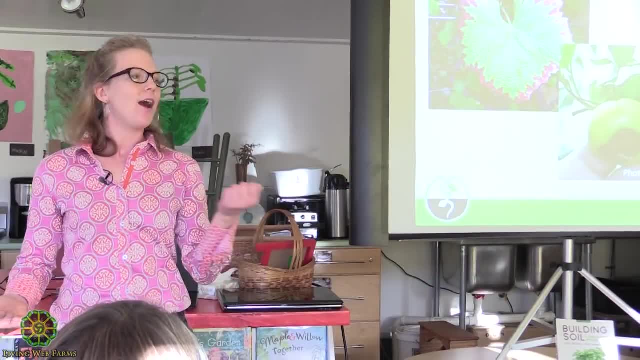 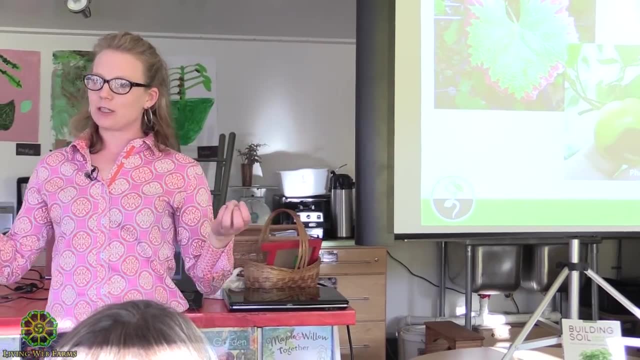 which, when we're talking, I mean for our profits, that's bad. but when we're talking about our living soil systems, that yield is the photosynthetic capture that we get from the sun. That's the carbon that we're pumping into our soils. 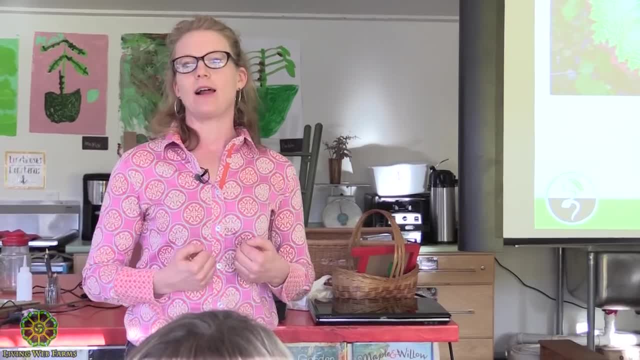 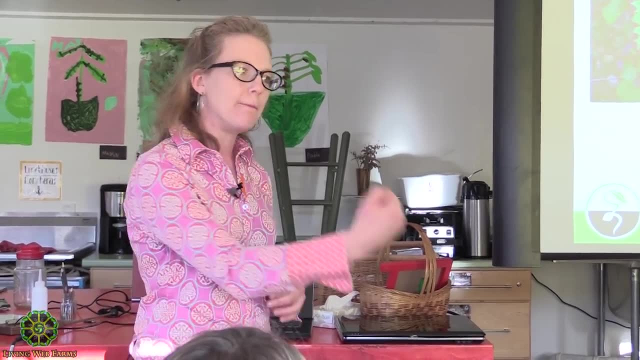 That's why I care, because I want to be pumping that living system full of the currency of carbon, full of the food of carbon. Okay, so I want to maximize my photosynthetic capture. I don't want to limit the ability of my living system to function. 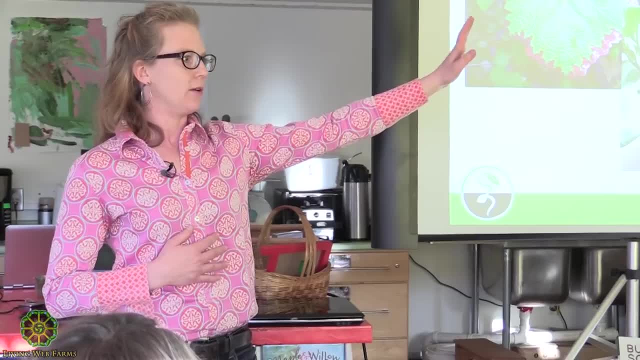 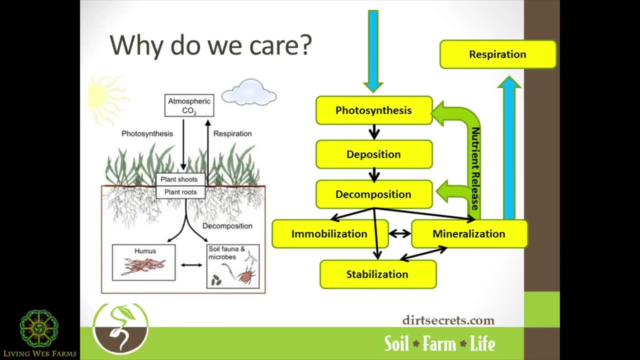 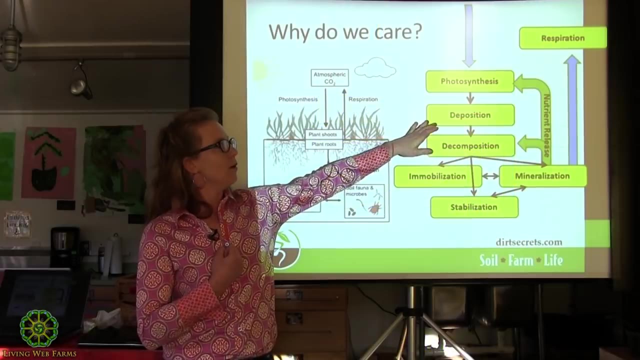 because there's some deficiency from past management or another reason that I haven't addressed. So why do we care? So this is the carbon cycle. okay, So we have photosynthesis, capturing carbon from the air, pulling it into the plant tissues. We have deposition of that carbon. 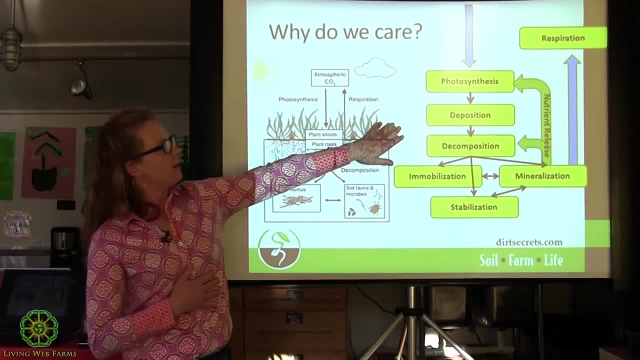 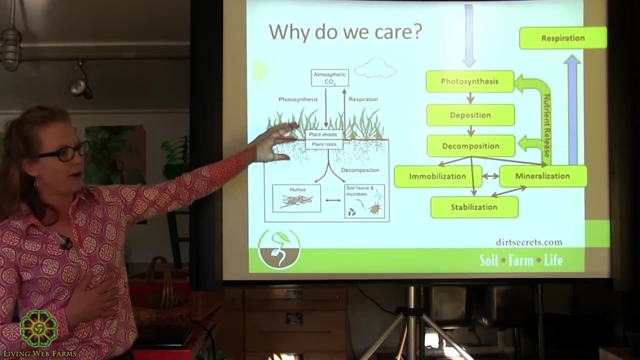 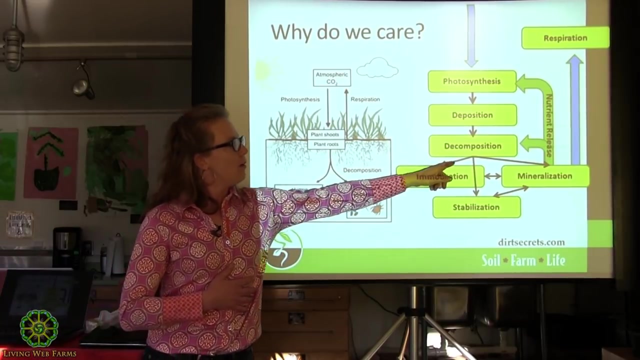 and, in the case of nitrogen fixing legumes, deposition of that nitrogen from the plant tissues, the roots sloughing off above ground, parts of the plant being incorporated into the soil, And then we have decomposition of that plant matter. Part of it is immobilized in the bodies. 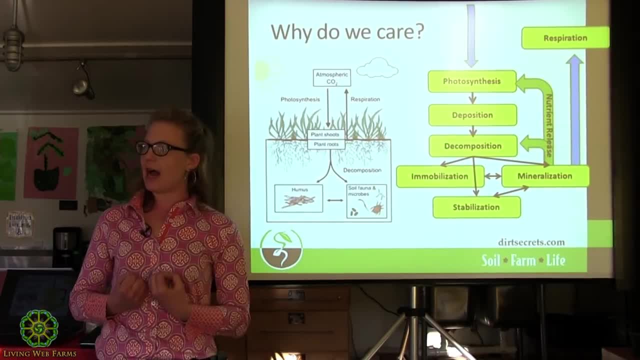 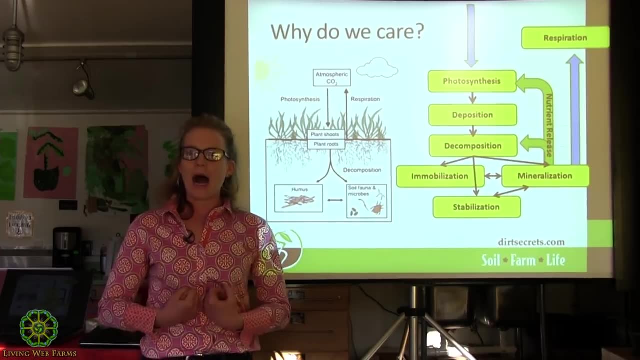 in the actual bodies of the microorganisms. So people ask me: oh, isn't it bad when you put carbon down because it immobilizes nitrogen? That's what we mean. We mean that it's in the bodies of the microorganisms, And that's actually a really good thing. because those microorganisms are going to die and release it again And then they're going to eat each other and put it back in their bodies. So that's keeping it, like I said, in those organic pools, not in that soil solution. Of course it depends on when we need that nitrogen, when we need those nutrients. But a lot of it's also mineralized, Like 70% of the plant materials or the organic matter deposited is mineralized because decomposition, especially in our living systems. 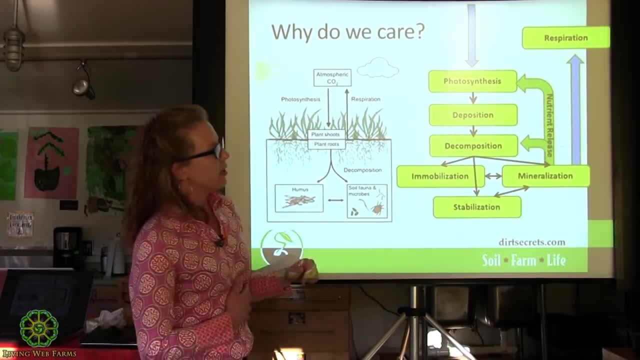 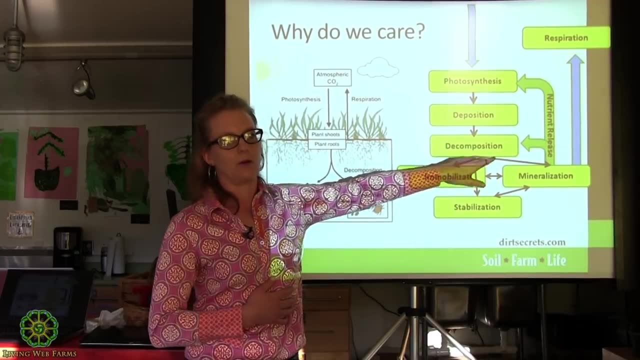 is a pretty fast process. When it's mineralized it's going to release nutrients that go to pump this decomposition and pump this continued photosynthesis. So it's going to drive production And some of what's decomposed isn't decomposed. 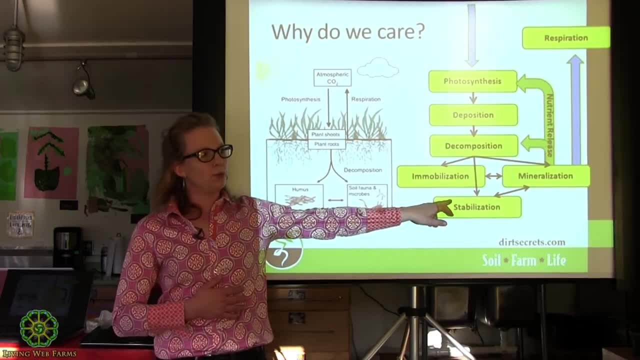 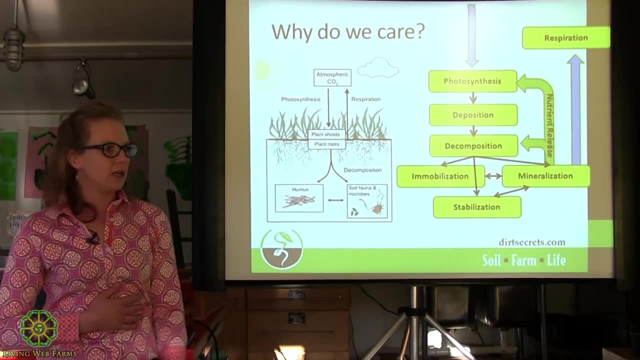 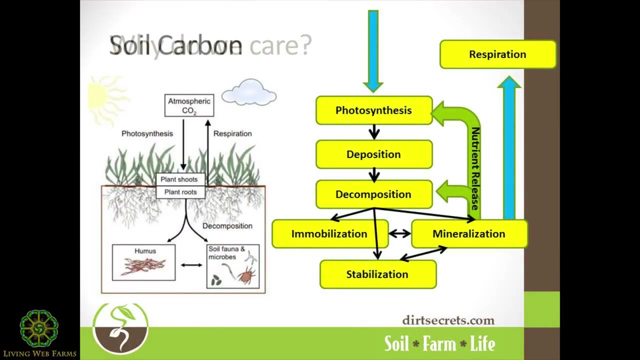 and it's stabilized in these really, really old pools of organic carbon that accumulate in our soils over time and are really important for long-term nutrient, long-term carbon sequestration. So I want to maximize my yield, I want to maximize my living plants. 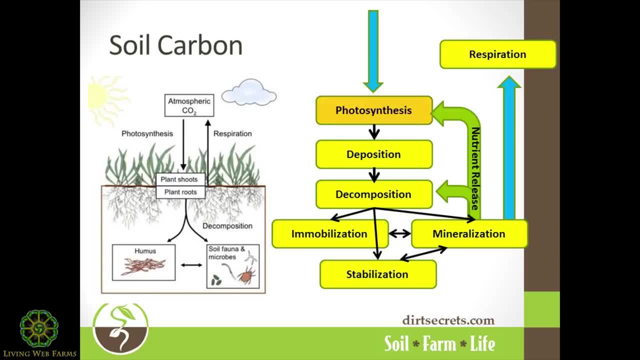 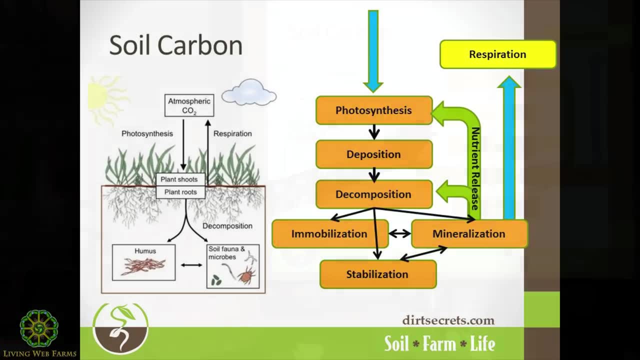 I want to maximize my cover crops because I want to maximize that photosynthesis which maximizes this whole process. Right? So I'm going to keep. Can you see how this is a positive feedback? look that when I get it going. 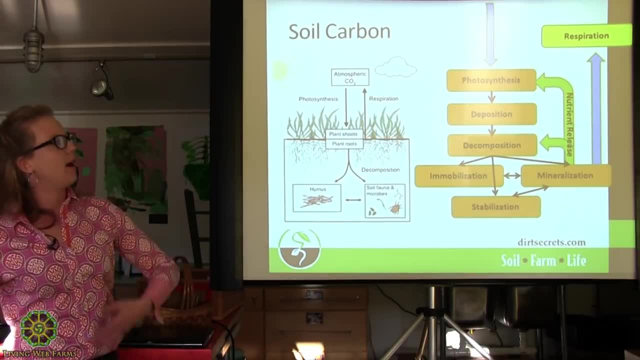 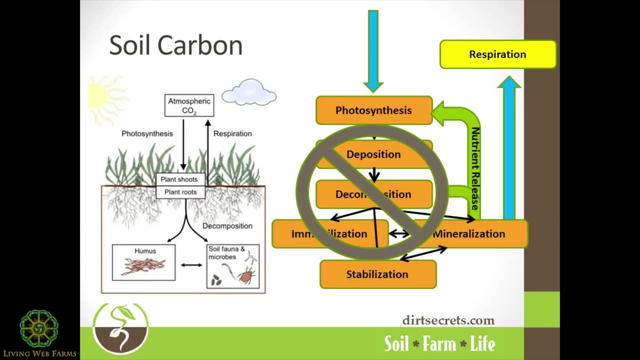 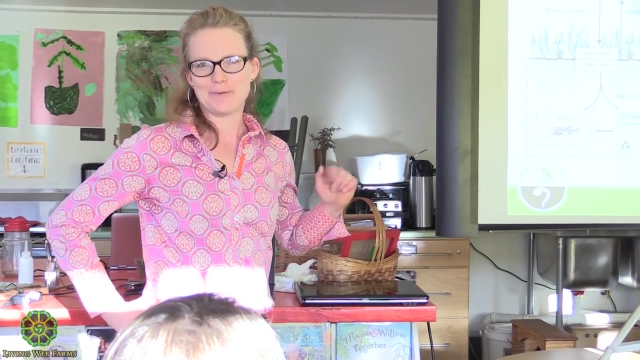 I can keep on increasing the health, the cycling of this system. Oh yeah, I don't know why I put that there. I think because of you limit your nutrients, you lose out on that process. I'm pretty sure Because carbon is the food. 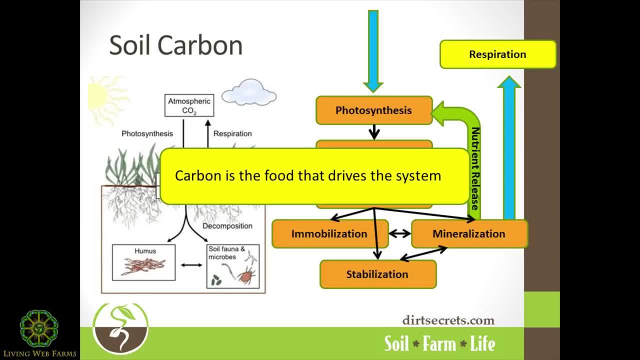 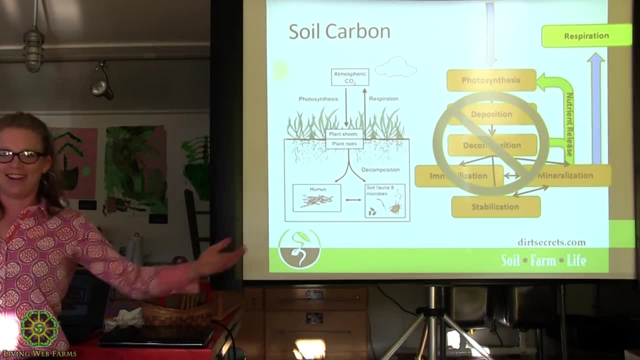 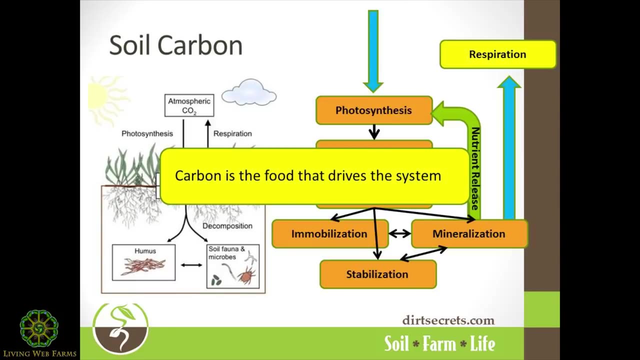 that drives the system. Oh yeah, That's what I was going to say. So if you have less photosynthesis, you have less of this whole process, Because carbon is the food that drives the system, So it's nutrient cycling in here. 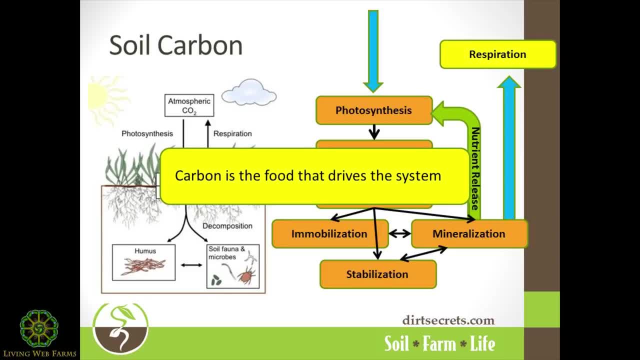 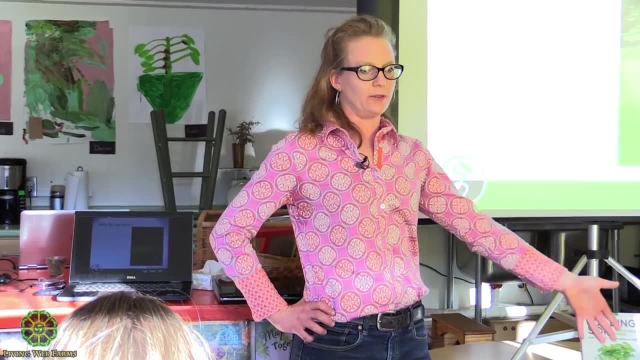 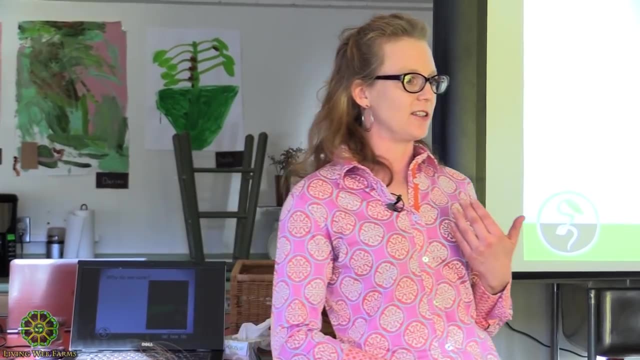 and keeping this whole thing active through this active carbon cycling. Why do we care? Because we don't want to continue to pollute our world, So there doesn't have to be this disconnect between our environment and our food production, And I think it's really important. 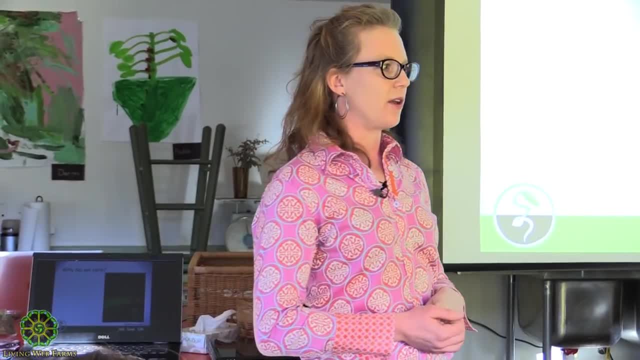 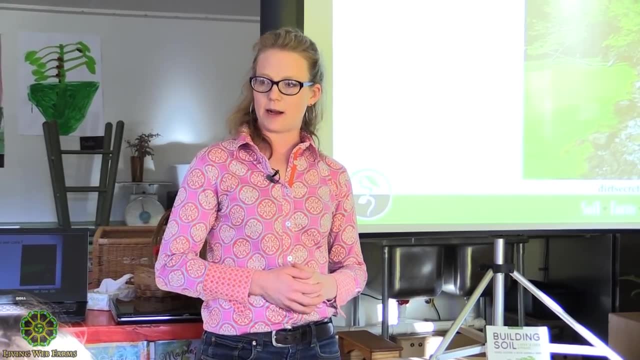 as we face the critical challenge of feeding 9.3 billion people by 2050, that we accept the fact that we're going to have to do it in a sustainable and environmentally responsible way, which means we need to treat our agricultural systems. 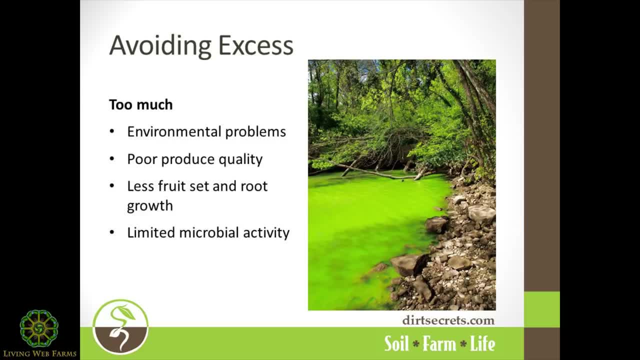 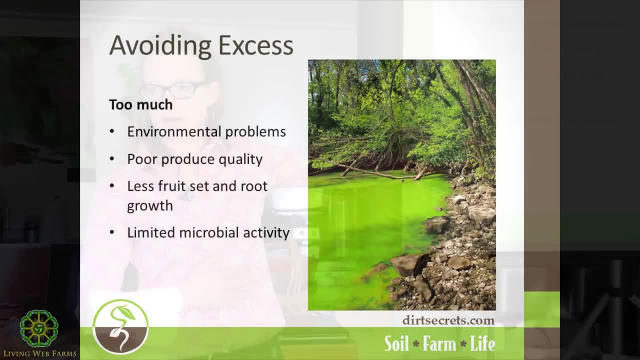 in my opinion, as ecosystems, And also too much nutrients. excess nutrients affect the quality of what we're producing. So if you have too much nitrogen, you produce a plant that's really leggy. It's going to have a lot of green growth. It's not going to have good fruit set. It's not going to have good root development, It's not going to taste good. It's going to be susceptible to pests and disease. It's not going to have a long shelf life. Okay, so having excess nutrients? 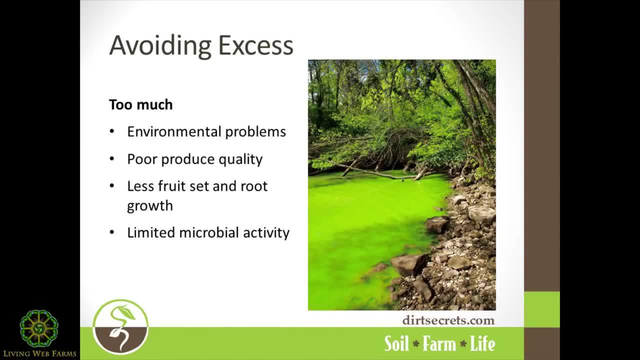 not only does it lead to eutrophication, but it leads to poor produce quality, environmental problems And excess nutrients also limit the activity of the microbes in our soil, So we limit their ability to be efficient agents of nutrient cycling when we're providing everything in excess. 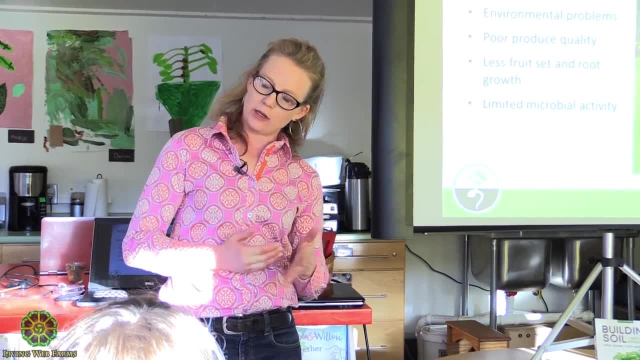 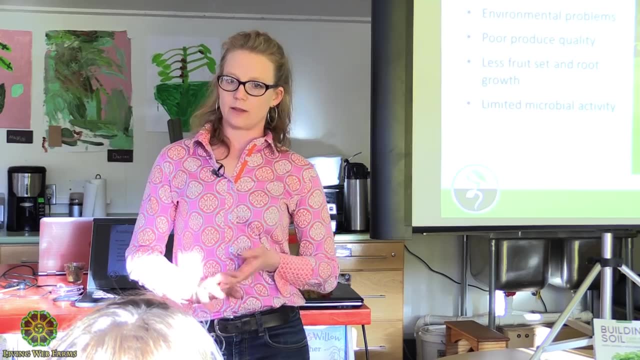 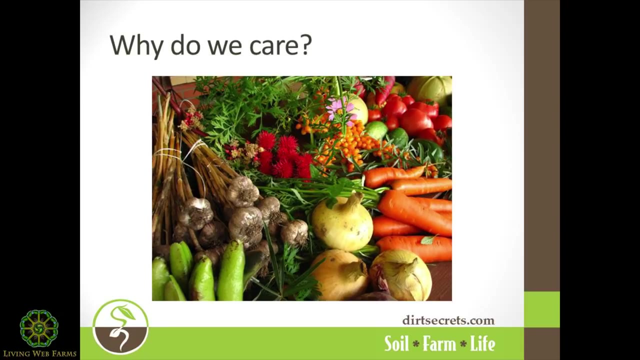 And this is a big problem in inorganic or non-organic systems, but it also can be a problem in organically-based systems, And we see that sometimes with manure applications which can be tricky to manage. Why do we care? Any ideas? 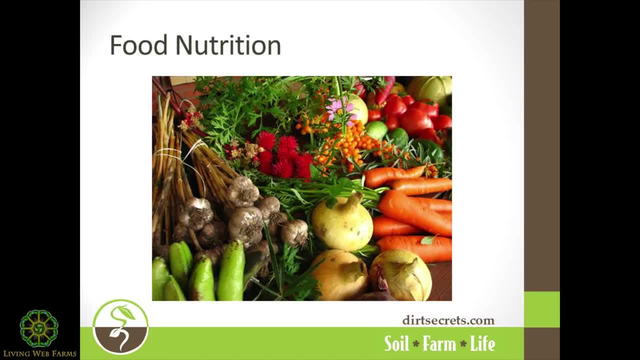 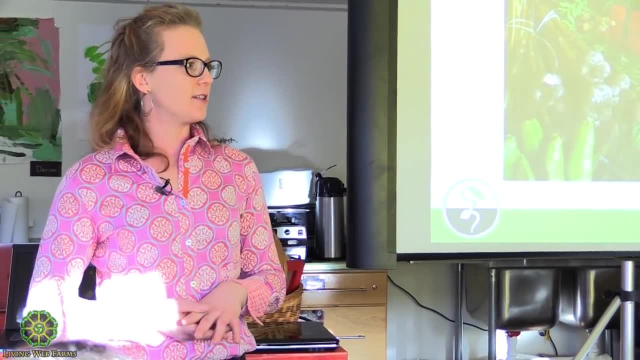 It's the last one, So there's a lot of talk about food nutrition now and the nutrient density of food. In 2004, or in the early 2000s, there was some work done where someone looked and looked at the nutritional density of food. 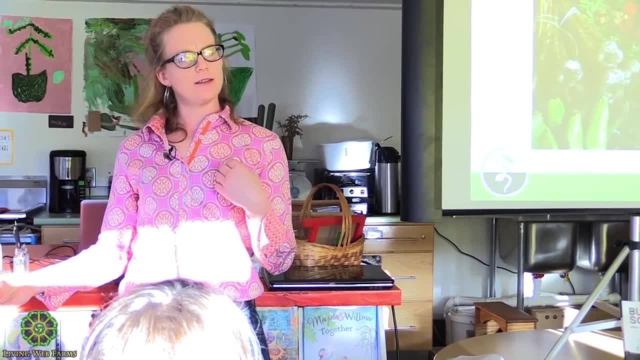 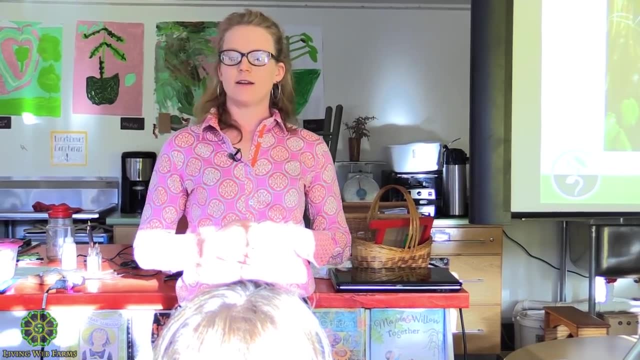 from the 1950s and 1999, I think I believe it is 99 or 95. And saw that in 43 garden crops nutrition actually declined. So you know this is an issue. It's an issue for food security. 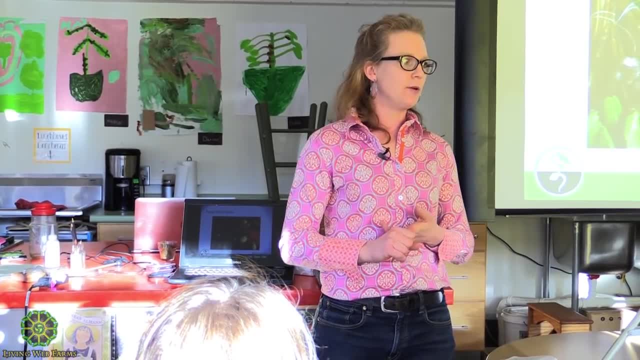 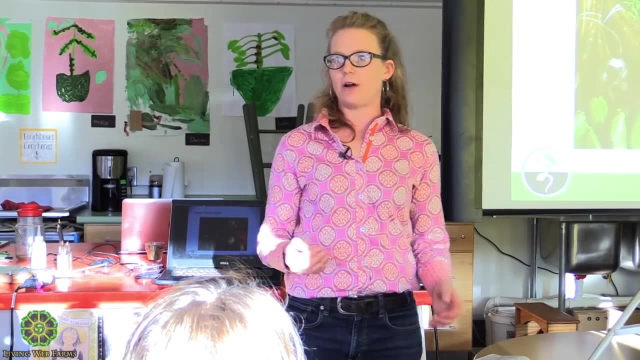 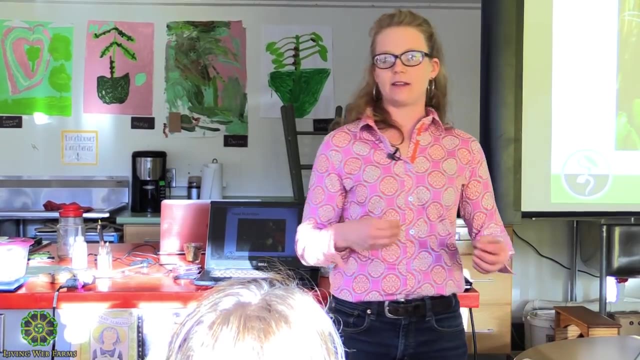 which is not only access to enough food but access to nutritious food. But it's also an issue for, like, the shelf life of food, So you have a longer shelf life. if it has a higher nutritional density to it Flavor, There's more resistance to pest disease. 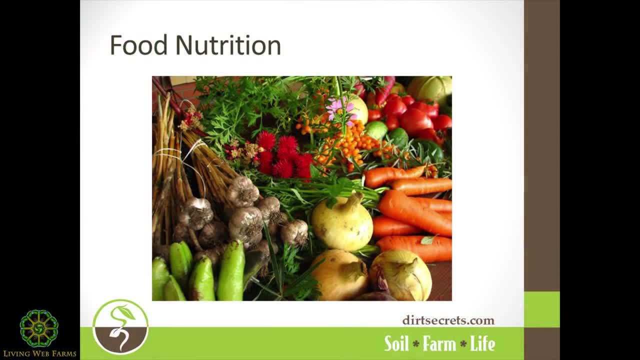 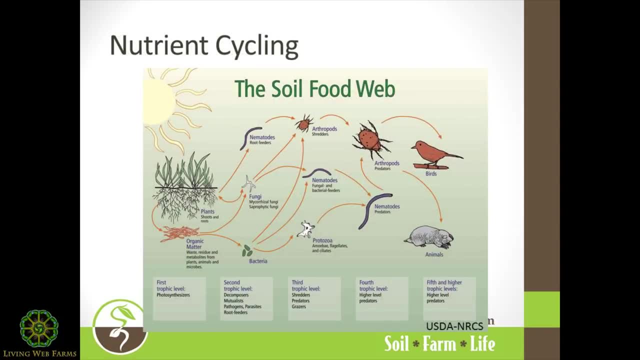 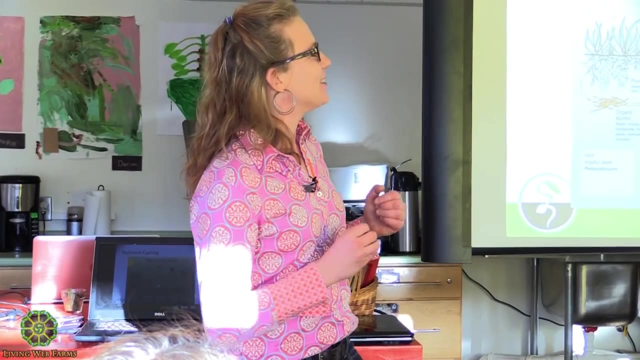 if there's a good nutritional density, Not excess but sufficient. And this is all driven, like I said, who's seen this picture before Everyone? I hope So- by the living soil food web. okay, So biology are the agents. 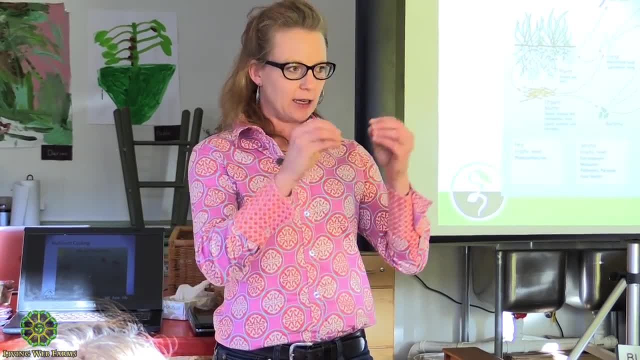 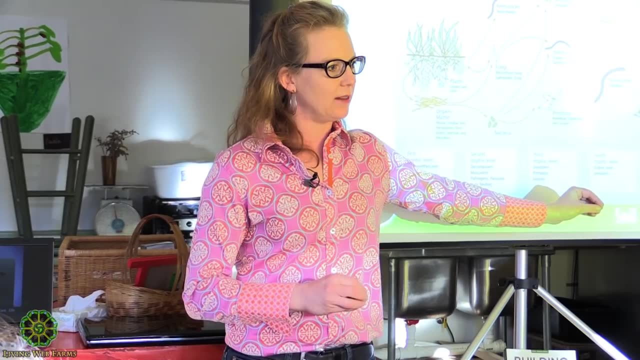 of this nutrient cycling that we're talking about And it is an ecosystems approach. okay, So it is. you know there's many trophic levels. It's important to have a lot of diversity in this system. We get diversity by having diverse systems. 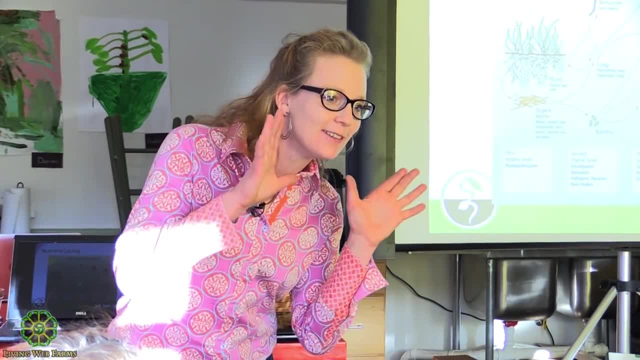 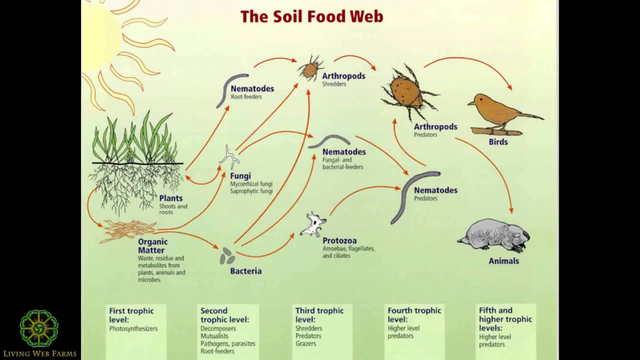 by having animals, Animals, By having animals in our systems, by having diverse crops, having diverse crop rotations- okay So we want diverse microbial food web. We want to give them diverse foodstuffs. Okay so this is the nitrogen cycle. 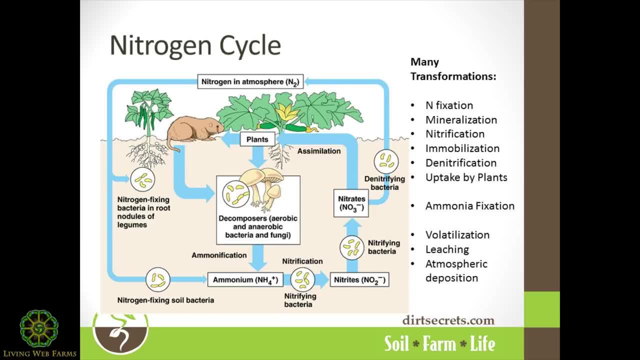 We're not going to talk a ton about it, but it's important to see that nitrogen is on the move. There are a lot of transformations going on. What form we put nitrogen into our soil has a big effect on pH. In general, nitrogen is taken up. 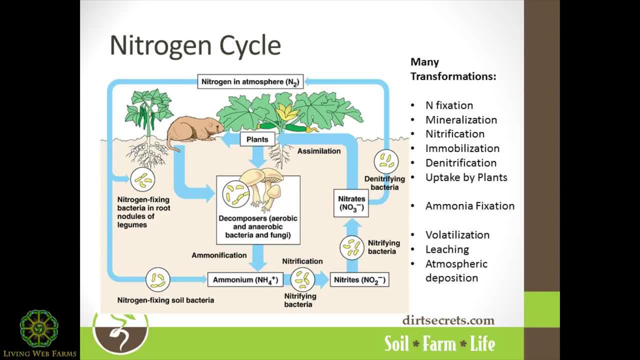 as ammonium or nitrate. There's a lot of mechanisms of loss, including volatilization, Which is a big mechanism of loss of manure or fertilizer nitrogen. especially during transport or spreading, There's leaching, which is a big form of loss. 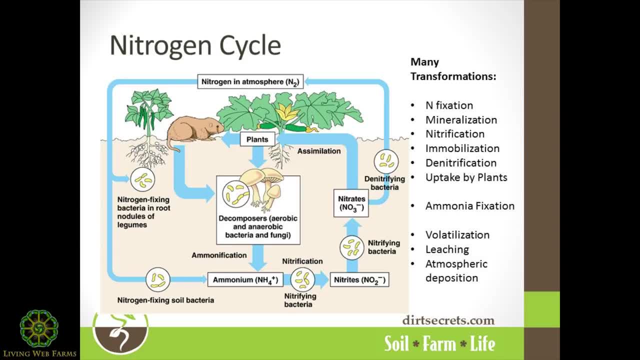 So there's a lot going on and most of this, most of these transformations- the ones on the top, I've separated them- are biologically mediated. okay, Ammonia fixation onto clay minerals is somewhat biologically mediated: Volatilization, leaching and atmospheric deposition. 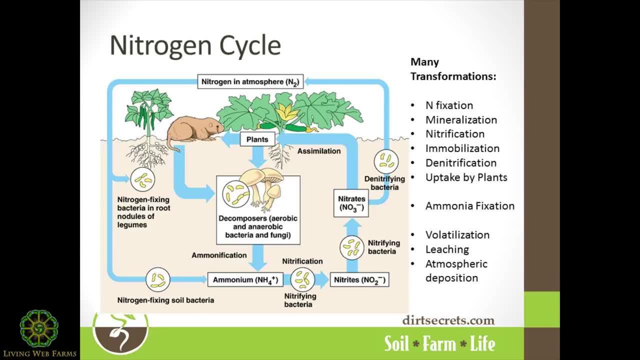 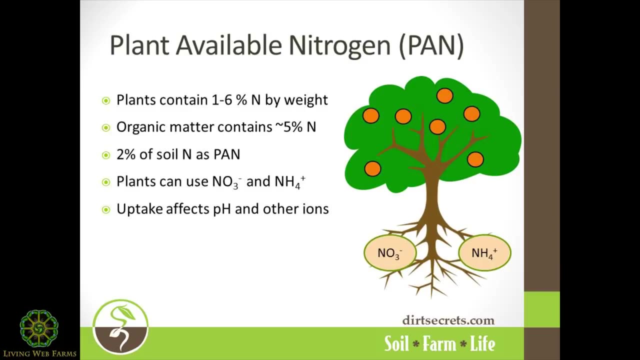 at this time we're not considering them very biologically mediated, but you never know, We could biology's at play, but they're more physical processes. So it's tricky because the total nitrogen in our system is not what our soil test measures. 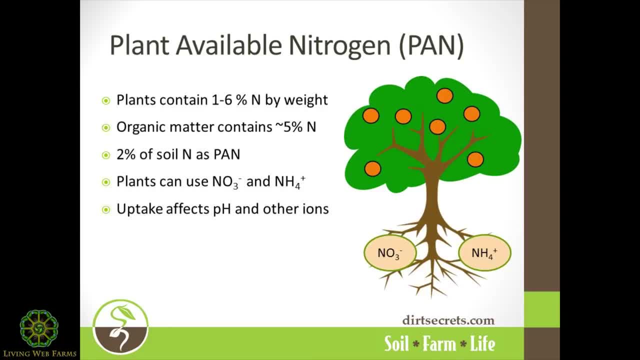 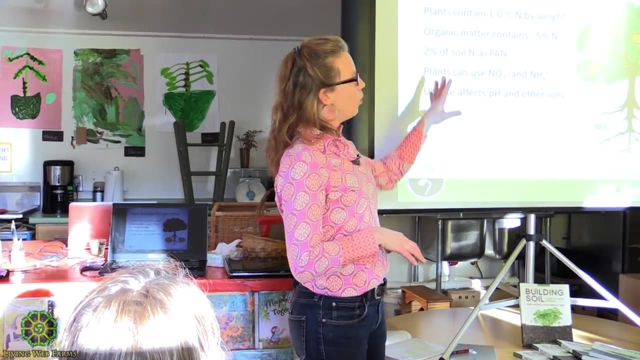 We know we measure soil solution nitrogen, but we do want to have an idea of how much plant available nitrogen we have in our organic matter. okay, So how much of the nitrogen in our organic pools will become plant available during the times that the plant needs it? 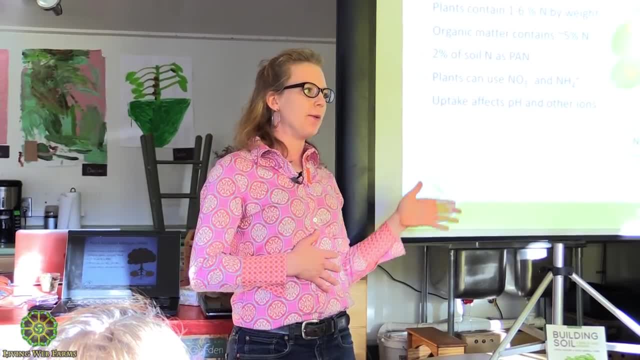 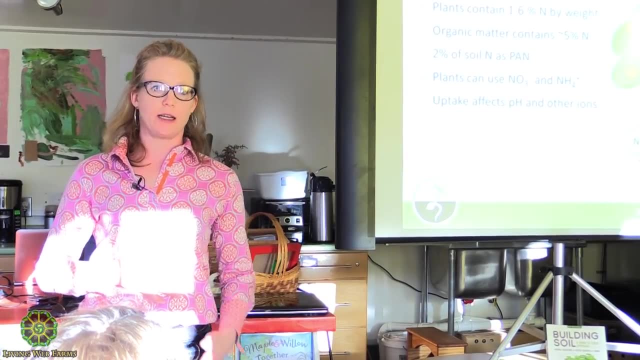 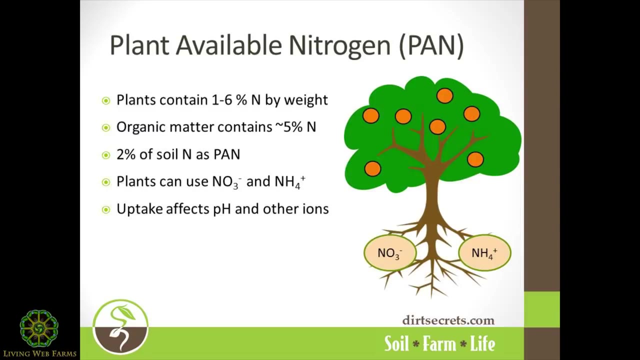 Okay. so this is an important concept and this is something that hopefully new tools, as they begin to develop, will get better at predicting, or helping us predict or at least estimate the plant available nitrogen from our organic nutrient pool, And we'll talk a lot more about that. 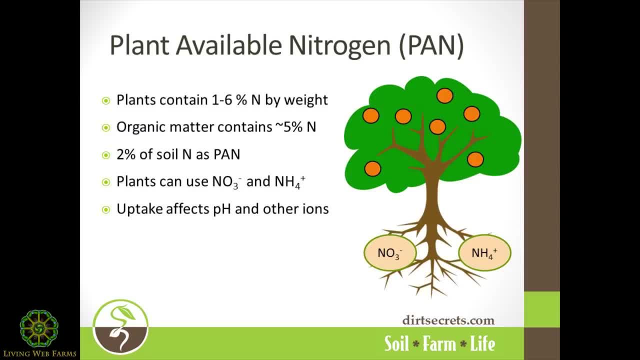 but plants contain about one to six percent. one's pretty low, but six percent nitrogen. by weight, Organic matter contains about five percent nitrogen. Let's see, that seems a little. that's high, for that's the overall pool, A living organism anyway. 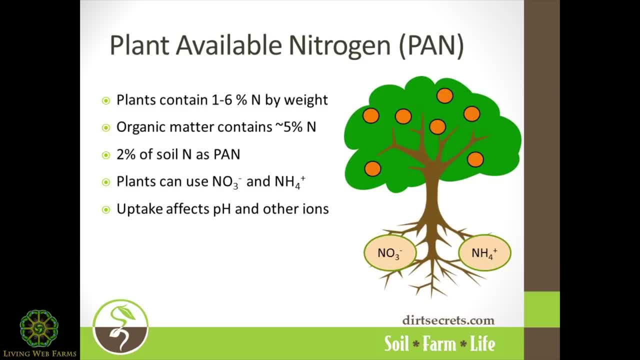 organic matter contains about five percent nitrogen. So two percent of soil nitrogen. so that's five percent of that organic matter nitrogen. two percent of that is usually accessible as plant available nitrogen. Just to show you kind of how these fractions break down. we'll talk more about this. 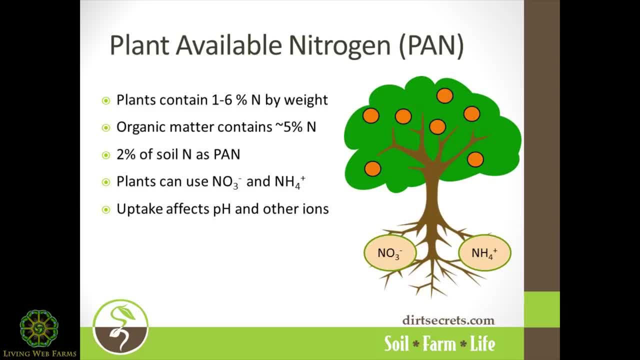 it's just an introduction. Plants can use nitrate and ammonium. they uptake nitrate and ammonium, which is what you get when this nitrogen is broken down by microbes and made plant available. So what we want to estimate is how much from the organic matter becomes plant available. 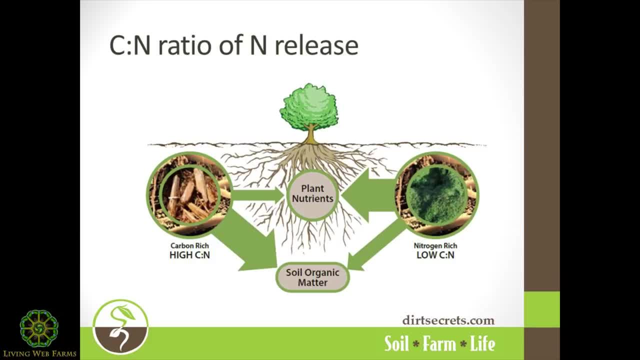 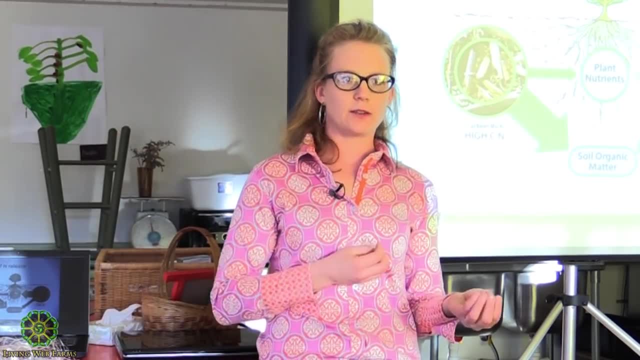 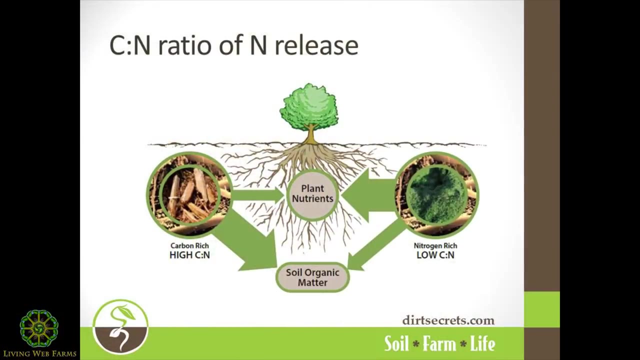 And most of you are familiar with the CDN ratio. So the CDN ratio is the ratio of carbon to nitrogen in organic materials. So we know that using organic amendments is important and we know that carbon is the food that drives our system. So the carbon to nitrogen ratio kind of determines. 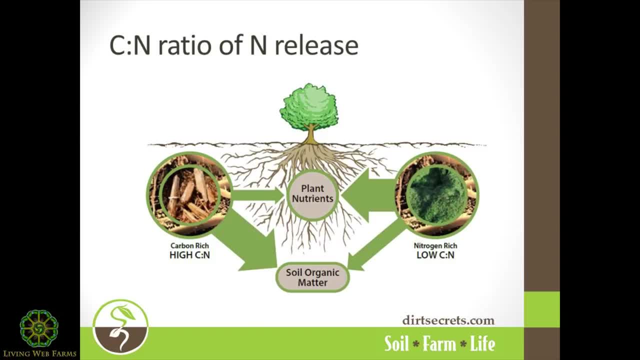 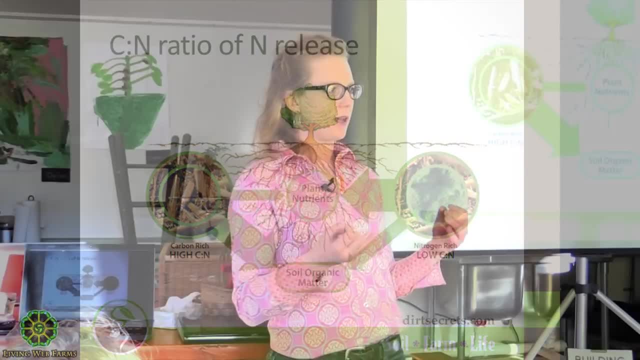 what's going to happen with that nitrogen when it goes into our system. So if that ratio is over 20, so if you think of a neutral material, we're talking compost leaves in general. This is just kind of textbook. We're talking compost leaves. about a carbon-nitrogen ratio: horse manure that's mixed with straw. the carbon-nitrogen ratio is about 20.. So when we add it, there's no net release in the moment that we add it or in the weeks shortly thereafter. There is net release down the line When we add a very high CDN ratio material like straw, which I think has a CDN of about 80, don't quote me, I don't have my tables in front of me- but a low quality, not very green material. 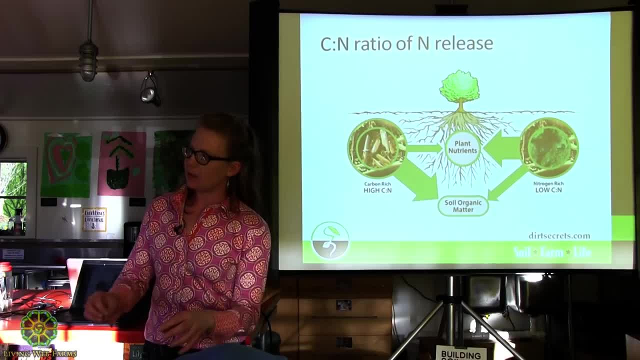 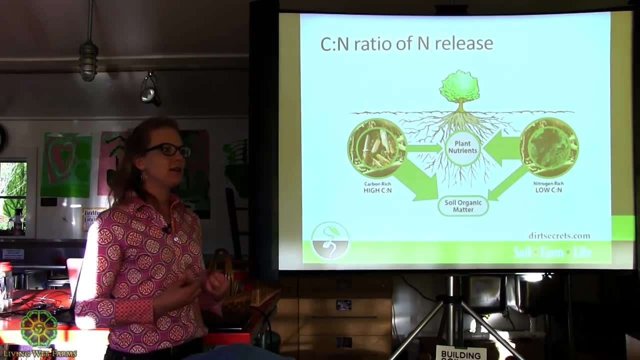 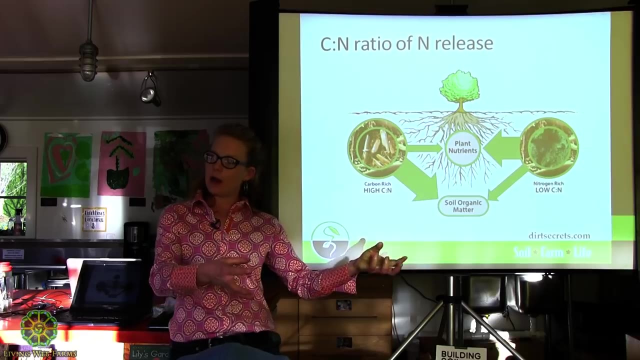 it's not going to have a net release of nitrogen. This is what people are concerned about when they talk about immobilization of nitrogen in that material. But if there is, it's an immobilization in time. Okay, So to decompose: 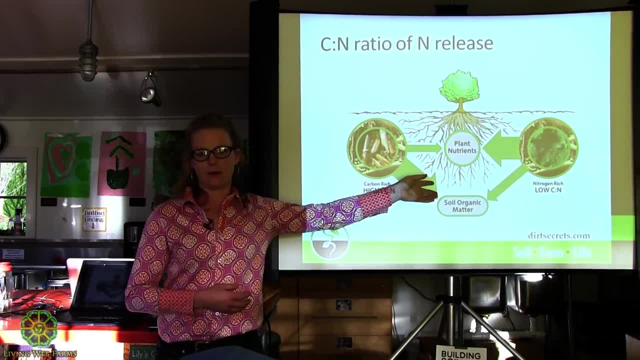 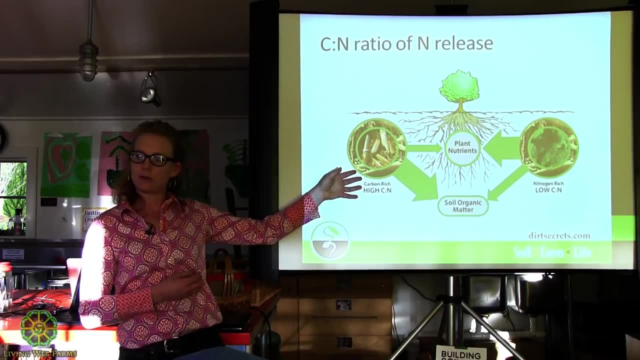 there's not going to be an addition of nitrogen to the system. there's going to be a retraction of nitrogen into those organic pools. But we want this sometimes because we want that nitrogen to be released later. So what is the time that we'd want our nitrogen? 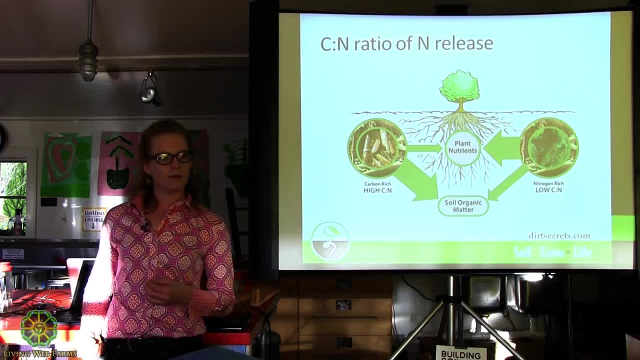 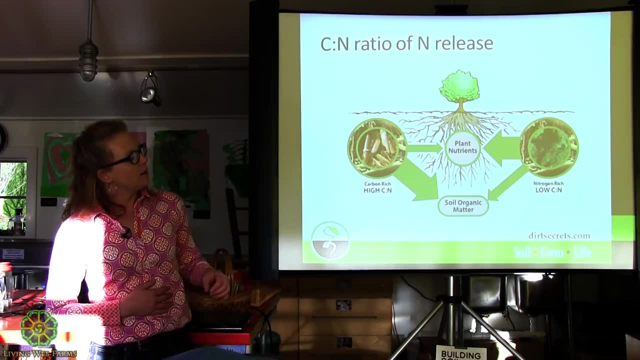 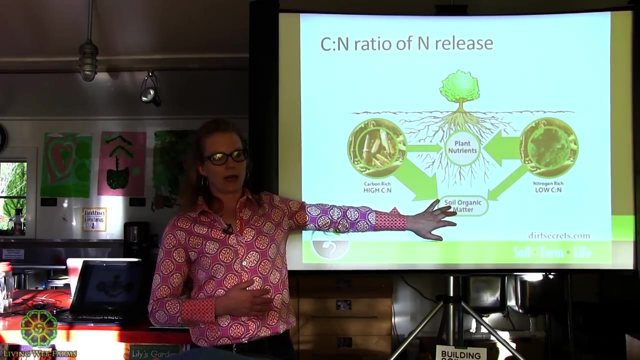 to be released or not available. Yeah, over the winter. So we want our nitrogen to go into these pools over the winter, for instance. But materials with a high CDN ratio, they go into this long-term organic matter pool. So when we add compost to the soil, for instance, 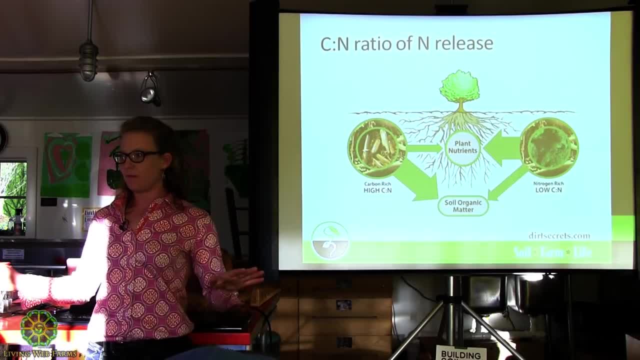 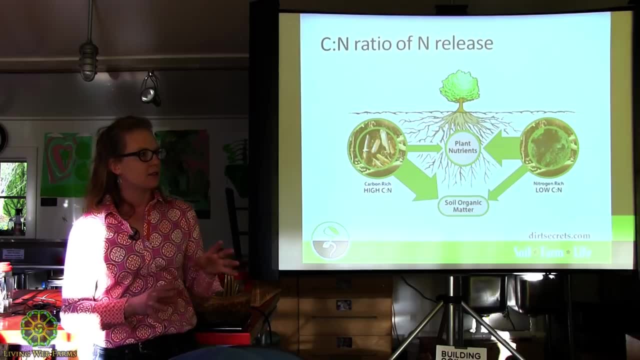 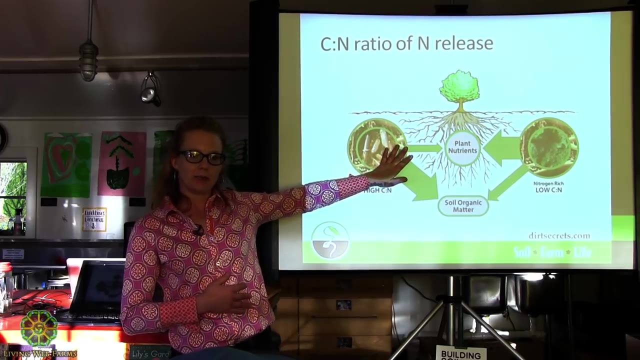 and I'm generalizing. there's a lot of variations because all organic amendments in all systems are very different in nutrient quality And, like we said, the way the biological system processes. it can be really different. But in general, when we add a higher CDN ratio, material 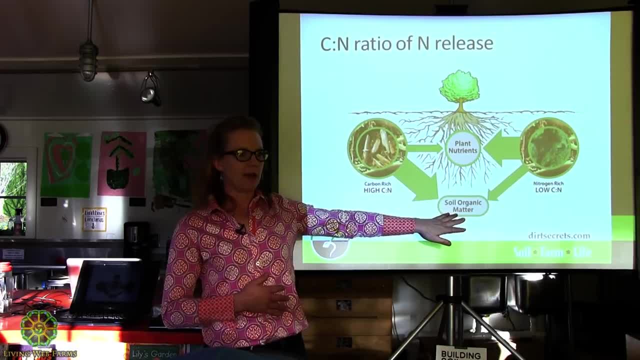 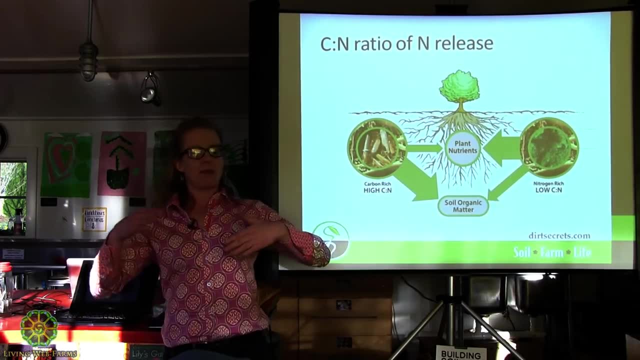 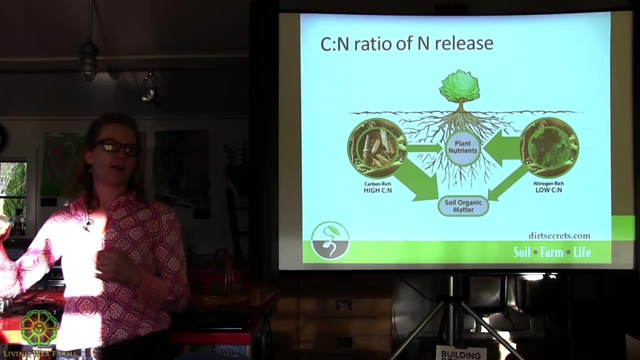 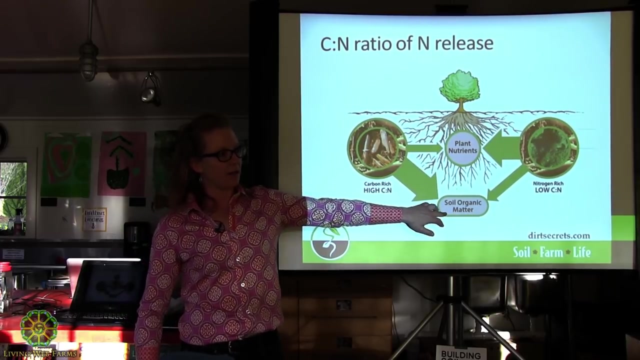 it goes into this soil organic matter savings account. So it goes into this long-term soil organic matter pool that maybe be available over the years, contribute to soil fertility in the long term. most importantly, contribute to important soil health functions of the soil that are driven by having this soil organic matter pool. 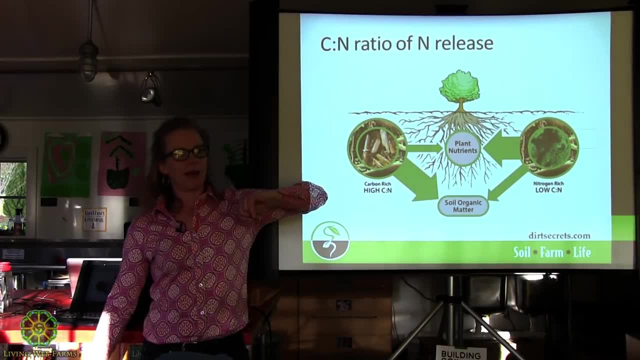 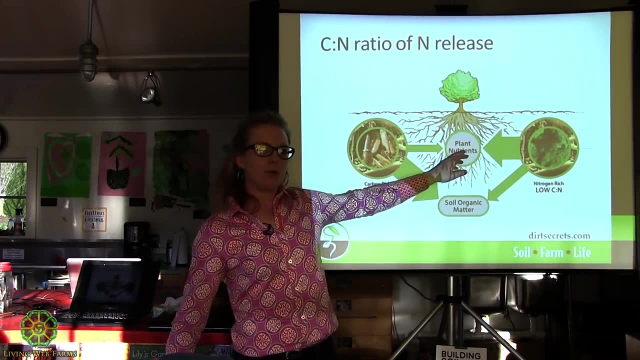 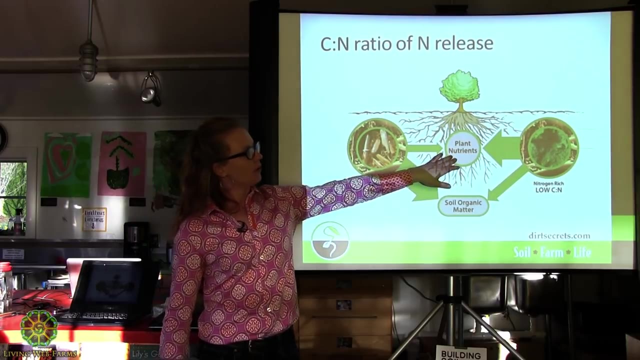 Whereas material with a very low carbon to nitrogen ratio, like grass clippings or fresh manure without straw or nitrogen fertilizer, go straight more into this soil solution pool. So it becomes plant-available nitrogen more quickly, which is great because that then drives plant growth. 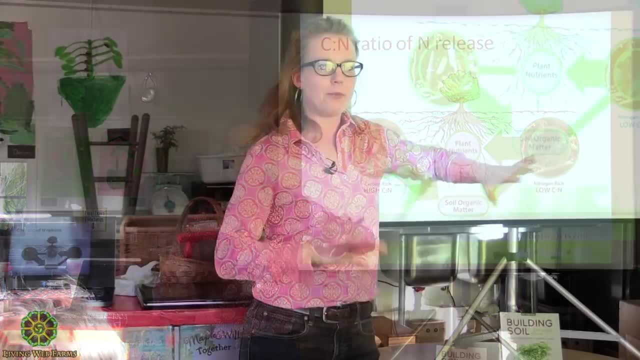 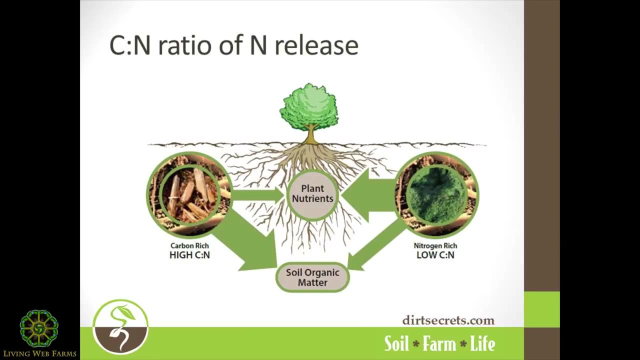 which then can drive our organic matter pool. So both are important. This is just a fundamental concept that I think a lot of people have questions about, so I think it's good to address it. So yeah, so it's highly variable. So if you want to have good benefits, your benchmark's: 15,, I've heard 20,, I've heard 12.. So above 20, we know it's going to be tying things up in the short term, So it depends on what else you're adding and what else is going on in your system. 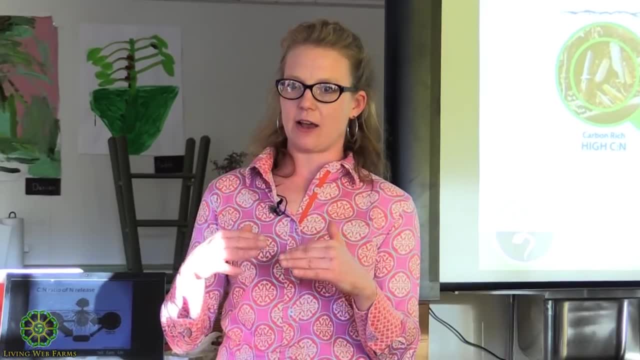 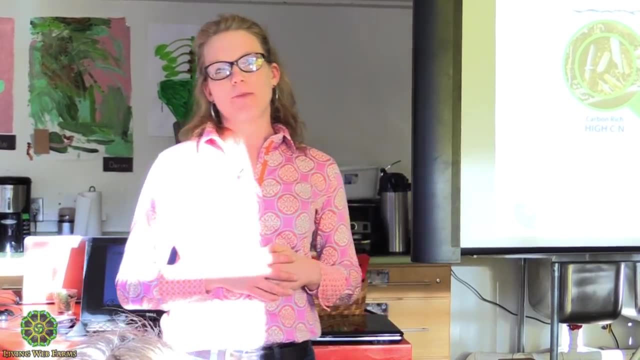 And to get that ratio, it really depends on how you compost it. And yeah, it's really Yeah, and you know it depends on your management style. So some people are using compost more just as an inoculant and looking, you know. 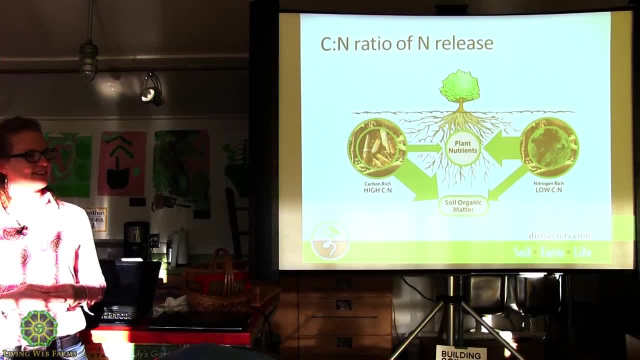 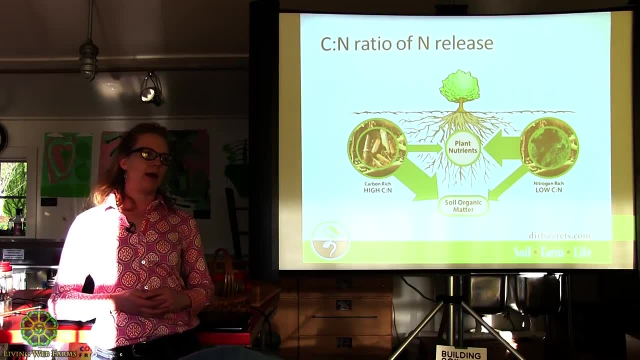 more to other sources of nitrogen. Is there an easy way to know what your ratio is? No, no, We'll talk about. well, I think we'll talk about amendment quality a little bit. But yeah, you can send your amendments off. 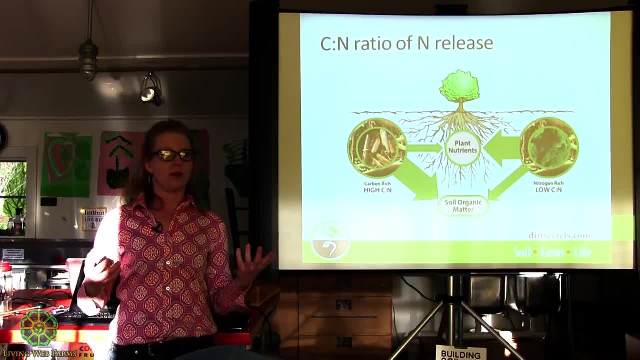 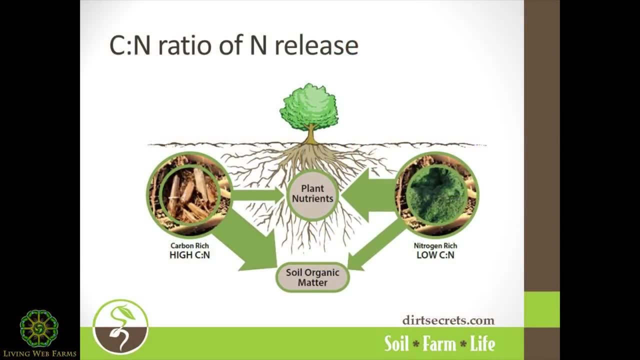 to get an idea of what your carbon-nitrogen ratio is. Or even you can look at it for C to N. That's a great benchmark. That's a quick benchmark. Your amendment test will also tell you the percent nitrogen percent. 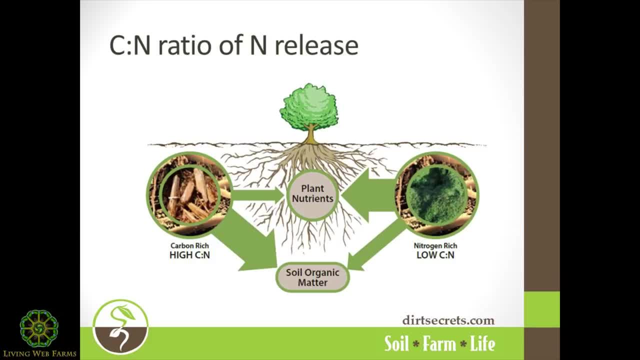 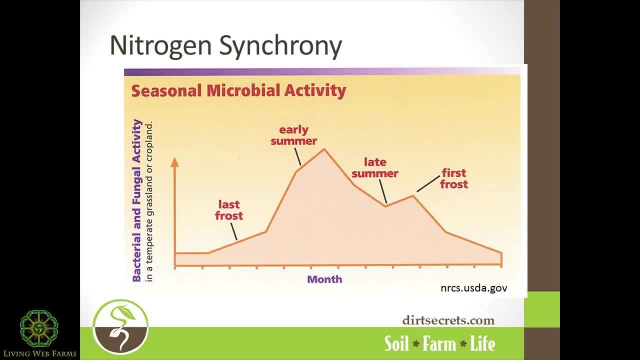 you know, just like your soil test would of different nutrients. Okay, so this is kind of what we're talking about. is this: matching your plant nutrients with your microbial activity, So your microbial activity increases? Oh, isn't that nice. You can use this in the northern. 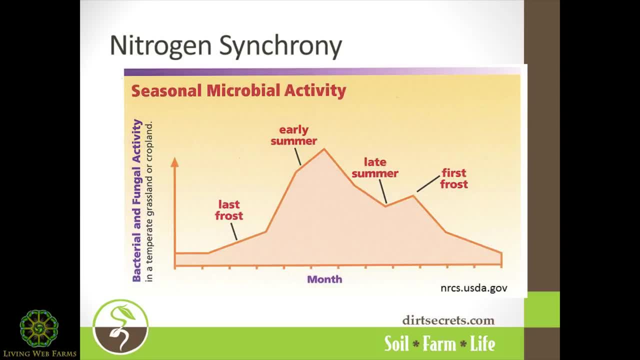 or the southern hemisphere. Okay, so your microbial activity increases with temperature And this is what drives the release of nutrients from your organic material. So it depends. you know this is going to be early summer, so let's say June, right here? 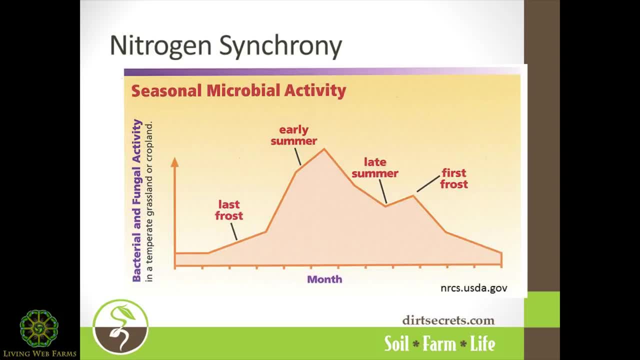 So you might have some spring crops whose maximum nitrogen need is here. You know you might have some late summer crops whose maximum nitrogen need is here. So this is just one of the things to consider is that your biological processes in your soil are driving this. 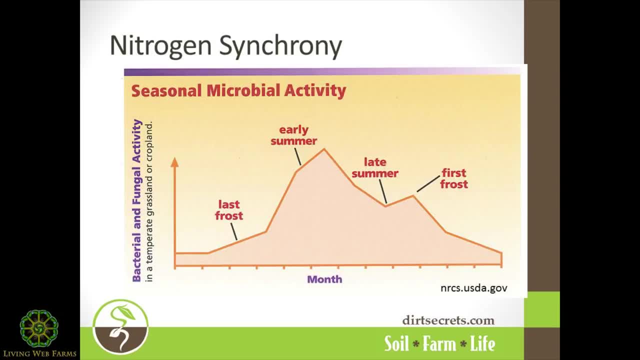 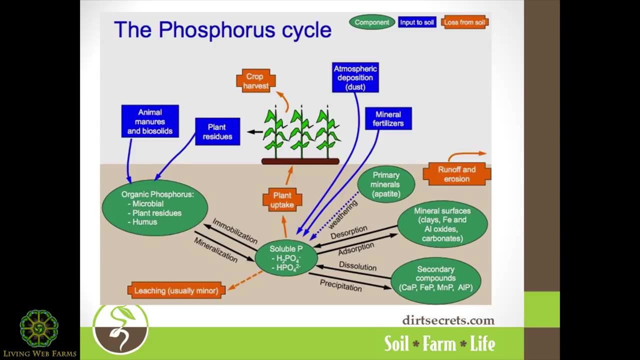 So you can't take measurements and match this, but you can focus on nutrient cycling so that there's always this kind of release and retention going on. This is our phosphorus cycle, So it's different in that we don't have as much leaching. 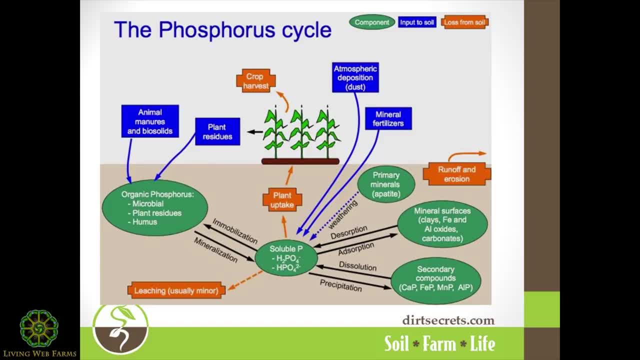 but we do. we can have a strong amount of soil absorption of phosphorus to inorganic parts of the soil, which means it's inaccessible to us. The benefit of working in this organic pool is we kind of start bypassing this by working with this organic system. 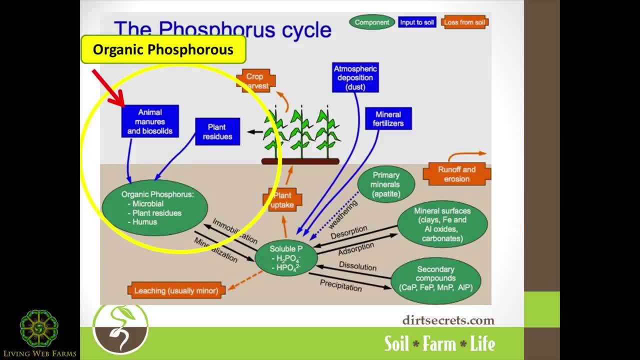 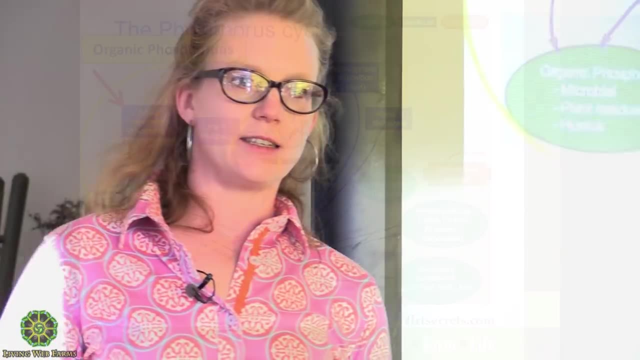 Okay, so we fill up all these sites with organic material and then we can use organic nutrient cycling to give plant available phosphorus to our plants. And this is phosphorus cycle- is largely, largely influenced by the action of mycorrhizae. 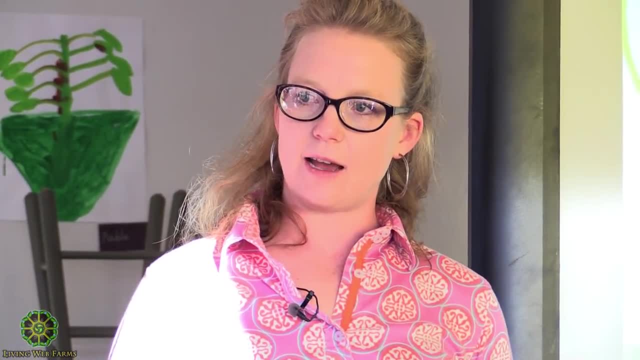 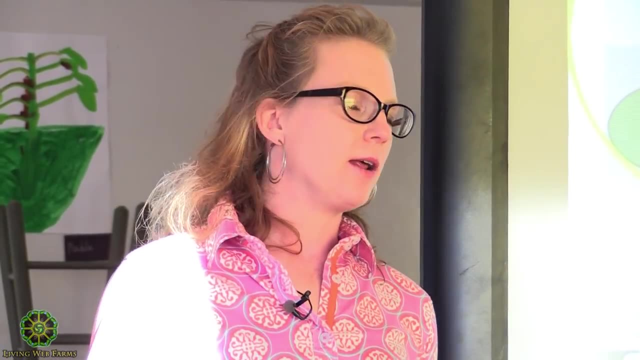 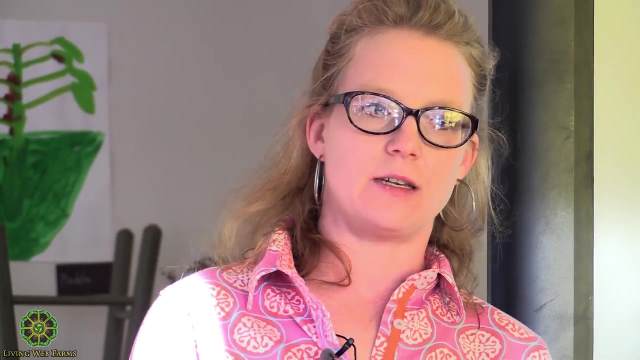 and their ability to mine phosphorus and other cations, And it's an important function, because not only does it bring more nutrients to the plant, but it also has a lot of other accessory functions, such as better water use efficiency, a more extensive hyphal network, 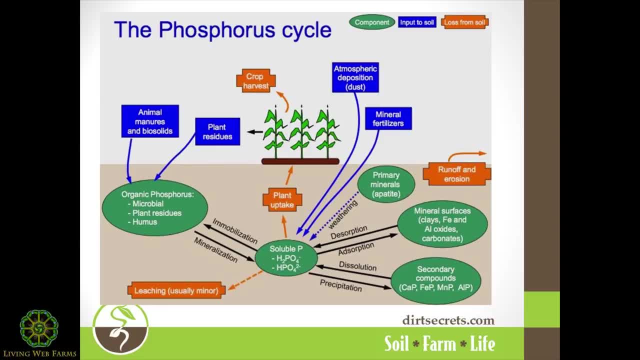 root network and a lot of soil health benefits that go along with being active in that soil biology. So if you have excess phosphorus in your system, you limit the activity of mycorrhizae Okay, so that's an important effect. 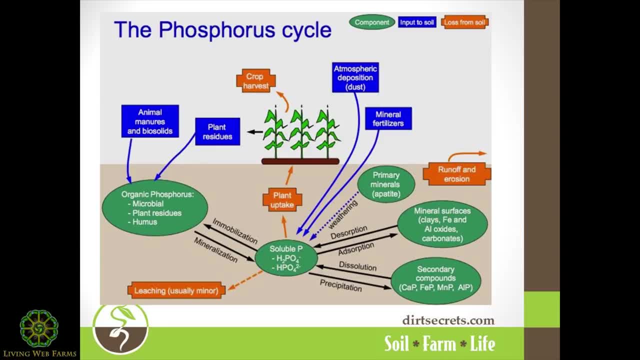 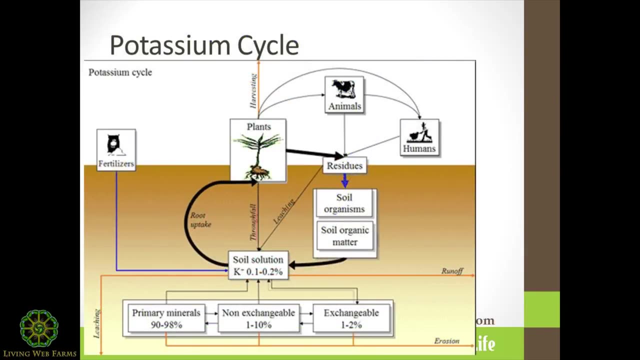 of having soils that have too much phosphorus, Okay, which can happen with a lot of our repeated manure applications. So when we're talking about driving the soil biological system, this is a big effect. Potassium cycle: what did I want to tell you about this? 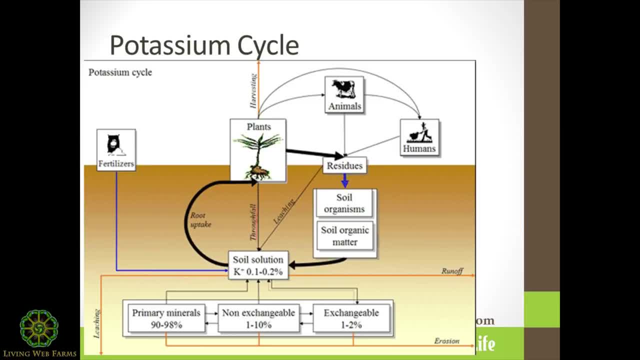 So we talked about? oh, one thing is that compost about? so only about 20% of nitrogen in compost. we're going to talk about that more. Let's see, So a smaller percentage of nitrogen is released from compost. a medium percentage of phosphorus. 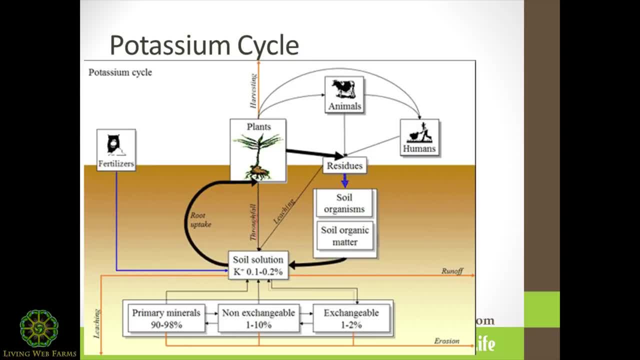 but potassium- about 85% of the potassium in compost- can be released pretty quickly, So compost is a great source of potassium. Do you find that Well? yeah, Sure, I mean. actually we have so many leaves, I worry that down the road. 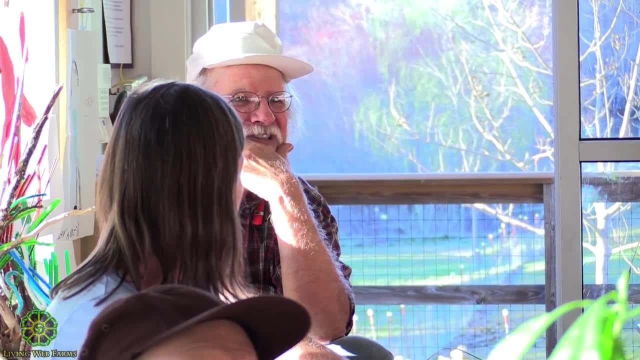 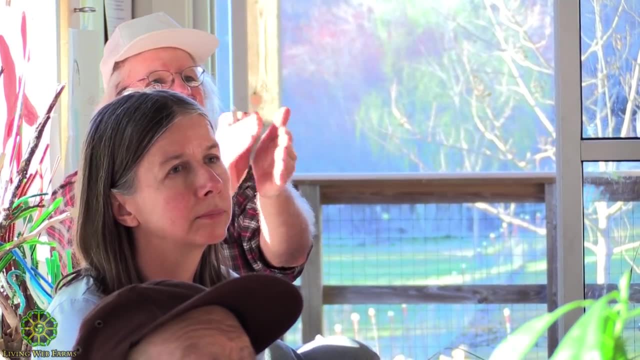 we're going to be backing up on potassium. Yeah, Yeah, I had a question for you about phosphorus. Yeah, On a soil test, where do you think the you know if you were mid range, low range, mid range? maximum range. sure maximum range is going to shut down mycorrhizae. where do you think it's? Yeah, So generally what I've read is that mycorrhizal function is maximized at moderate fertility and by having a large amount of soluble sugars. 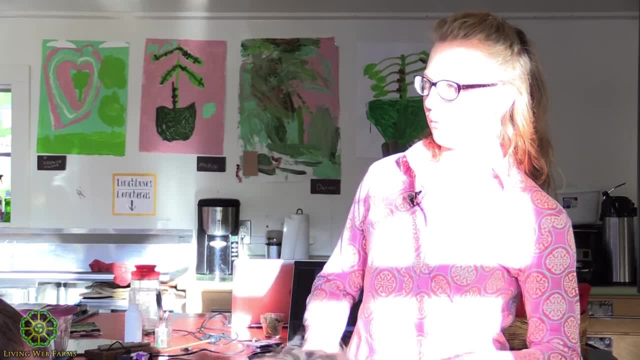 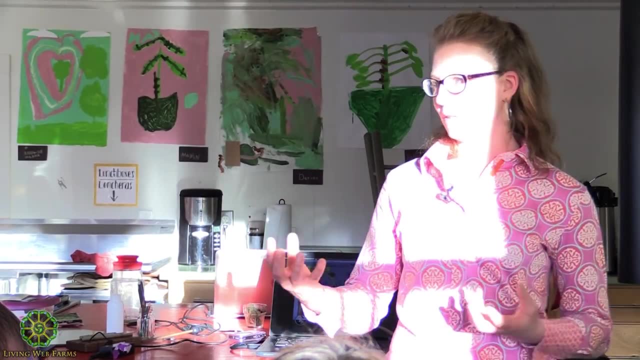 so like a lot of photosynthetic action and deposition through the roots. So I would you know. that's a good question And this is like when we were talking about it too. it's an area where more research needs to be done. So I would just take that moderate fertility as the M. Yeah, I think so. so what I tell people is when you're starting out like if you haven't had a soil building program and you're at the very low or the low end of the phosphorus, 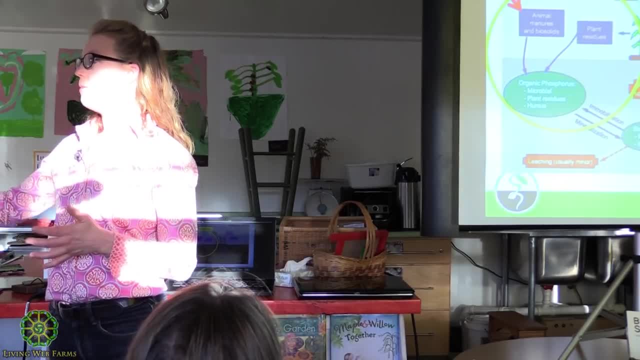 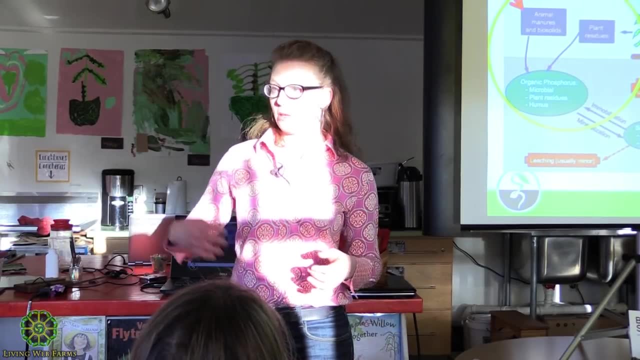 that's when you want to think about increasing your phosphorus supply. But if you've had a number of years of organic matter management and good yields, you're not seeing problems with yields and you're lower on phosphorus, then I think you can totally get away with it. Yeah, Because it's not measuring what's in that organic pool And a lot of phosphorus is retained, if you can do a good job retaining your residues And having cover crops. and yeah, Because not much is lost through the soil profile. Potassium. on the other hand, it can be lost to leaching, So you can get some accumulations deeper. If you do have excess potassium, you can have problems with salts. Not as much as an issue here, I don't think. in the humid regions, But at deeper soil levels you could have some buildup which can cause problems even at deeper levels. So just something to be aware of. You know we're talking about excess limitation. It's good to understand what happens. 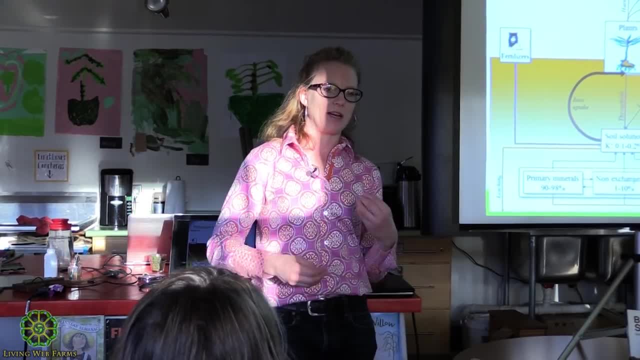 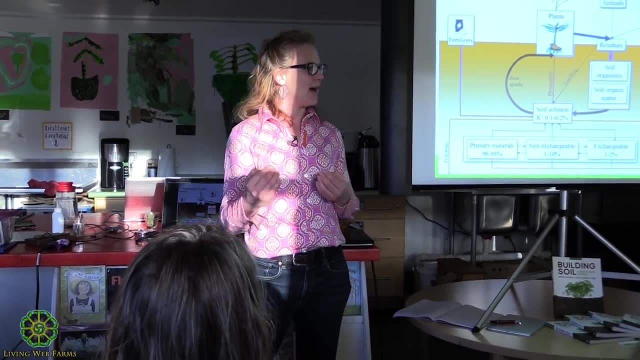 at either of these extremes And it's good to understand that any of your management practices- if you do the same thing over time, like you were talking about, you can kind of have an effect, Because nothing matches perfectly, Like your composts aren't going to match perfectly. 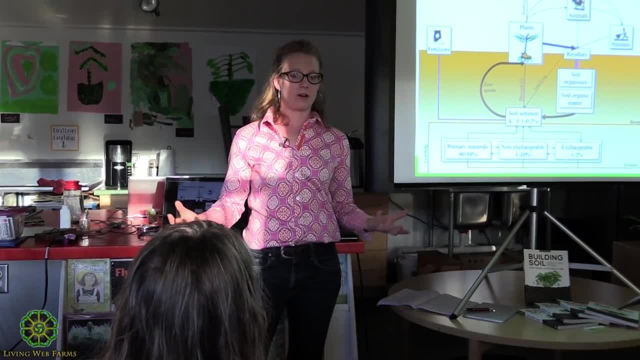 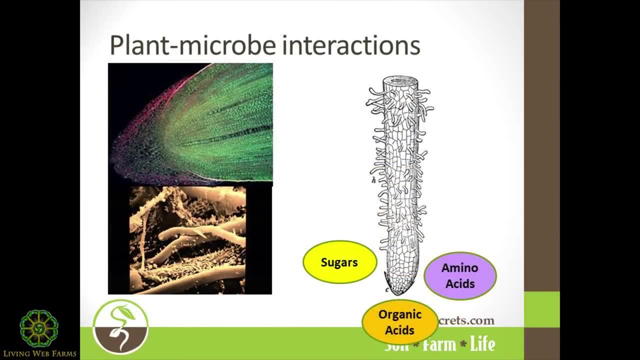 what your soil needs. Your manure's not going to match perfectly Cover crops. that's why cover crops are a great resource for nutrient management too. Like we were talking about, these plant-microbe interactions really drive what's happening here. 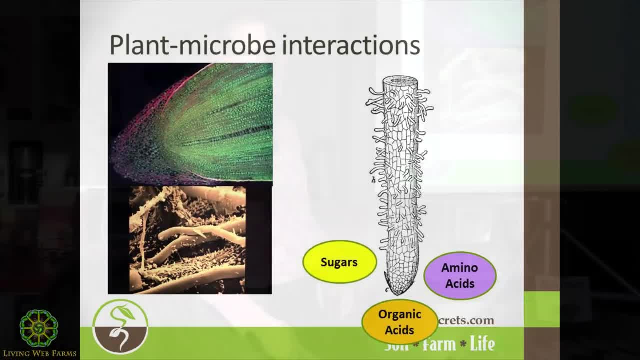 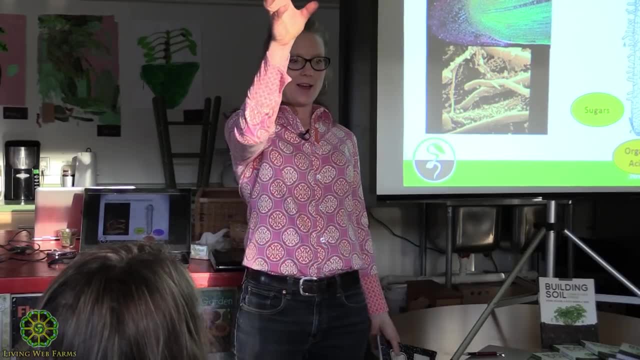 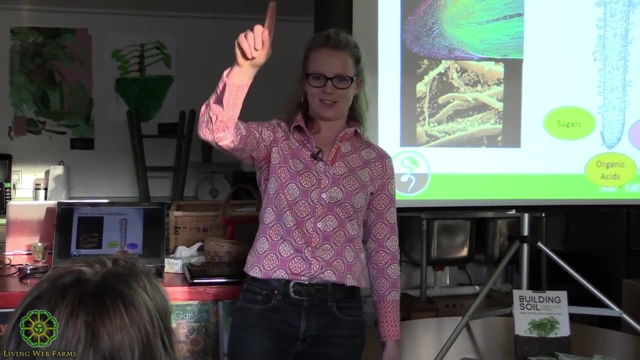 You have the rhizosphere, which is basically the hotspot for microbial activity. If you look at an electromicrograph, you see. or an infrared microscopy, you see this red hot zone of microbial activity just around the root. You go out a little further. 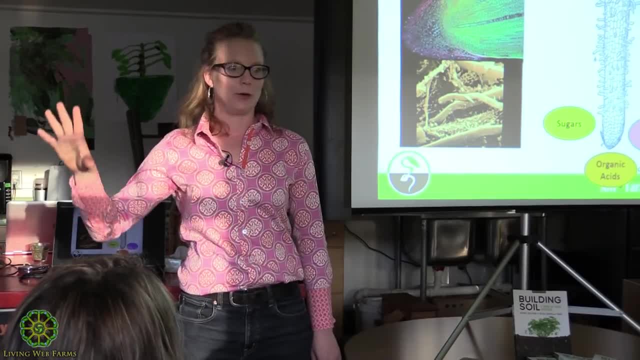 it's orange, You go out a little further. it's yellow, You go out a little further, it's blue. Nothing's happening, okay. So the roots are like the party, the microbial party- right, They're just exuding these sugars. 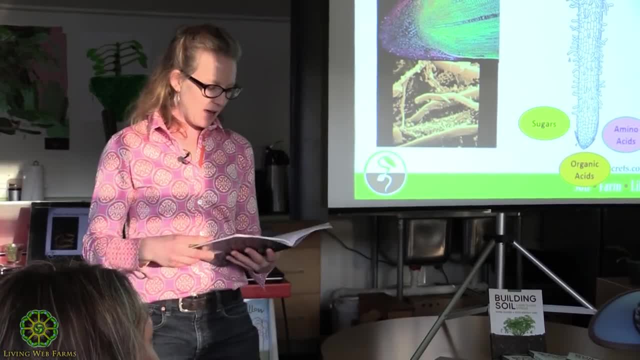 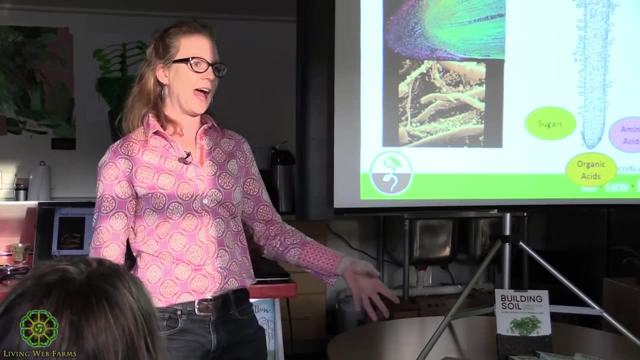 these amino acids, these organic acids, And they're really mediating a lot of soil-nutrient interactions, including how the plants take up nutrients, like we talked about mycorrhizae accessibility of nutrients. I'm just looking to see. 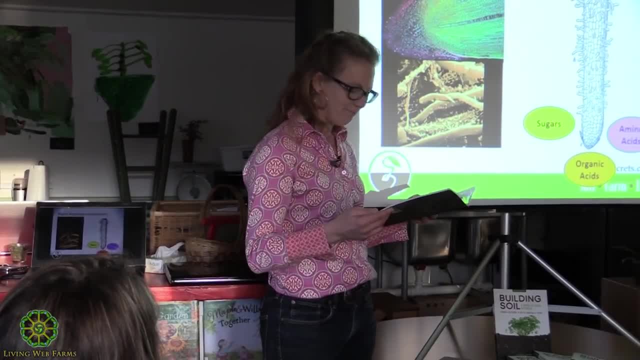 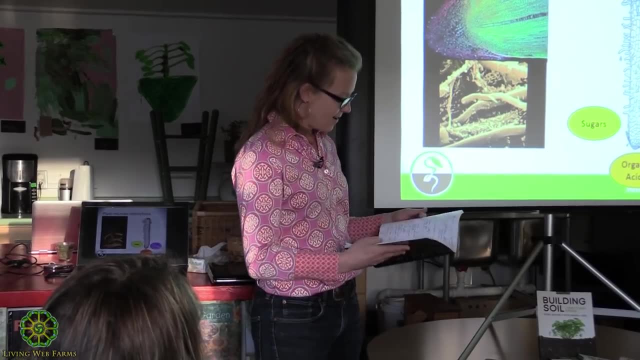 if there's something really cool here, There's something really cool. I wanted to tell you: No, not really. They affect like pests and disease. You know they can fight off pests and disease right on the roots there. So it's not an input-output process, right? 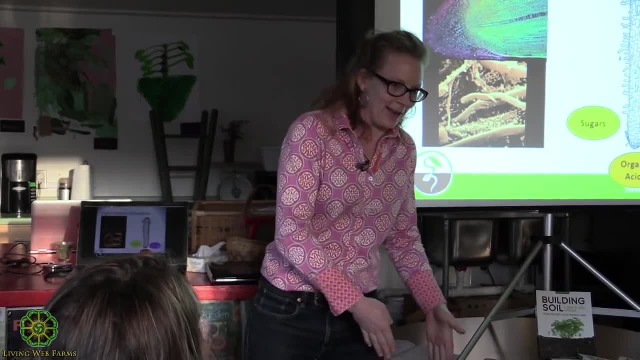 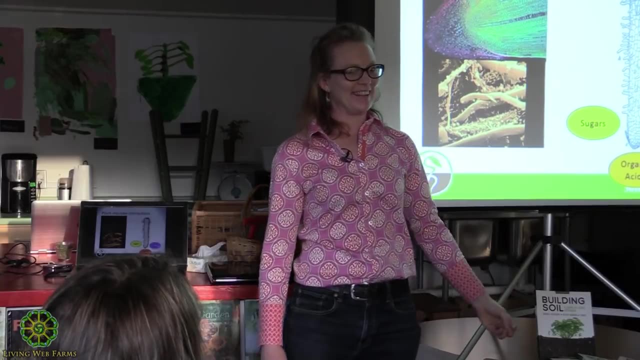 It's not. your plants take up nutrients, you put them back in. right. There's this crazy like wild ecosystem just on these root hairs, right? So this is why our biological systems are really important And it's why it is important to address. 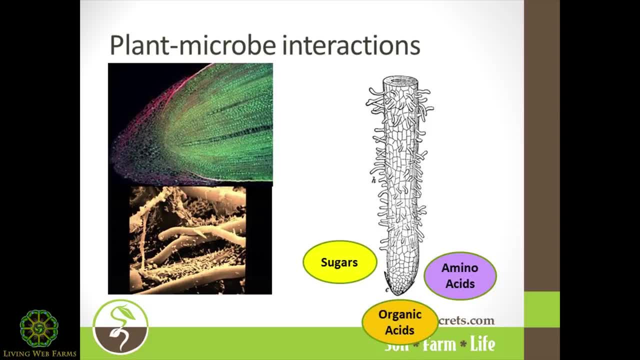 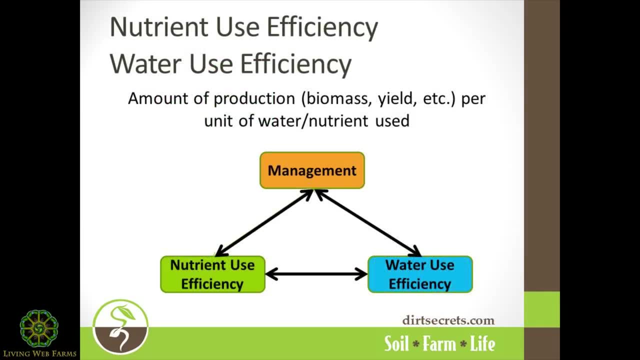 excess as well as deficiency, But our soil tests don't necessarily help us do that. Okay, so just a word about this nutrient use efficiency, water use efficiency thing so that I can see if I can explain it better than I did this weekend. 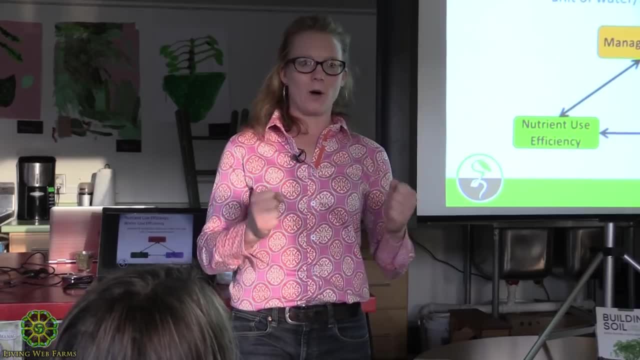 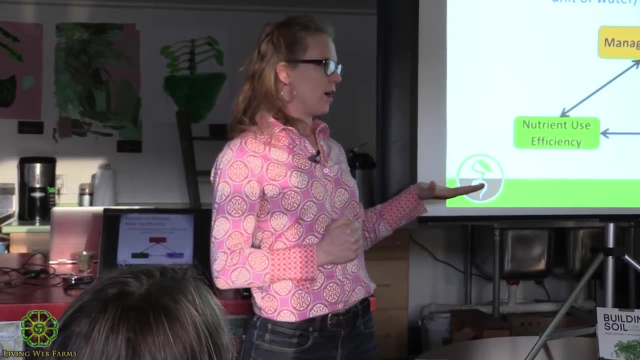 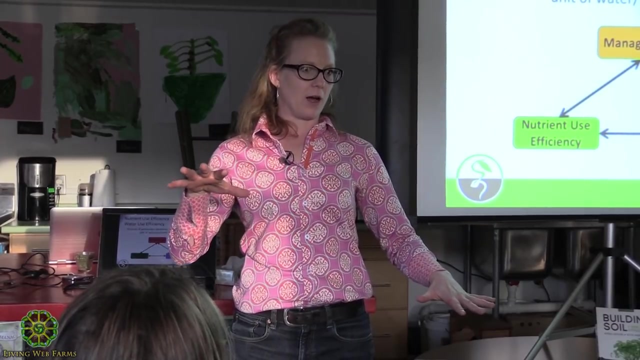 So nutrient use efficiency and water use efficiency are tightly, tightly coupled. okay, So it's not about the total amount of water you have or the total amount of nutrients. You can have two different systems that vary incredibly in the amount of water and nutrients. 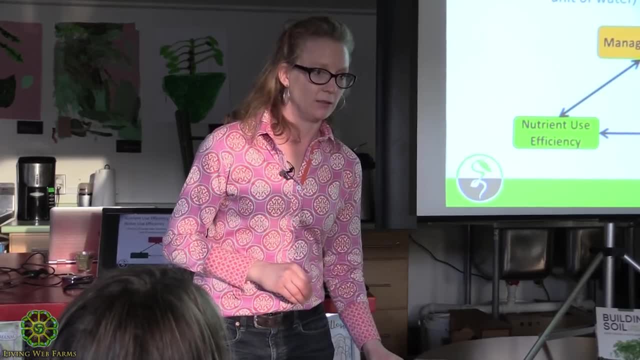 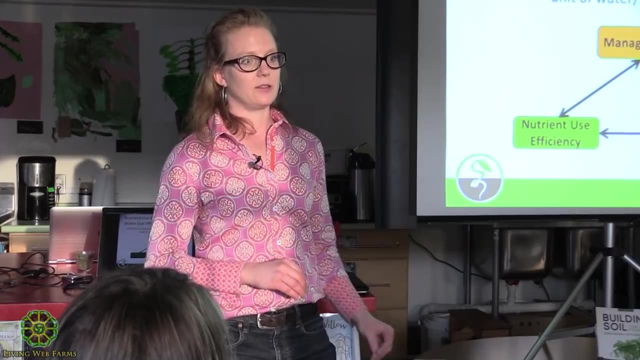 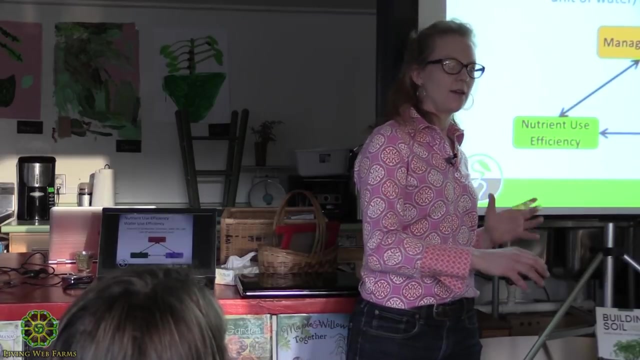 and you can have more production- dramatically more production- from a system with less total nutrient or water if it has better water and nutrient use efficiency, okay. So relying on ecosystem processes increases both nutrient and water use efficiency, which has this synergistic positive feedback effect on each other. 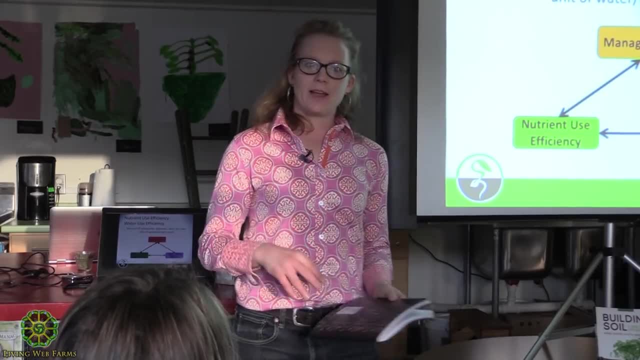 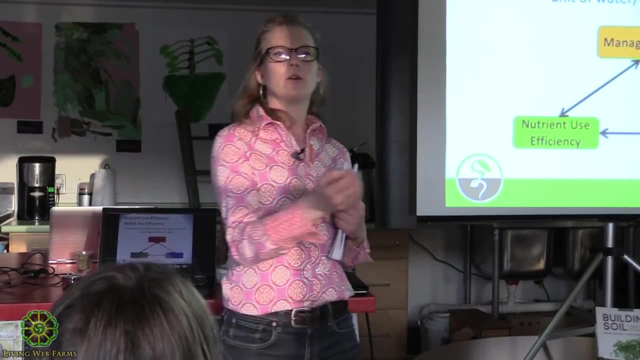 So in the Great Plains there's something called the drought myth. okay, Sometimes we think it's an effect of water, that we're getting low yields, when really it's an effect of fertilizer, okay, And you can get the same yields at a fifth of the water. Actually you get four times the. in one study you got four times the yields at a fifth of the water in a system that wasn't nutrient limited okay. So there's a big effect on how much water you have to use, how much irrigation you have to use. how much water you can get away with producing bigger yields if you have more efficient use of nutrients. Does that make sense? And that all depends on your management and how much you're relying on nutrient cycling. okay, So it's not just about the total. 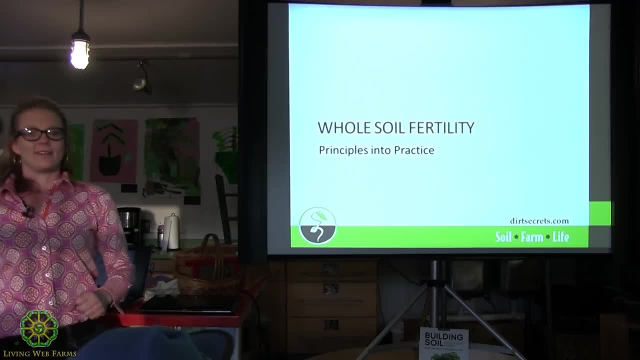 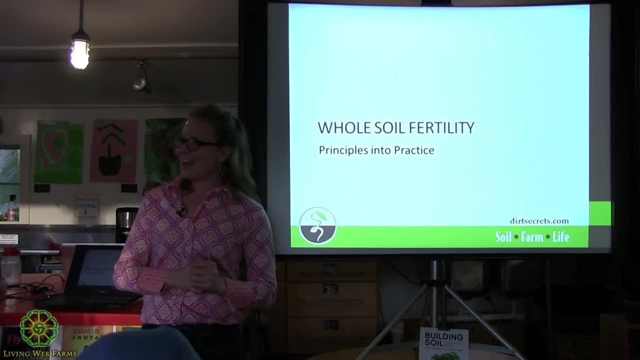 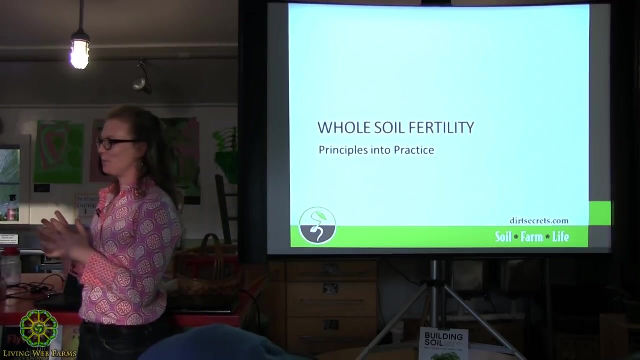 it's about the efficiency of use. Okay, So that was a brief background. I'll get to the fun part. Yeah, fun for you. I don't know, Does anyone have any questions? Yeah, When you want to alter your CN ratio. 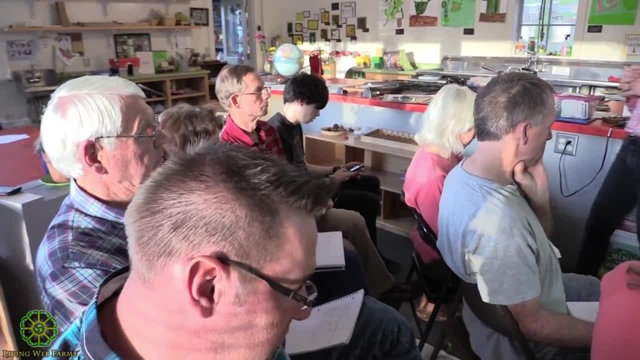 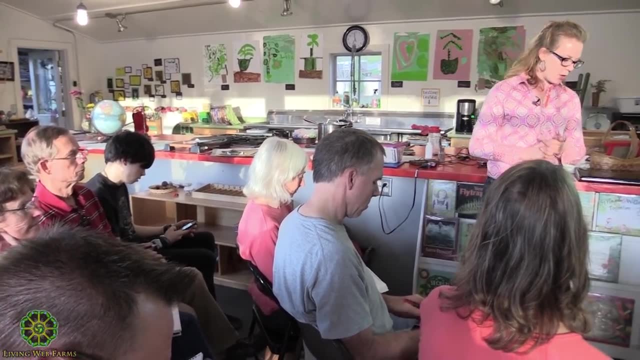 what tools do we have to do that To alter the CN ratio of your organic amendments or your soils Of the amendments Of your amendments? Okay, so it's Like compost or whatever. Yeah, it's important to add organic material. 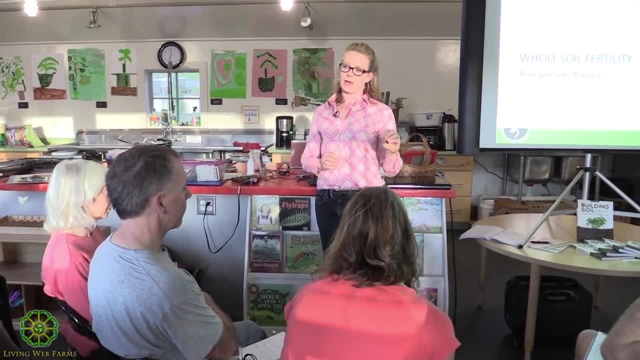 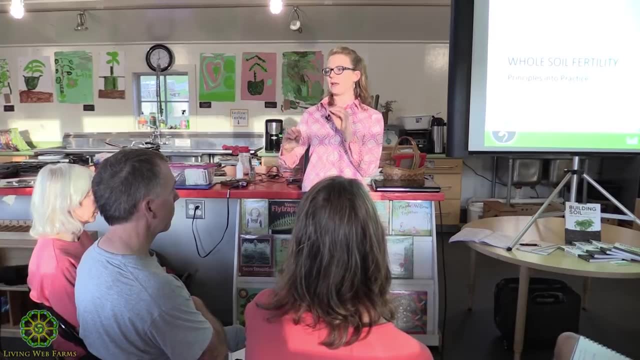 And a lot of the organic materials we have might have a CN ratio that's higher than optimum, And in those cases we want to make sure we're adding a lot of materials that have a lower CN ratio. Okay so, And it also depends on the time of year. So I'm okay with adding like mature plant material in the fall as residues, because I don't really want a net nitrogen release. but it will feed, You know. they will decompose slowly over the winter and there's usually a mixture of nitrogen. 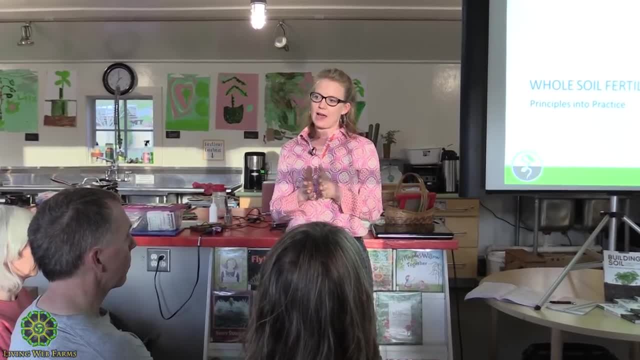 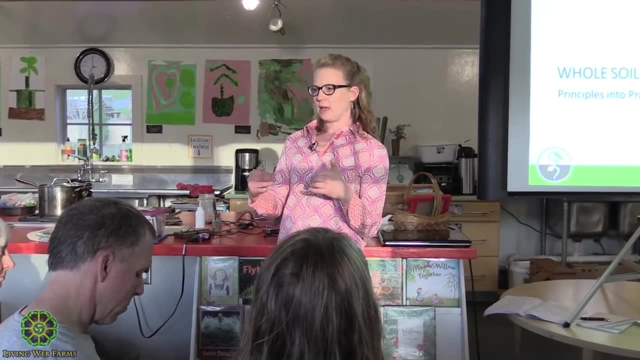 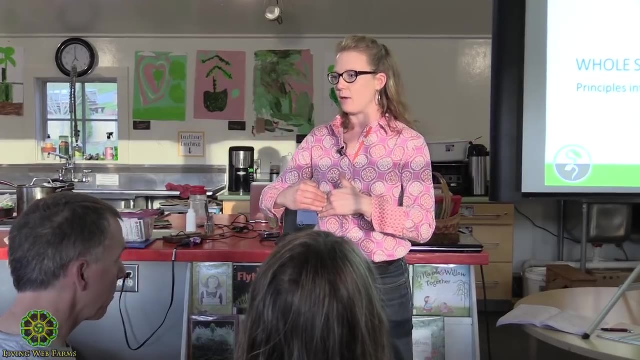 In the spring, in the early spring, I can add some higher input materials with lower input materials. This is used more like in chemical systems. now They're using a more integrated management system where you're adding really low quality residues with really high input chemical fertilizers. 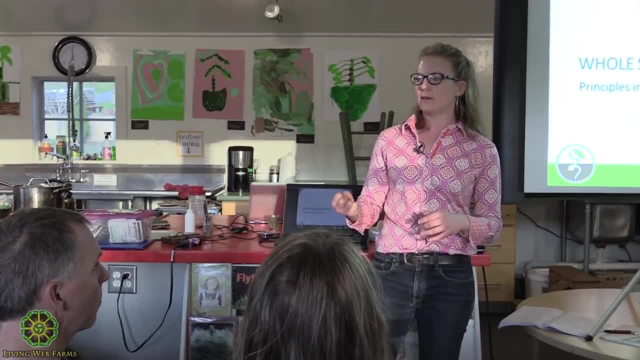 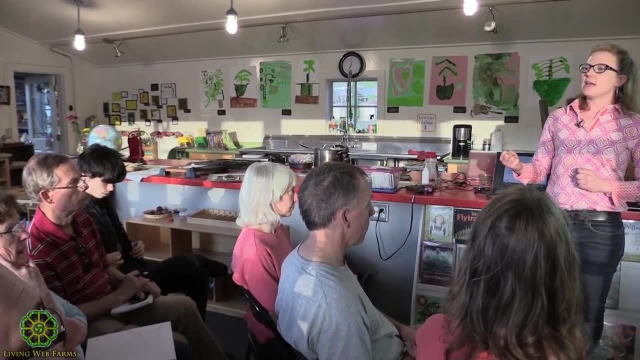 And it's a way for the systems to hold onto those fertilizers. Can you use simple things like watering or No? no, it's Yeah, and you don't really want to necessarily. I mean, it's not that you don't want to have. high C to N ratio materials. It's that you want to make sure there's enough of the other stuff accessible to microbes And it really depends on your system. So low C to N materials or anything that's in the early young. green stages of life. grass clippings, cover crops before they get very mature. Okay, so that's why we kill cover crops before they get super mature. That's why we try to graze our grasses earlier. Well, we don't graze them. 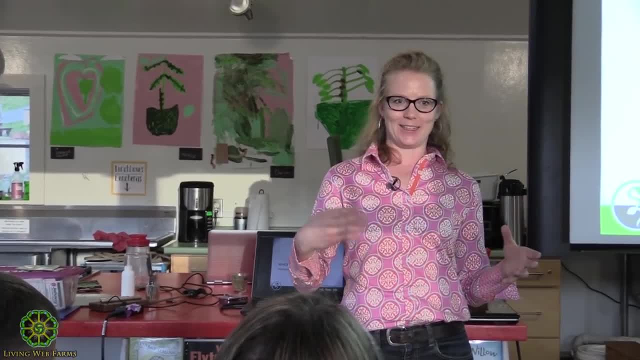 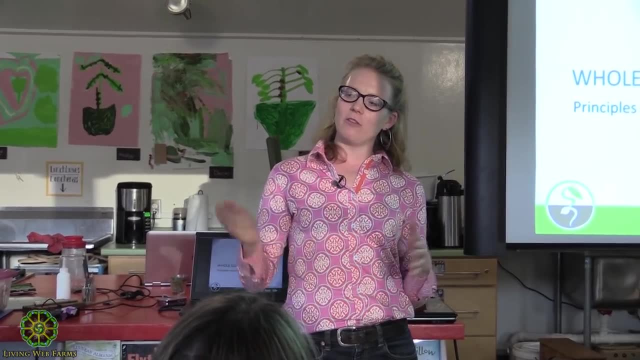 but our animals graze them right, Because there's more protein for them. I don't know if I'm really answering your question, but maybe, Yeah, you don't really want to try to change the quality of your materials. I mean, sometimes people do fortify amendments. with fertilizers, But it's something. But if you are going to add a low quality material, make sure you do add some. If you want to be growing plants a few weeks after, make sure you add some high quality nitrogen. Yeah, but it's also about timing somewhat. 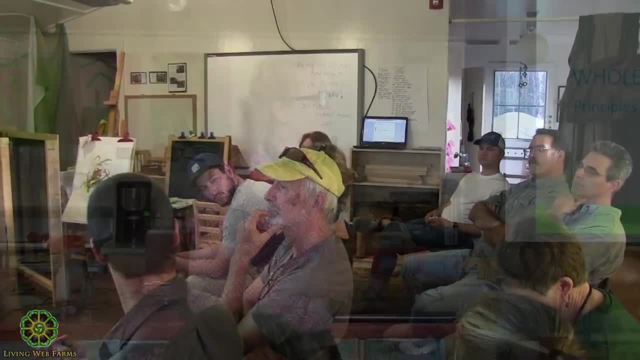 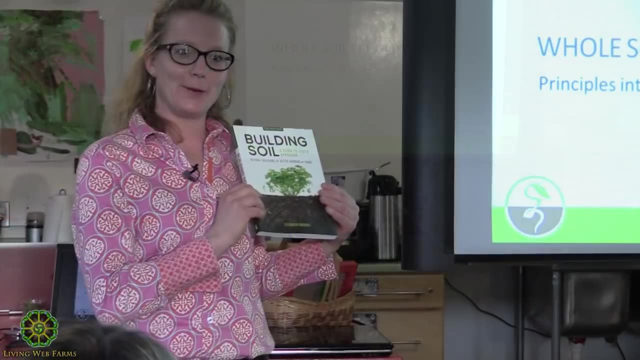 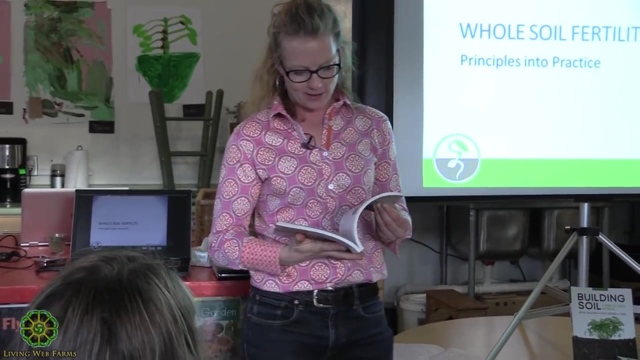 Yeah, Do you see a ratio of worm castings in general? Five or eight. Let me look at my book Building Soil, which will be on sale after class. Five or eight. Anybody know off the top of their head worm castings? 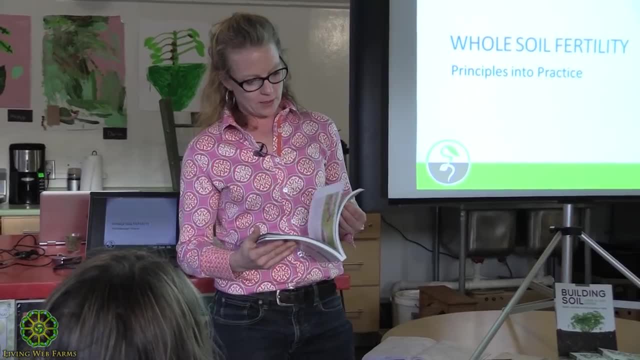 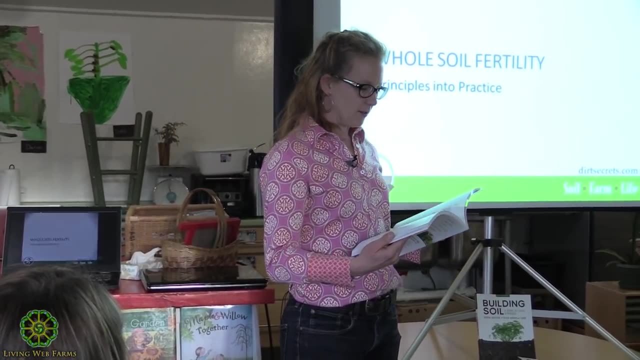 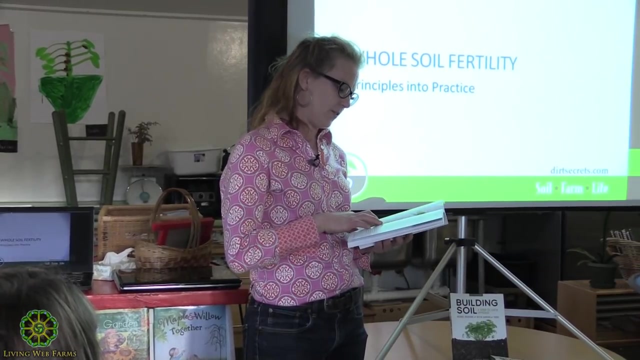 I think it might be eight. It's pretty darn low. Yeah, that's why worm castings are like basically little pellets, power pack pellets. I mean they're concentrating nutrients, Worm castings- Oh well, this says 12 to 15.. 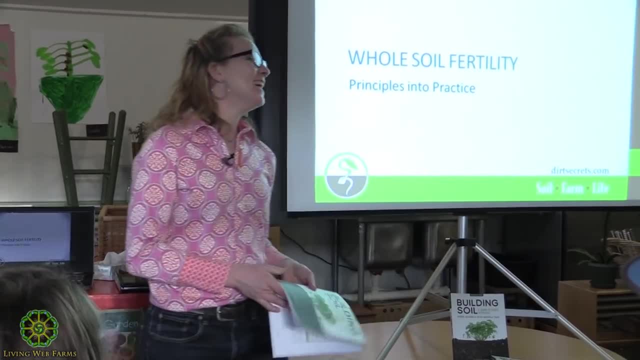 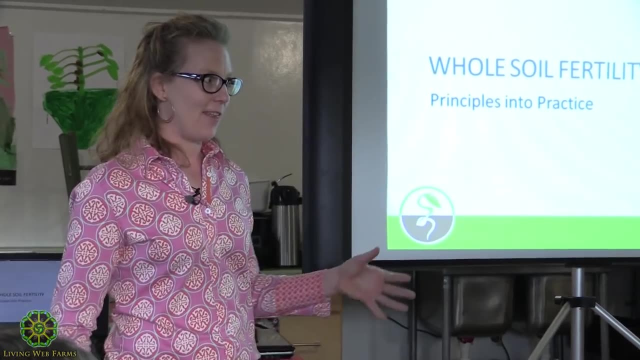 This book says 12 to 15.. I think it's lower. No, it's really variable. So it's incredibly variable. okay, And we're going to get to What we do with all that variability which, in my opinion, 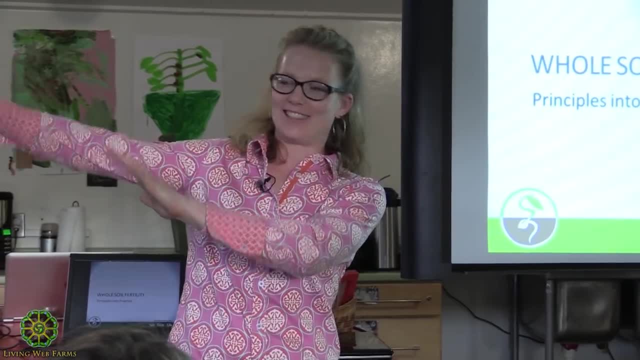 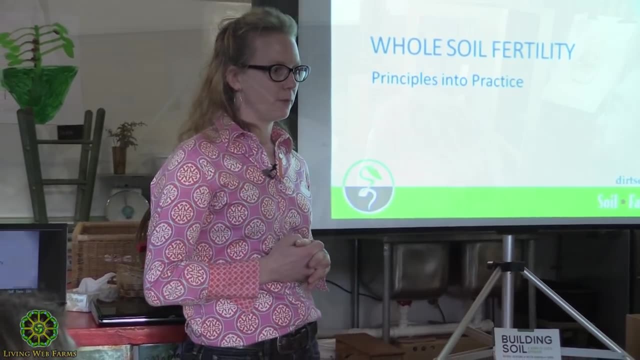 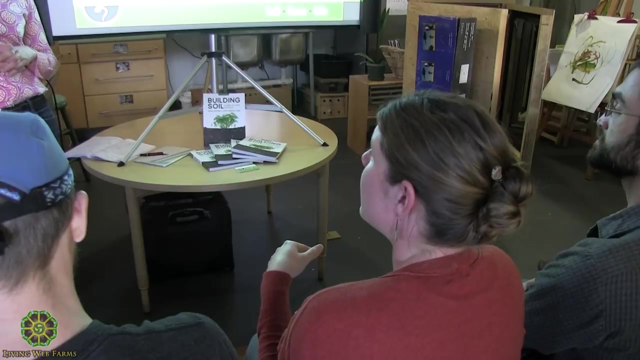 is you kind of toss it out the window and make your best guess and look at your plants? Yeah, I just wanted to clarify something that you had said earlier about. You said: maximize the living plants and minimize chemicals and salts. Can you give examples of sources of salt? that you would want to minimize. Okay, sources of salt. Any fertilizer is a salt, whether it's organic, inorganic. A salt is a chemical term referring to these cations and anions, Mostly cations that we're talking about. 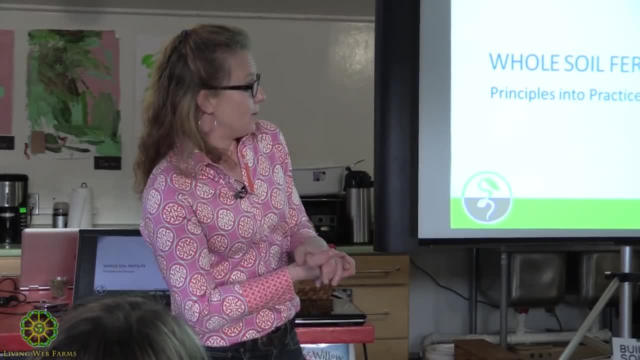 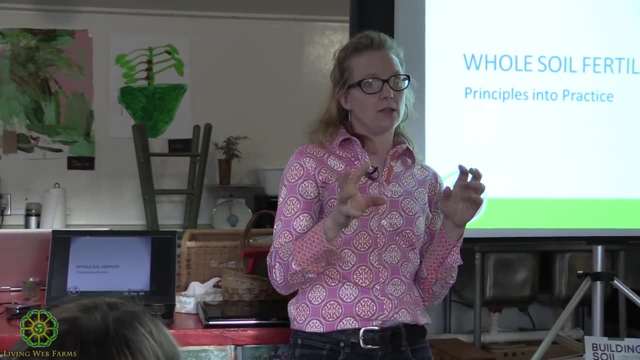 or anions too. Yeah, so that's a salt. So high salt materials or any fertilizer is a salt. And then materials that have a lot of salts are materials that have gone through a lot of wetting and drying, So those can get concentrated in salts. 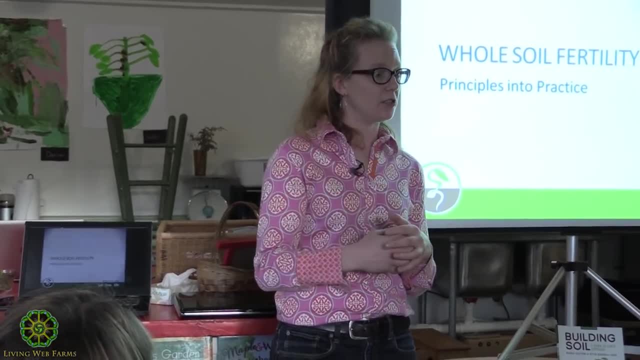 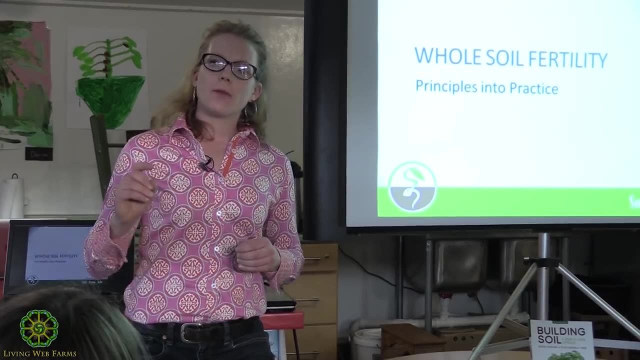 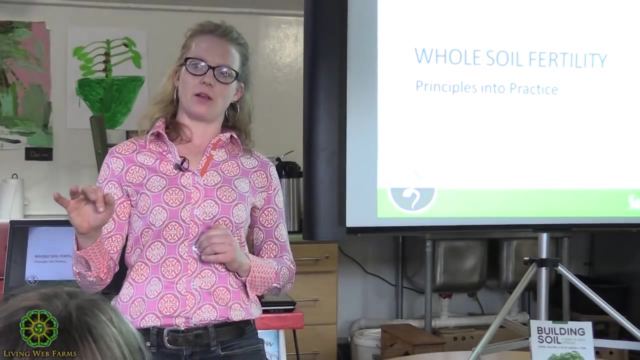 Manures are generally concentrated in salts. I mean because they're really concentrated fertilizer sources. So those are examples. What about leaves? I have heard of that a little bit with the potassium, but not so much. It depends on how much rainfall you get. and your soil type as to whether You know if the soil's not draining. that's when you can have some salt buildup too, depending. So mostly we see salt problems in areas that have been mismanaged by fertilization and areas with poor quality irrigation. water can also be a source. You can have poor quality irrigation water. You can also have irrigation water that has a lot of nitrogen in it, So you can be over-fertilizing with nitrogen just from your irrigation. So it's good to have that checked out.